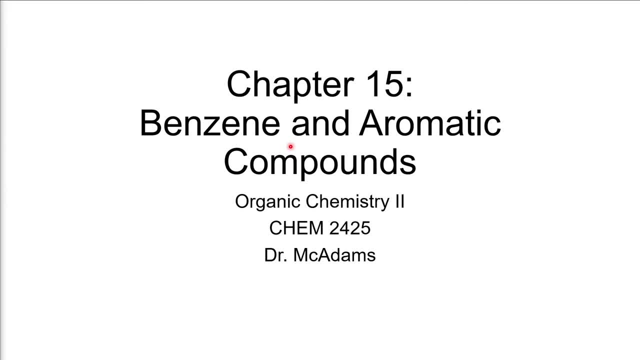 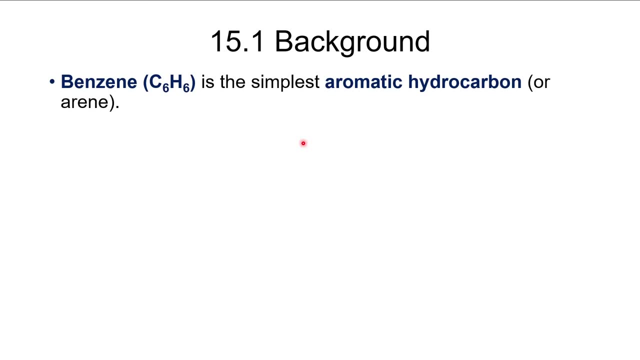 and other aromatic compounds like benzene. So we want to look more closely at benzene and these other aromatic compounds. Let's get started. So we're going to start by looking at the simplest aromatic hydrocarbon, and that is benzene. Benzene has six carbons and six 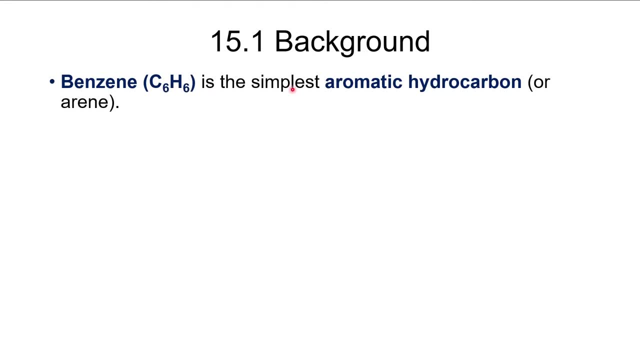 hydrogens, So one hydrogen on each of the six carbons has a planar structure. All the angles come out to 100%. All the angles come out to 100%. All the angles come out to 100% And we typically represent it as a hexagon with three double bonds, three alternating double 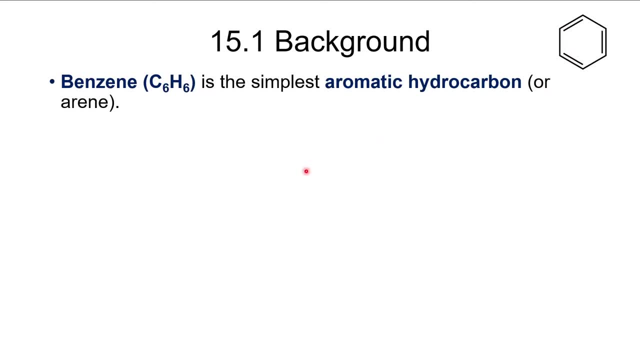 bonds And that is our best structure of benzene that we can draw. Because of the three double bonds in the ring, we'll find that benzene has four degrees of unsaturation. Now we're going to do a little bit. later we're going to do some calculations of degree of unsaturation. If you 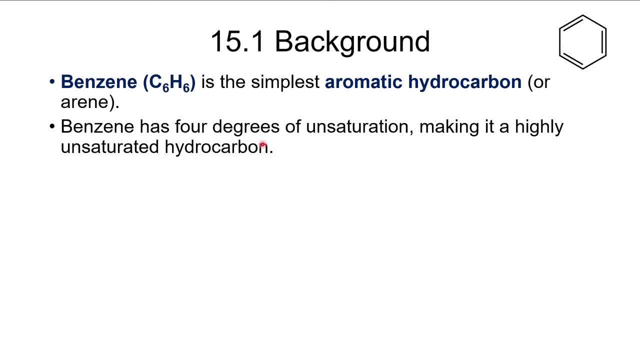 don't remember it, go back and look at chapter 10.. And at the beginning of chapter 10, we're going to I show how to calculate degrees of unsaturation. Now compounds, other unsaturated compounds like alkenes, alkynes, polyenes, all right, they will all undergo electrophilic addition reactions, like 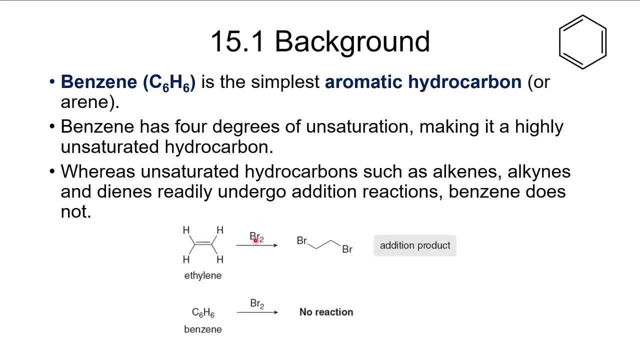 this. So, for example, ethylene, if we react that with bromine Br2, we will get 1,2-dibromoethane. If we take benzene, we'll get 1,2-dibromoethane. If we take benzene, we'll get 1,2-dibromoethane. 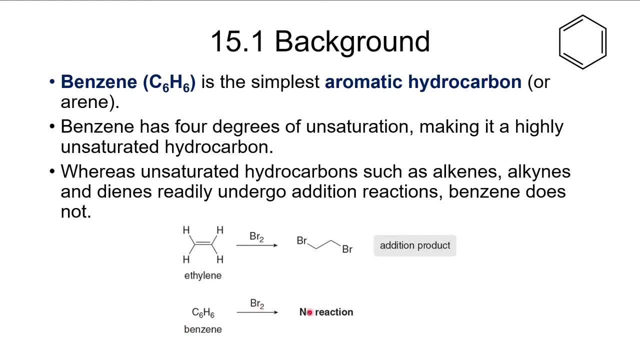 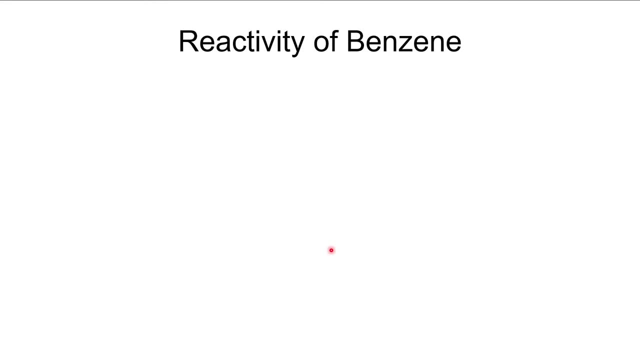 And put bromine in with it, we get no reaction. Well, if we put bromine by itself, we get no reaction. We definitely don't get electrophilic addition. So we will find that it is possible to react benzene with bromine, but only if we have a special catalyst called FeBr3 or iron-3. 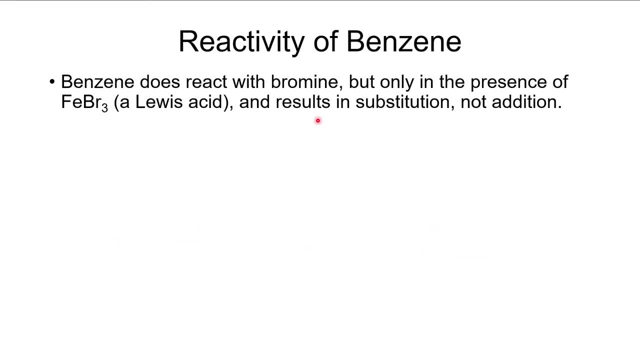 bromide. So what we're going to do here is we're going to take this Lewis acid and instead of giving us an addition product, it gives us a substitution. As you can see here, we've replaced one of the hydrogens on benzene with a bromine, So that is a substitution. In the next chapter we're going to 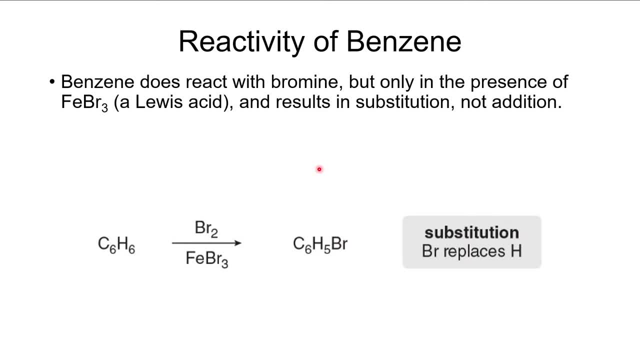 talk about the details of this reaction, which is called an electrophilic aromatic substitution reaction. We'll get into all the details in chapter 16.. But for now we will say that benzene does not undergo normal electrophilic addition, and that is where we add an electrophile. 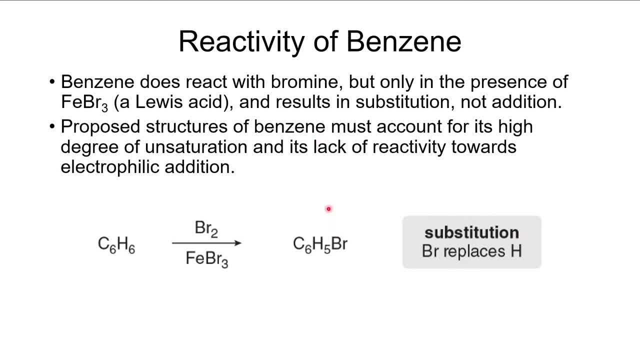 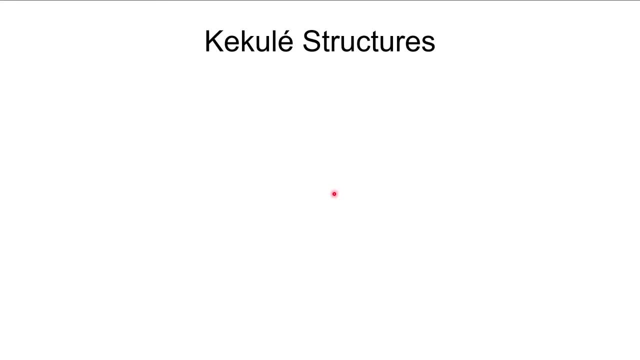 across a carbon-carbon double bond. We just don't get that to happen. So we want to look at the structure of benzene. We want to understand why benzene has the particular structure that it has and why we represent it in the way that we do. 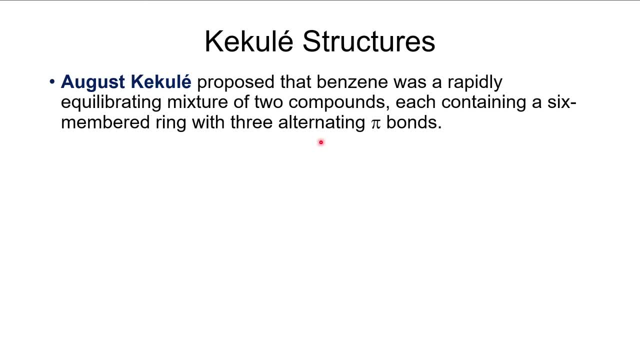 It all goes back to a chemist named Auguste Kekulé, who proposed that benzene was actually two compounds that were identical, but they equilibrated back and forth, where each one contained three carbon-carbon double bonds and three carbon-carbon single bonds, So we have the 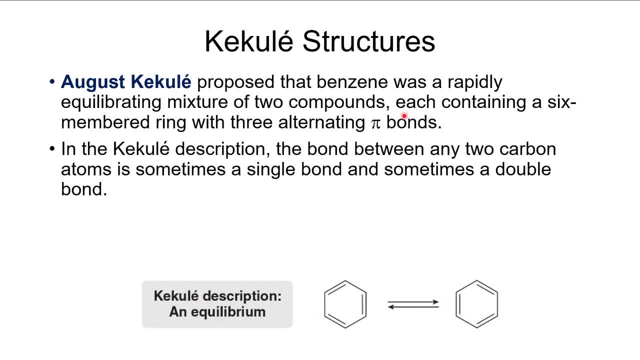 alternating pi bonds. In this description he says the alternating pi is an integral of a two-carbon-carbon double bond, So it's going to be a single bond and the negative is going to be a double bond. So the idea is that benzene went back and forth, back and forth between these. 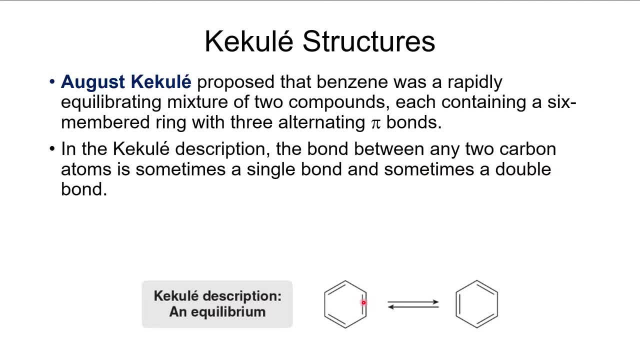 This looks a lot like what we do when we do resonance structures. We draw two resonance structures that look like this, but he said it was two compounds. Now, keep in mind he didn't have resonance structures. Resonance structures are a relatively new invention. 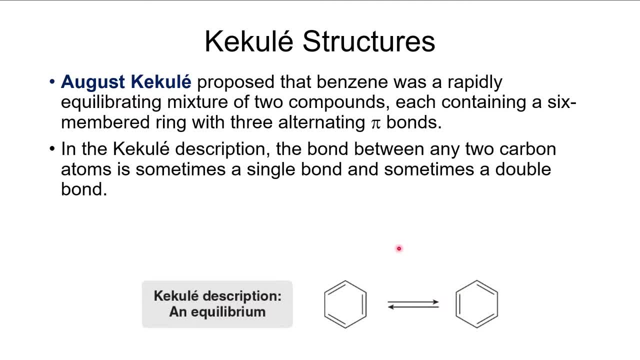 They're a twent century invention. So he didn't have the two-compound compound. We're not talking about the two-compound compound. So now we have a nucleus, the material, the, the ability to think of it that way. so this was insightful, but it's not quite right. benzene: we 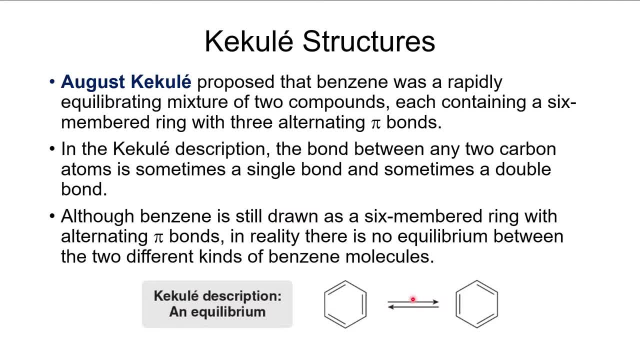 still draw it like this and, in fact, if we, instead of putting the double arrows, if we put a double headed arrow, then it's the correct representation of the two resonance structures, but there's not an equilibrium, as with all resonance structures that we draw, it's not that it's going back and 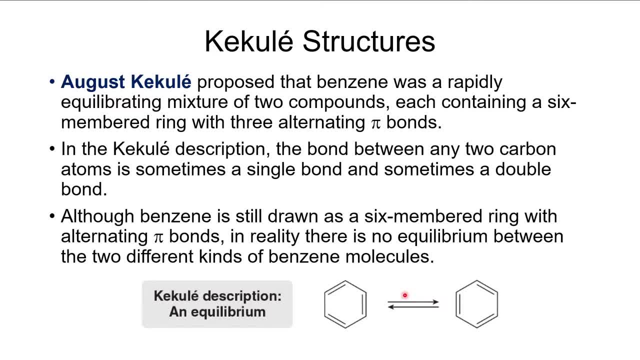 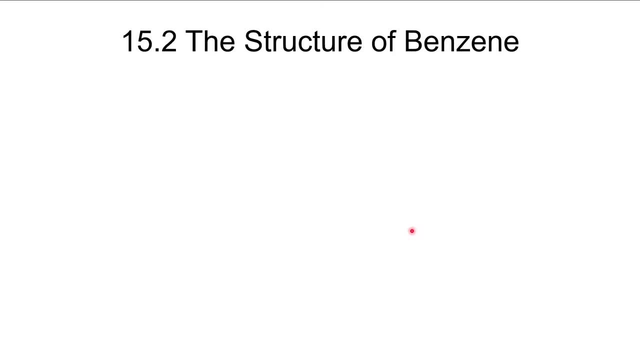 forth between the two. in reality it's it's a combination of the two. so so we don't have two different kinds of benzene molecules. we have one benzene molecule that's best represented by these two structures. so let's look more closely at the structure of benzene if we're going to have a good 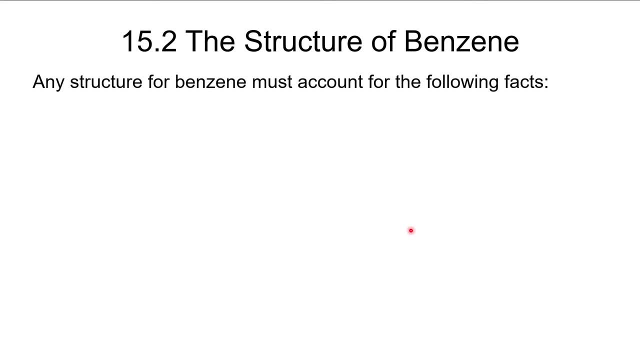 structure, then that structure needs to account for these facts. one: it's a structure that's not going to be a good structure. it's not going to be a good structure. it's not going to be a good structure. it's a six-membered ring and has three additional degrees of unsaturation. kakalai structure: definitely. 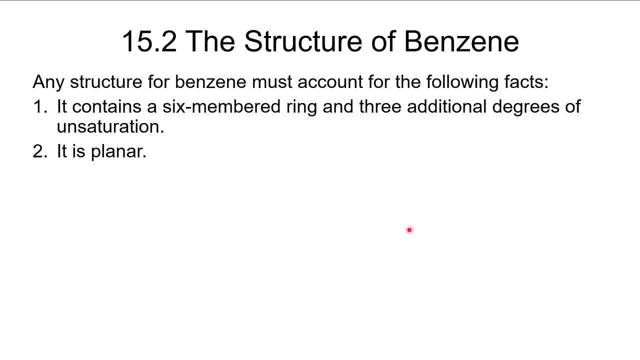 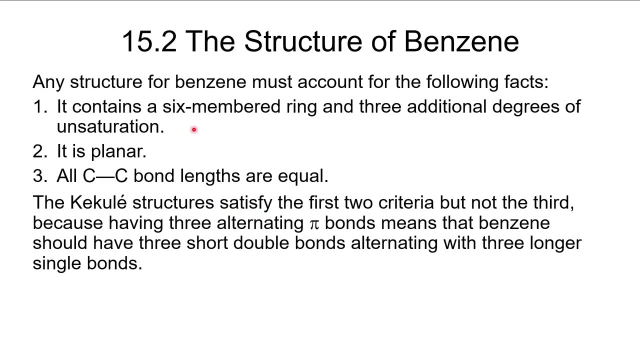 did that. two: it's planar kakalai structure did that as well. three: all carbon carbon bonds have to be equal in length. this is where kakalai structures didn't really work right. kakalai structures, they definitely satisfied the first two, but because it has three alternating. 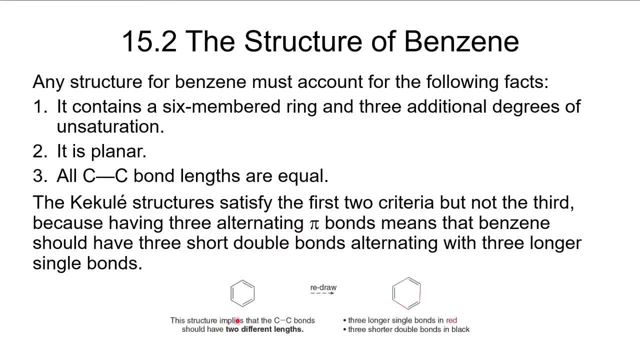 pi bonds. that would imply that we would have three bonds that are shorter, the double bonds, and three bonds that are longer, and that it would be alternating back and forth where the where the double bonds would switch position again. our modern view of benzene is that it doesn't do that. 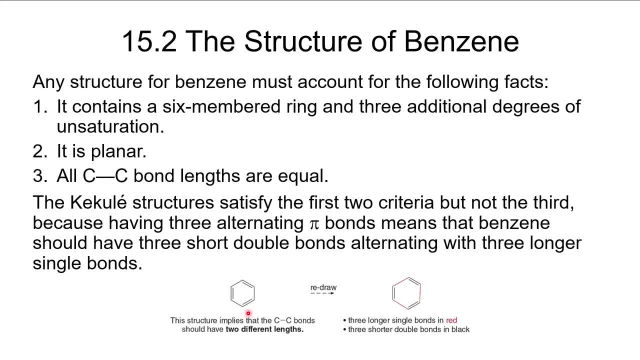 it all six carbon, carbon bonds and benzene are identical, and, and so that happens because of resonance, not because of the resonance of kakalai structures. so that's why we're talking about resonance, not because of the resonance of kakalai structures. so that's why we're talking about. 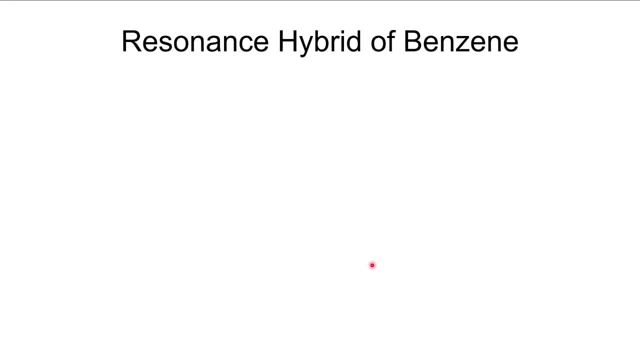 an equilibrium process. so let's look at the resonance structures of benzene. so there are two equivalent resonance structures. we've seen these before. we can easily get from one structure to another just by moving the electrons using our curved arrow notation, moving those electrons so that we get the other structure. and note that here we are using the resonance arrow, not the. 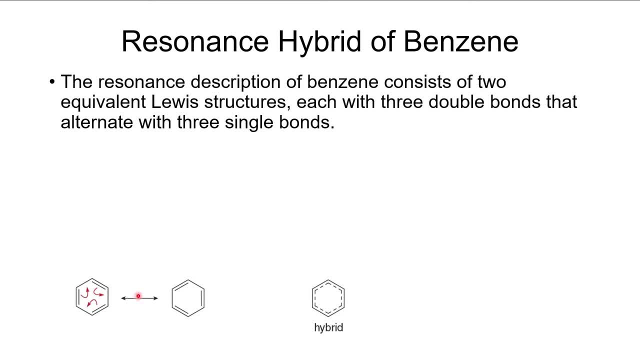 equilibrium arrow. so that's. that's a key difference. the true structure of benzene isn't the one on the left or the one on the right, it's this hybrid over here. that is this: the true structure of benzene doesn't have a full double bond between any of 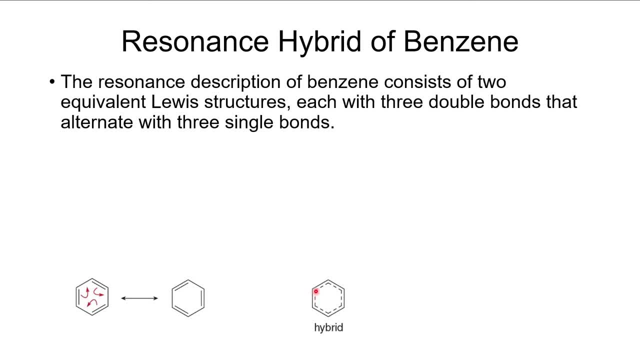 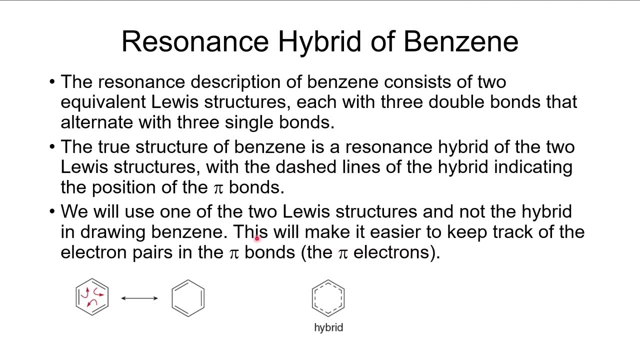 the carbon carbon bonds. it has a one and a partial bond between each of the carbons. so the true structure is the resonance hybrid. the dashed line represent partial bonds. when we are doing mechanisms, we are going to draw the lewis structures, we're going to draw these. 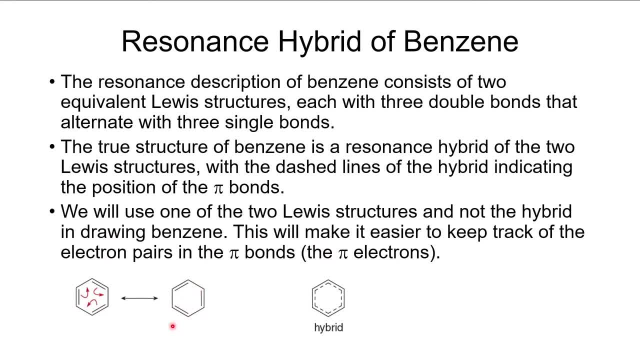 structures of benzene, these skeletal type structures. one, because hybrid structures are not legitimate lewis structures. hybrid structures are very important because they tell us what the molecule actually looks like, but hybrid structures don't tell us. they don't help us to account for the electrons. this very clearly shows that we have six electrons that are going to be in the 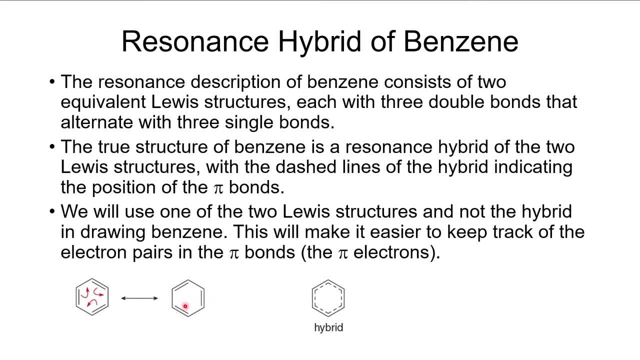 six electrons, that are the that are in p orbitals here, that are in the pi bonds. with this it is a little uncertain as to how many electrons are there. so we like to use, we like to use them, the lewis structures, when we are doing, when we are talking about benzene, when we are talking about its. 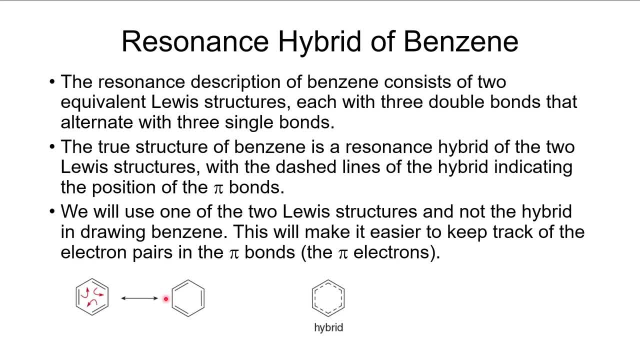 properties and when we are doing mechanisms on the reaction. in some textbooks you will see an image that looks like this and this is a variation of the reaction of hydrogen and oxygen in a portion of the, the hybrid structure. it represents that all carbon carbon bonds have equal length, but again it has 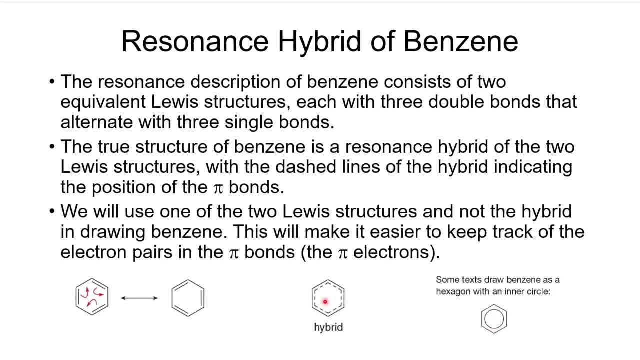 the same problem that the hybrid structure has, in that it's not a legitimate lewis structure and it doesn't tell us how many electrons are actually in the pi bonds. so you won't see me draw this usually and you won't see it in the textbook very often, except in talking about sort. 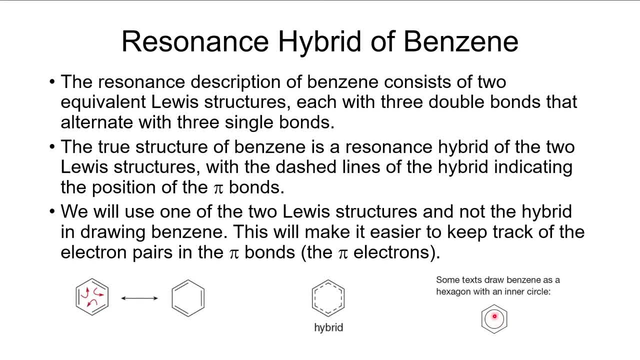 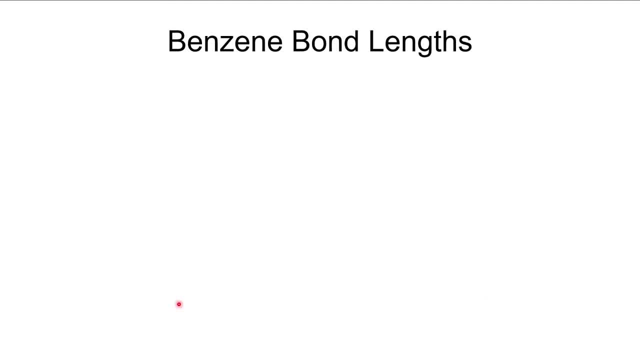 of generalized systems, so it's a quick way to draw it, but it's not an accurate way to draw it. most of the time we're going to use the lewis structures, so one thing we want to look at is the length of the carbon carbon bonds and benzene. as i mentioned, all of the carbon, carbon bonds. 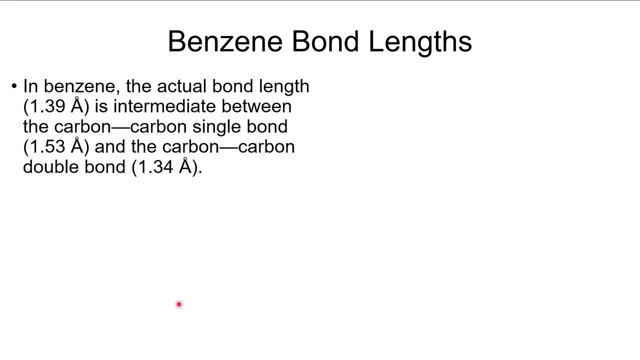 are the same length, and so they come out to about 1.39 angstroms, and that's in between the length of a carbon carbon sigma bond that you would have like in ethane at 1.53 angstroms, or a carbon carbon. 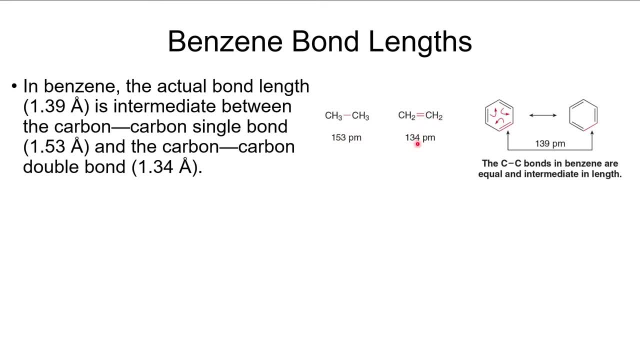 double bond that you would have an ethylene at about 1.34 angstroms, the carbon carbon bond length in benzene 1.39, so it's somewhere in between and since they're all the same, that tells you that none of these carbons are true double bonds. 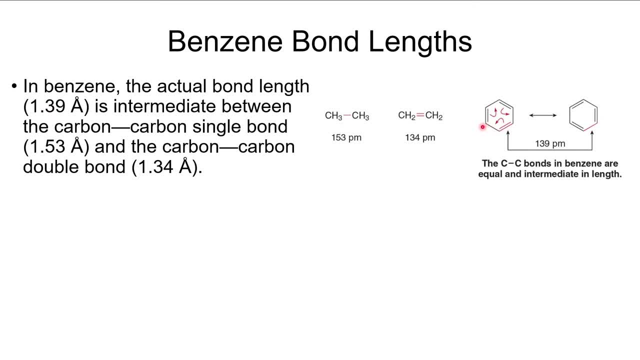 and none of them are true single bonds. they are partial bonds, but they are definitely. they are definitely more than one bond. it's just not a full double bond. we will find that each carbon is sp2 hybridized. it's trigonal planar. that makes sense because 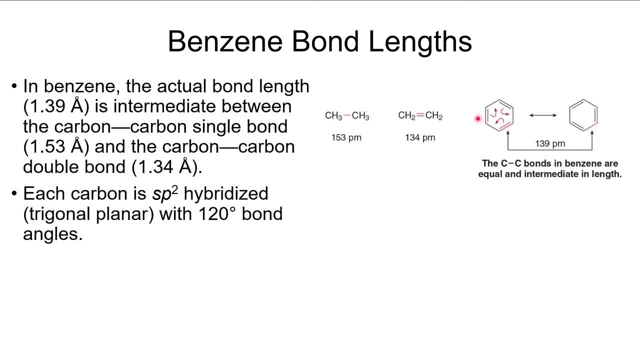 there's, there's three things that are connected to it. so trigonal, planar and all of these things are sp2 hybridized and all of the bond angles are exactly 120 degrees. so has this planar structure 120 degrees sp2 hybridized, which means that the sigma bonds. 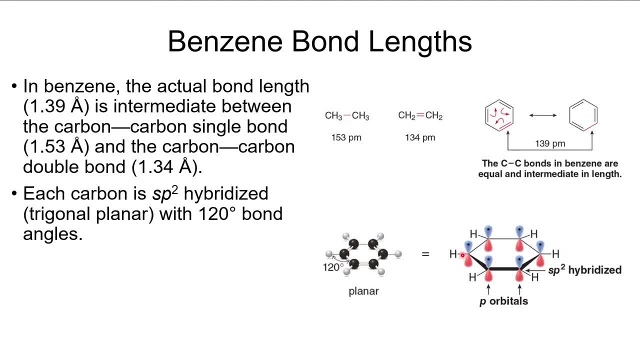 the sigma bonds between the carbons are represented by the overlap of an sp2 orbital on each carbon. the bond between carbon and hydrogen is represented by the overlap of an sp2 orbital with a with a 1s. so the sigma bonds between the carbons are represented by the overlap of an sp2 orbital. 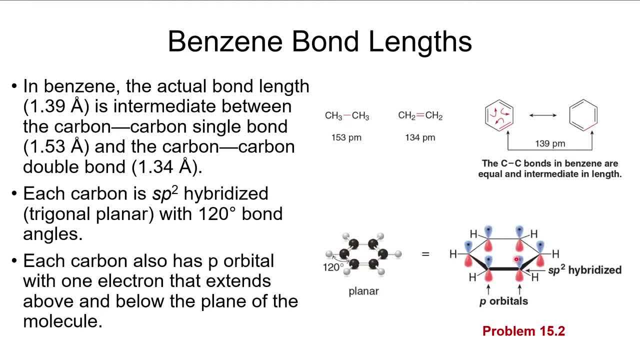 and the 1s are represented by the overlap of an sp2 orbital on hydrogen. all right, the pi bonds are caused by the overlap of these p orbitals which are perpendicular to the plane of the molecule. as i mentioned, the molecule is perfectly planar. all 12 atoms are co. 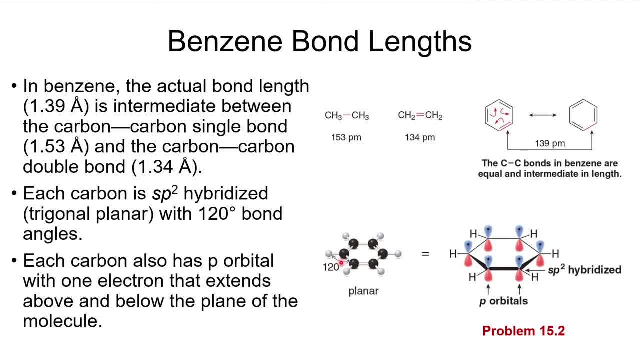 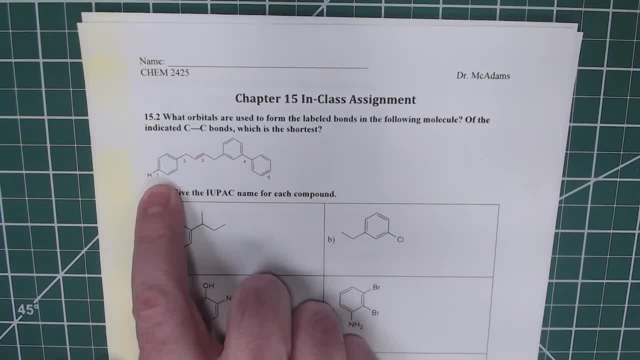 planar and the p orbitals are perpendicular to that plane. So we're going to switch over to the in-class assignment and we want to look at each of these bonds. So what orbitals are used to form the labeled bonds? We have bond 1,, 2,, 3,, 4, and 5.. 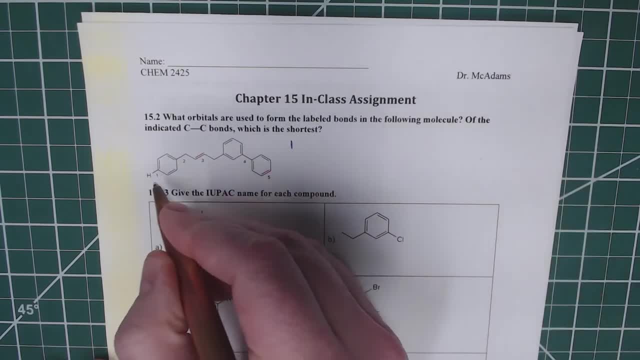 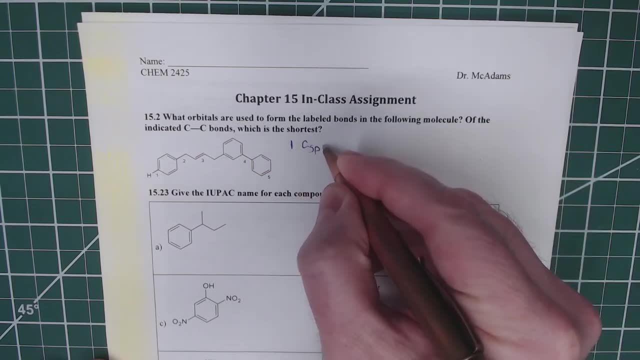 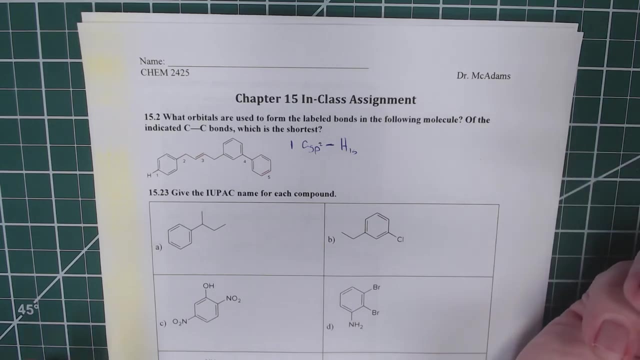 For bond 1, so I'll just put a 1. there we've got a carbon. that carbon is sp2 hybridized. so we'll say a carbon sp2, hydrogen 1s, because the hydrogen has just the one orbital it's. 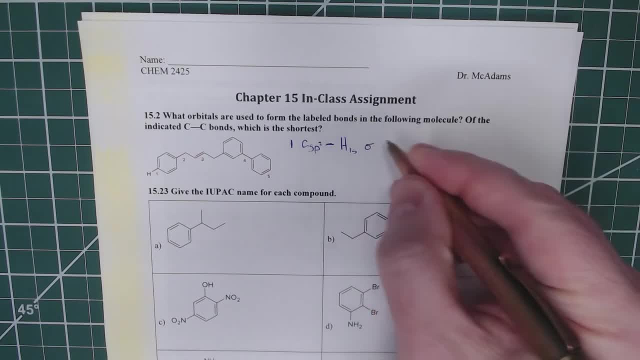 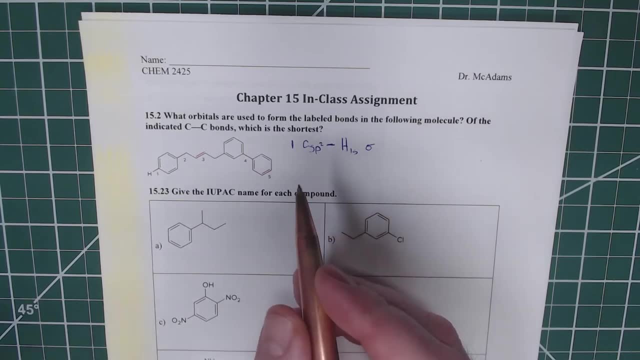 1s, it's not hybridized, and then that is a sigma bond. Any time you've got a carbon that's bonded to another carbon- and we're talking about the sigma bond- it's always going to be the hybrid orbitals of the carbon. 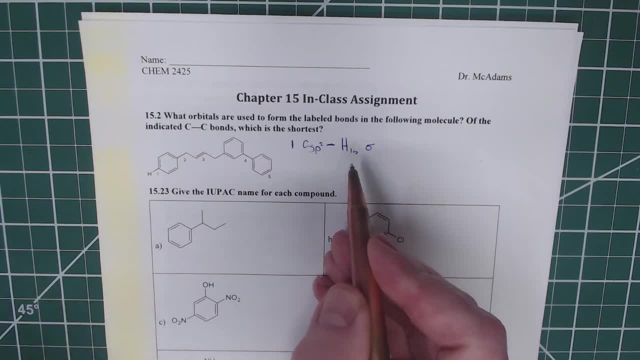 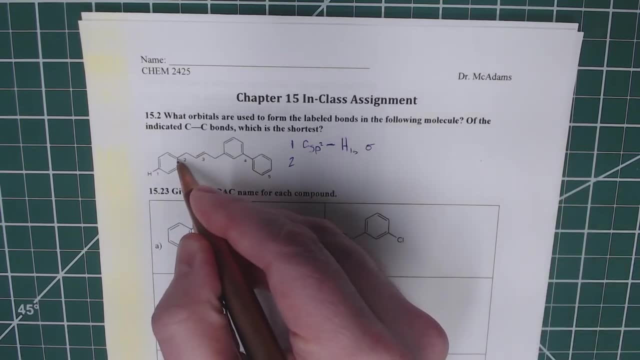 For hydrogen, as I mentioned, there are no hybrids, There are no hybrid orbitals for hydrogen, so it's just going to be 1s For bond 2, we've got a single bond between carbon and carbon, so one of the carbons is 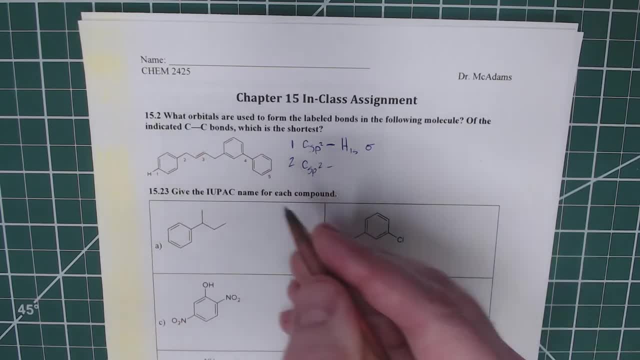 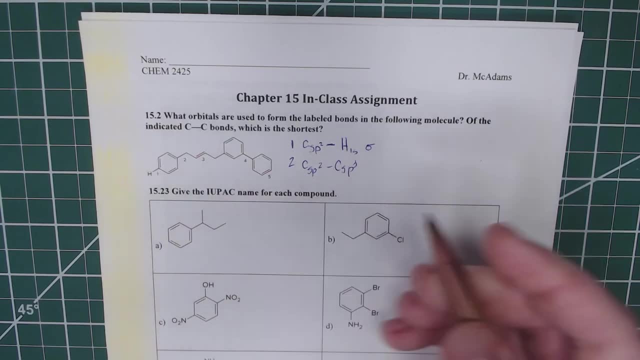 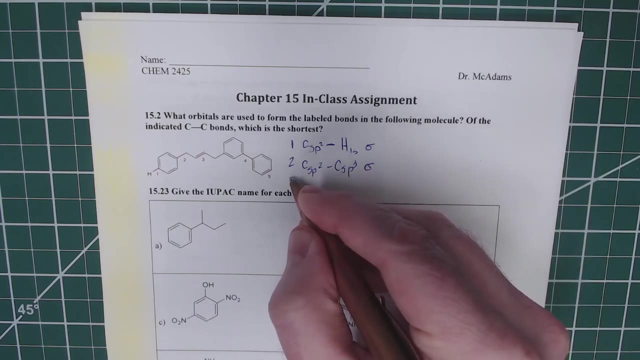 sp2 hybridized. that's the carbon that's on the benzene ring and the other carbon is sp3 hybridized and that is this carbon here And again, that is a sigma bond For bond 3, we've actually got two bonds. 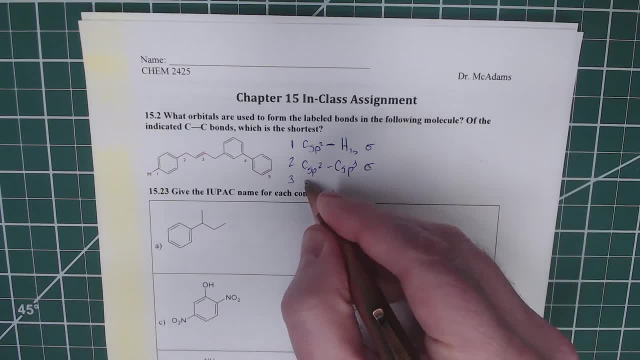 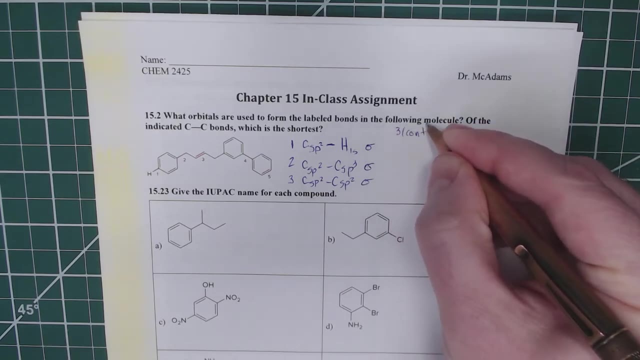 We've actually got two bonds. It's a double bond, so we'll do the sigma bond first. We've got a carbon sp2, carbon sp2, and that is our sigma bond, And then our other bond. I'll do 3 continued here. our other bond is a carbon 2p overlapping. 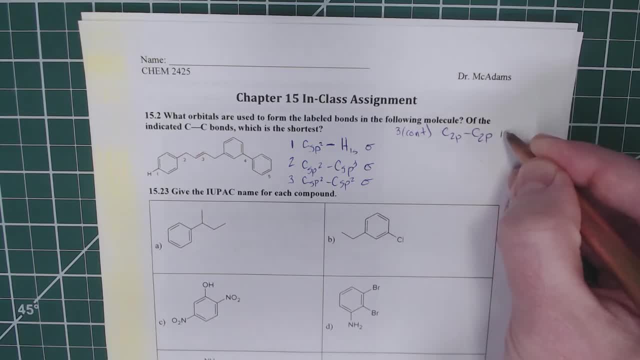 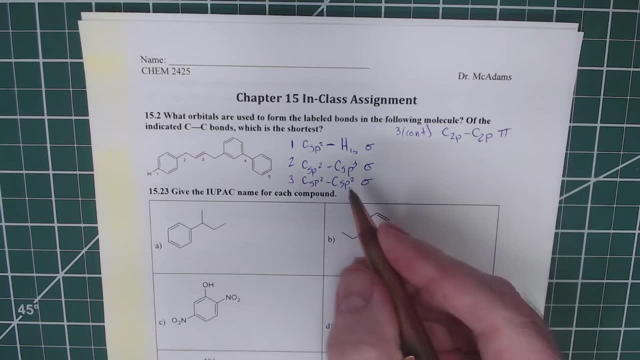 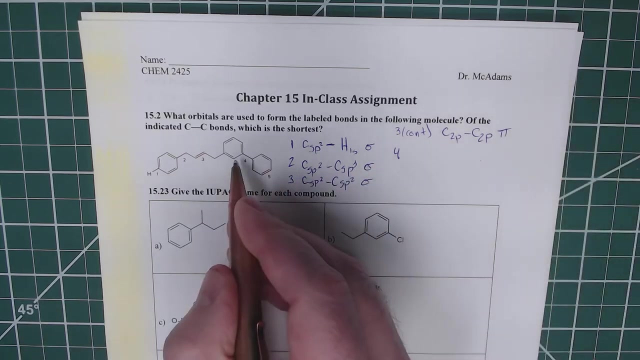 with another carbon 2p, and that is our pi bond. So there are two bonds there, and that's why we have to represent two bonds. in that list, Bond number 4 is a single bond, so we just need to represent the one. 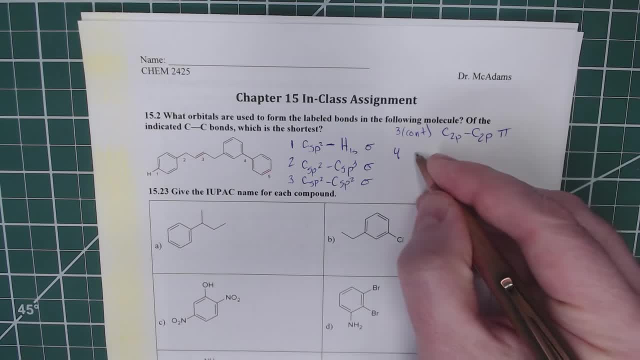 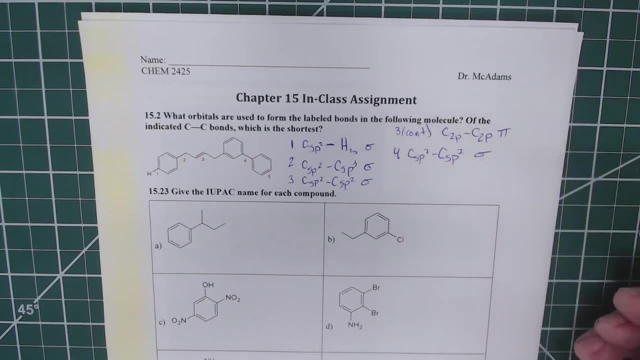 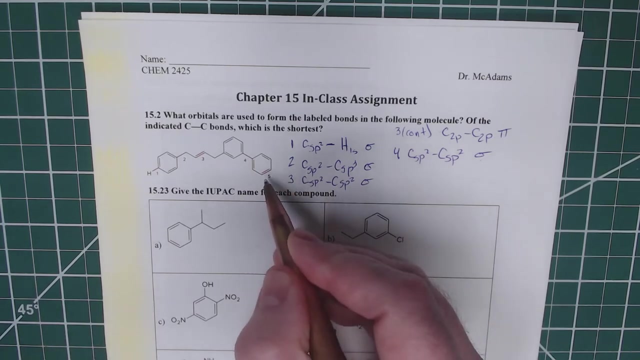 Each of those carbons are sp2 hybridized. so we've got a carbon sp2, carbon sp2, and it's a sigma bond. And that's all there is on bond 4.. Bond 5, we're going to represent it as a double bond. 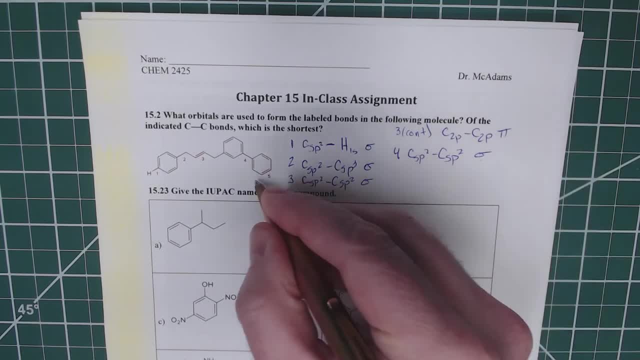 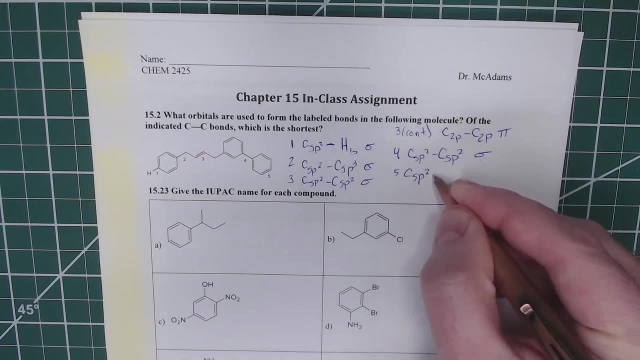 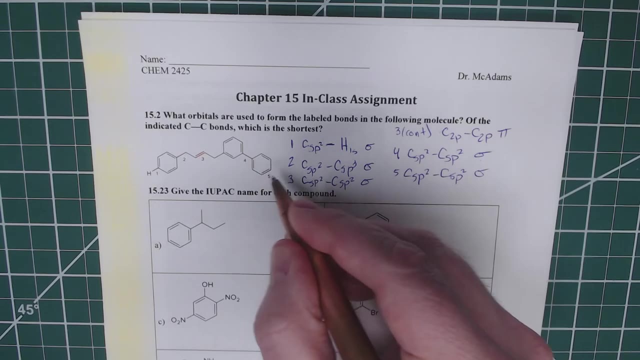 So that carbon- or on that one we've got both of the carbons- are sp2 hybridized. So bond 5, carbon sp2, carbon sp2, and that's our sigma bond And there's also a pi bond in between those two carbons. 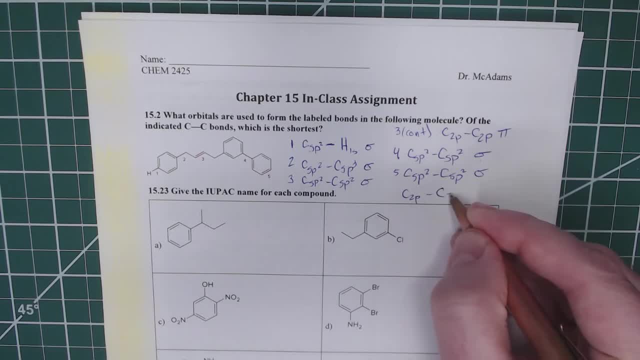 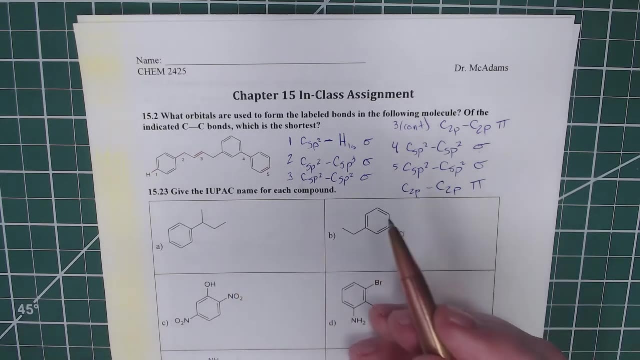 So we'll put carbon 2p, carbon 2p and that's our pi bond. So there's two bonds with bond 5.. Now the other part of this question of the indicated carbon-carbon bonds, which is the shortest. 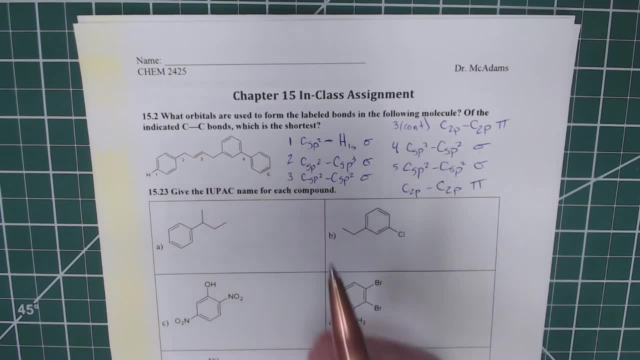 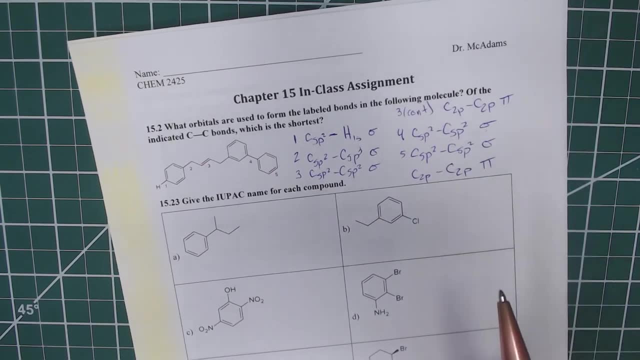 So, between carbon 2,, 3,, 4, and 5,, which one is going to be the shortest? Well, the one that is a true carbon-carbon double bond will be the shortest. So carbon 3 will be the shortest. 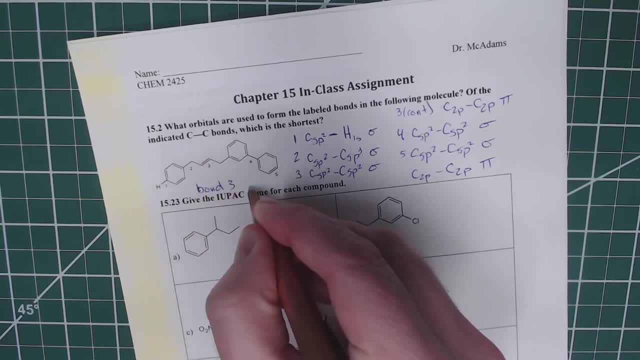 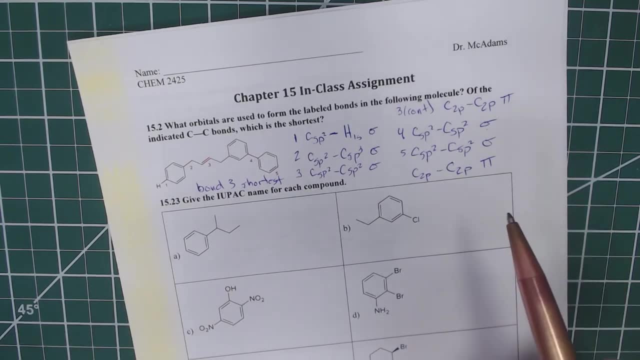 Our bond 3 is our shortest. Now we could go through and determine which ones do we think are the longest. Our longest should be the sigma bond, that's sp2, sp3.. This other one that's sp2, sp2, it would be pretty close, but probably a little bit shorter. 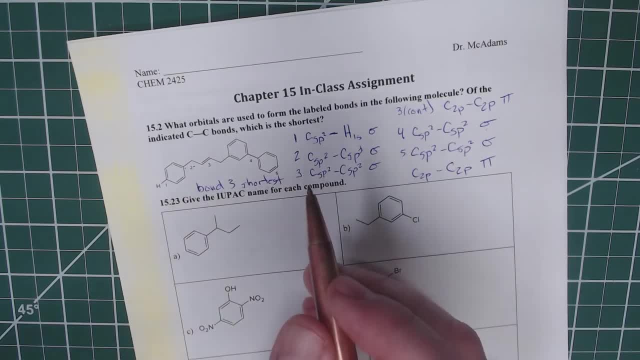 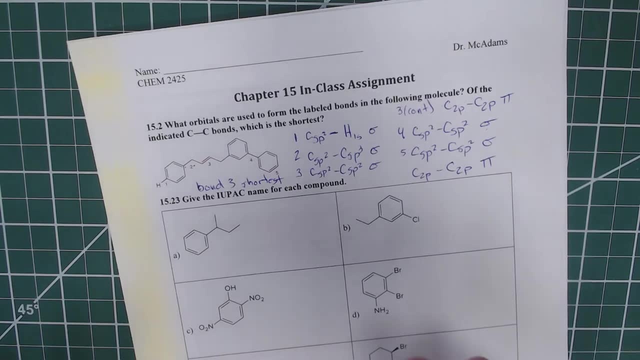 than bond number 2.. But our definitely shortest bond should be bond number 3 between that carbon-carbon. It's an isolated carbon-carbon double bond, So it's got 100% double bond character on it. No resonance structure Okay. 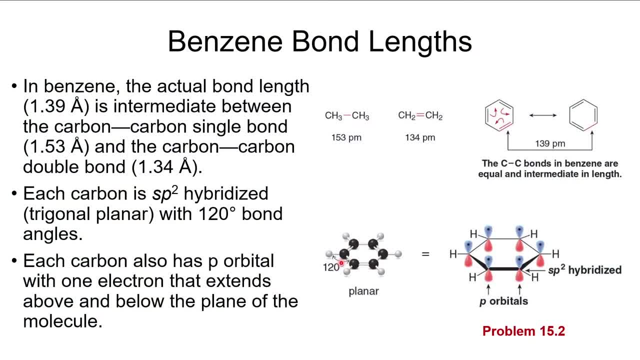 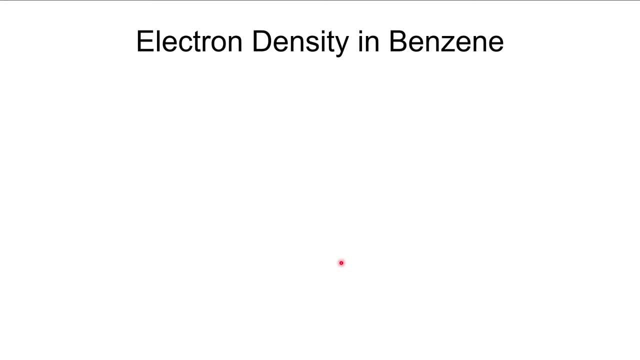 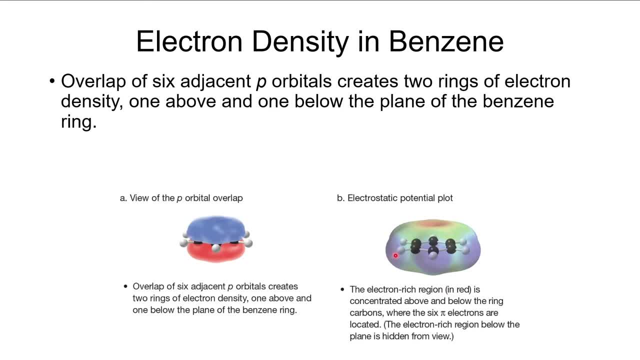 That means that, technically, there is a partial positive charge on these hydrogens and a partial negative charge on the carbons. Now, it is a small charge, but it is there. It is there. Now I'm going to show you a molecular model, one that I 3D printed. 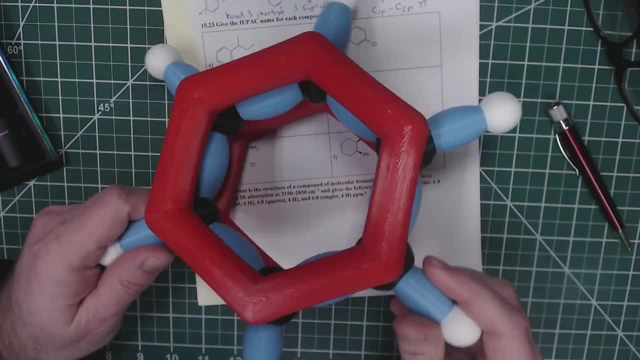 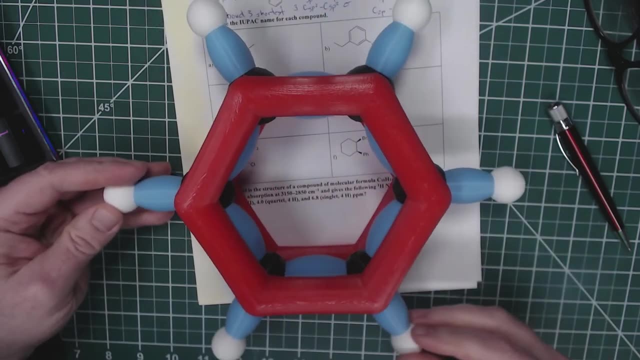 I'm going to go back to this image. So this is a molecular model that I made for my classes. I designed it and 3D printed it. The carbons and the hydrogens- all six of them- are coplanar, so they're all in a plane. 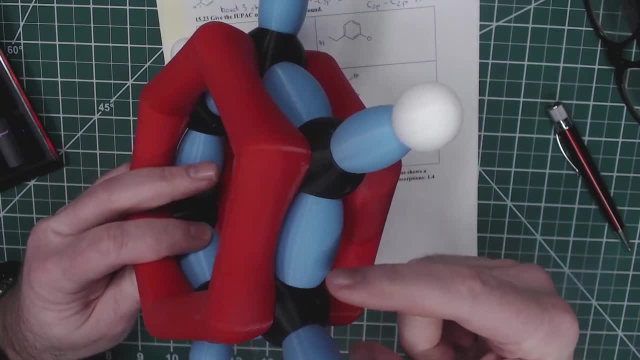 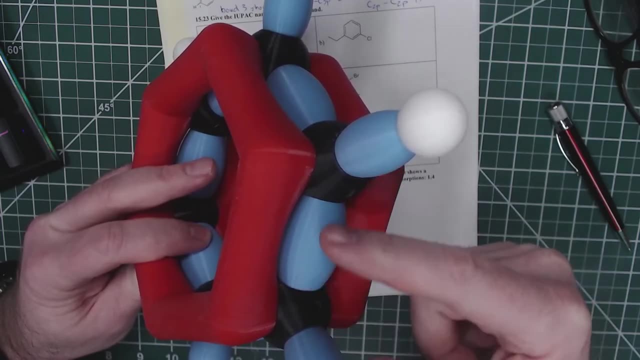 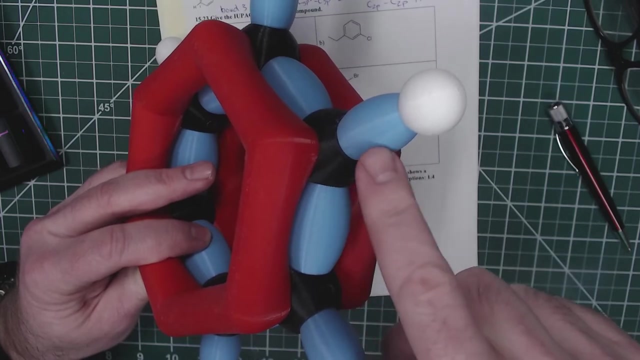 Between each of the carbons. the blue bonds here are the overlap of an sp2 orbital on carbon and an sp2 orbital on the adjacent carbon. So that is represented by that overlap, sp2 and sp2.. The carbon hydrogens are represented by the overlap of an sp2 orbital on the hot carbon. 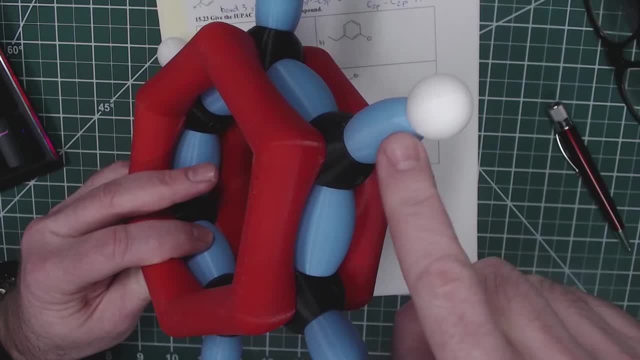 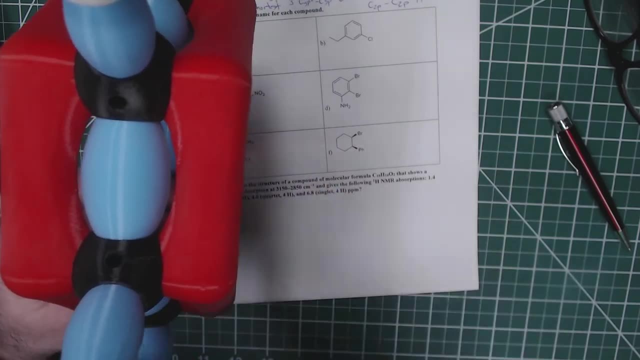 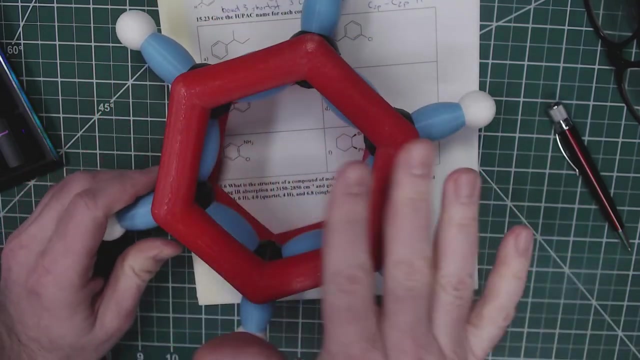 and a 1s orbital on the hydrogen, And so that is the overlap there. The p orbitals: here they're shown as a pi system but the p orbitals are perpendicular. They're perpendicular to the plane of the molecule and they overlap in a ring on the top and on the bottom. 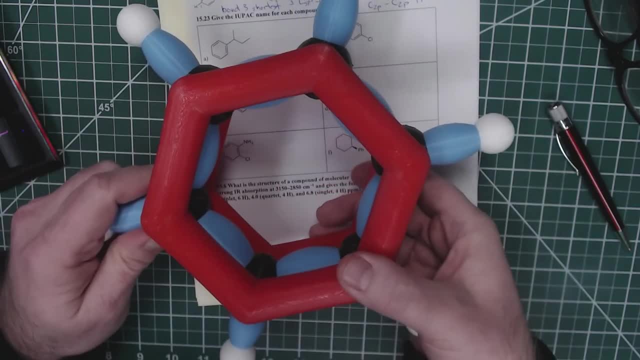 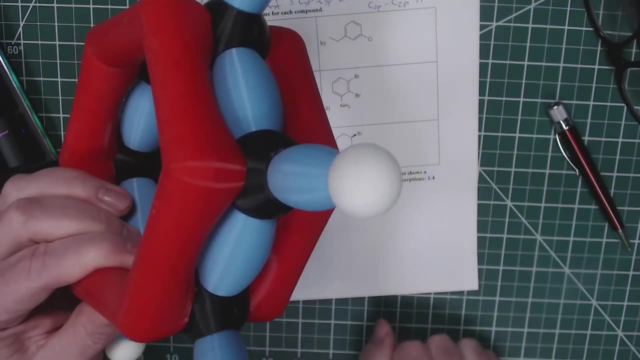 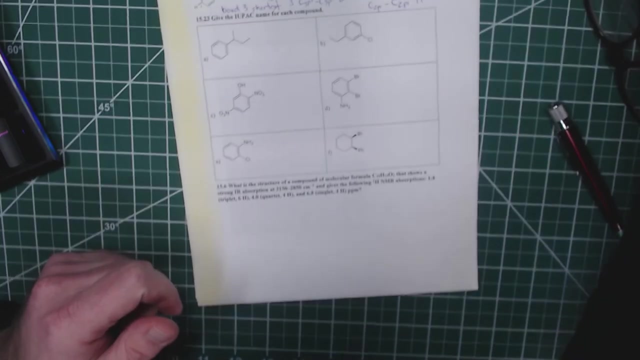 Now remember that pi system is both the top and the bottom. They're not separate, They're all one system, just like a normal pi bond. So that would be our structure of benzene. Now I've got another one here. 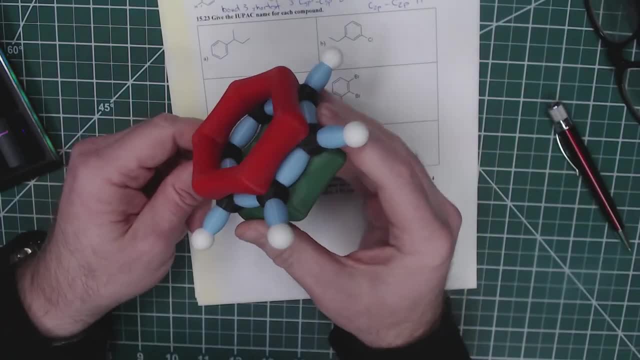 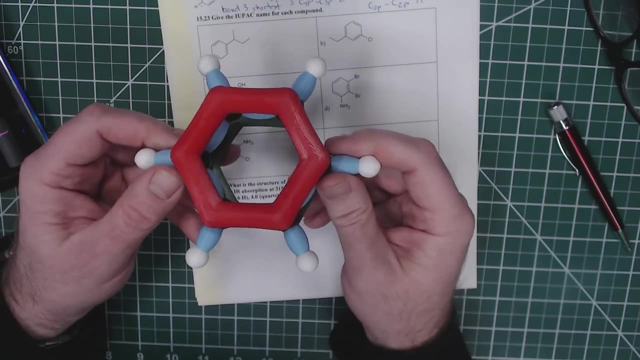 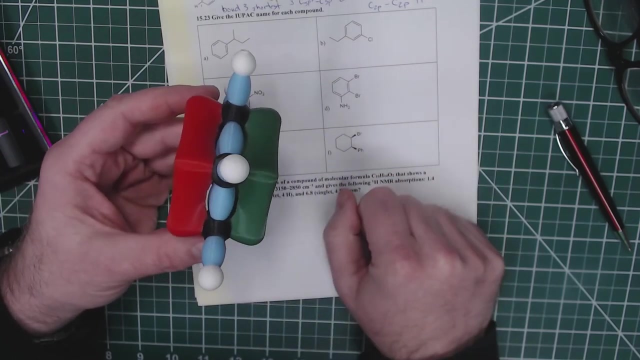 This one. this one's kind of cute. I made this one as a Christmas ornament that I gave out to my friends a few years ago. You know my friends have come to expect that they get kind of nerdy gifts, So this is one that I again designed it. 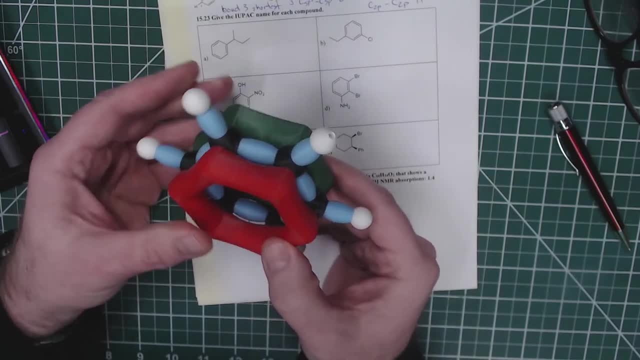 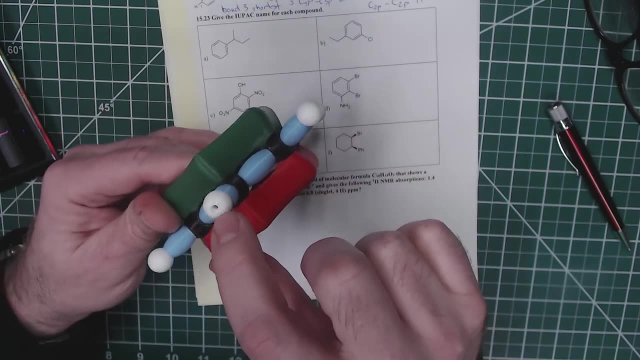 I designed it, 3D printed it and then gave it out to my friends And I made one side of it red and the other green, so it would look like a pretty Christmas ornament. And you can see right there that I just put a hook on there and it hangs on the tree. 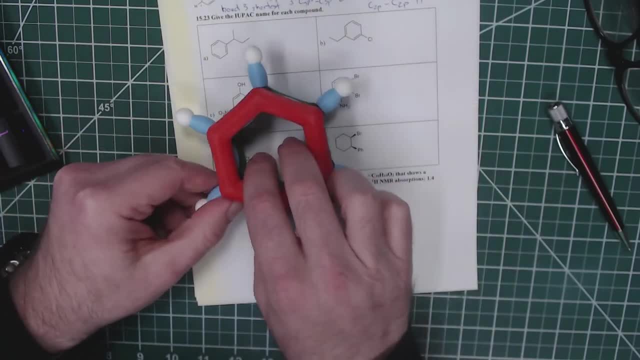 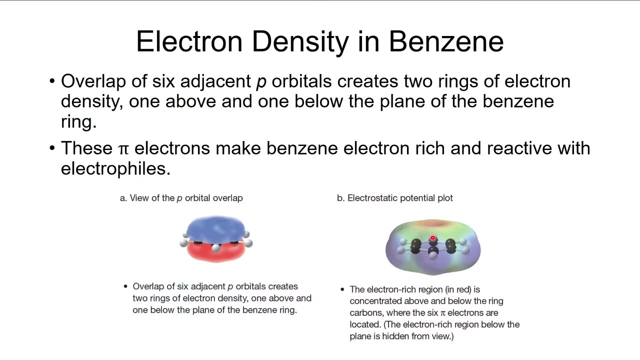 Kind of cool. All right, so let's go back. Next we're going to do the bottom, So I'm going to take the bottom off And we're going to put the bottom on the top, And then we're going to put the bottom on the bottom. 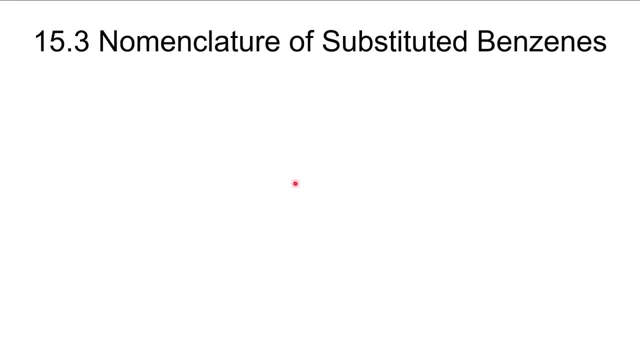 And then we're going to put the bottom on the top, And then we're going to put the bottom on the bottom, And then we're going to put the bottom on the bottom. we want to look at the nomenclature for these aromatic hydrocarbons, these substituted benzenes. 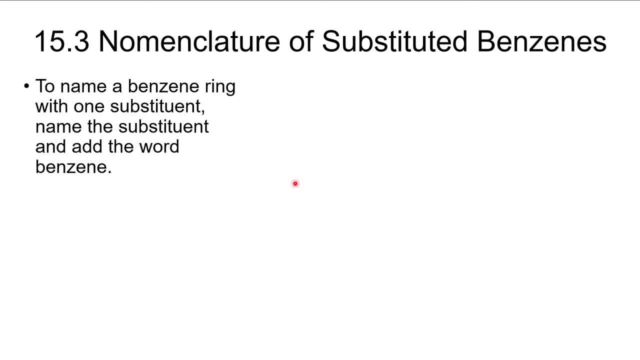 so to name a benzene ring with one substituent, you simply name the substituent and then add the word benzene to the end. it's pretty easy, and because- uh because- whatever that substituent is is carbon one. we don't have to put a number on mono substituted benzene rings. so this is simply. 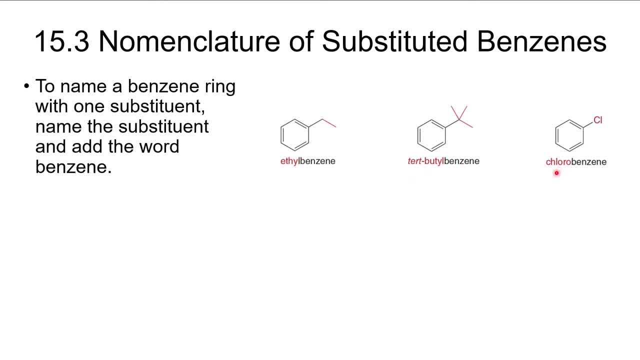 ethyl benzene, tert butyl benzene and chlorobenzene. there are a few names that we use that have common names that are associated with them, and in fact they're so common that they've become part of the iupac nomenclature system. 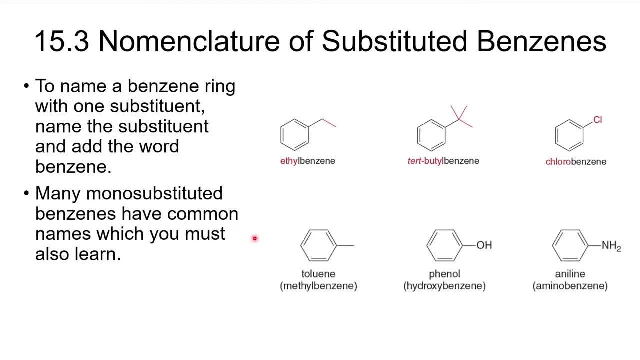 and so these are mono substituted benzenes that have their own special names, and so um. so. this one is called toluene methylbenzene. it's toluene. toluene is used as a solvent, an alternative to using benzene. it's it's got some of the good properties that benzene has. 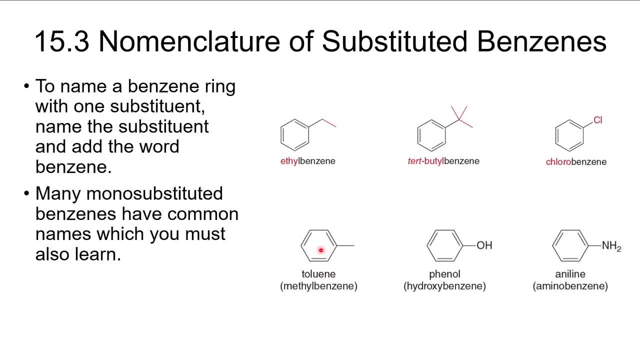 but it's not nearly as carcinogenic, so it's desirable that way. hydroxybenzene: we refer to that as phenol phenol- you may have heard of that in terms like for medical use. it's called carbolic acid and it is a very effective antiseptic. it's also a little bit poisonous, but you know, hey. 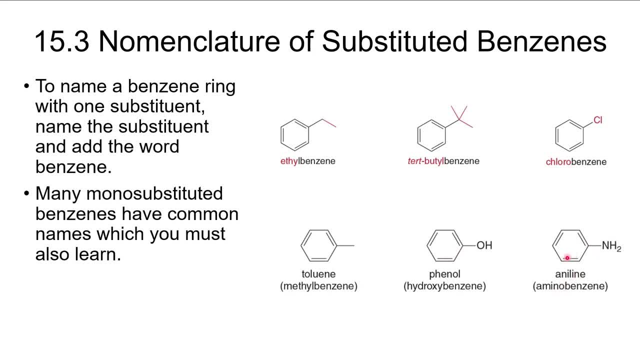 most of these are poisonous. and the next we've got aniline. aniline is amino benzene and that is just the common name for that compound is aniline and, as i mentioned, these have become such common names that they have been incorporated into the iupac system. 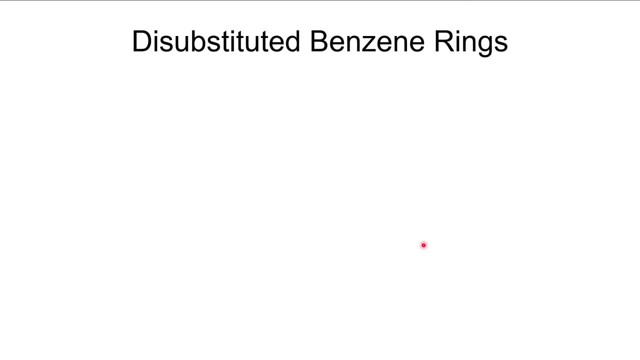 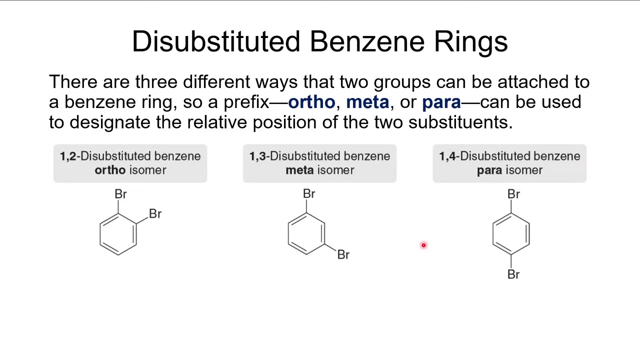 because they're a lil bit higher intuition than linoleic acid, how linked it is to aberrate and what i'm going to teach to you today will basically have 1, 4 substitution. we refer to that as para, which means opposite, So ortho is adjacent meta. 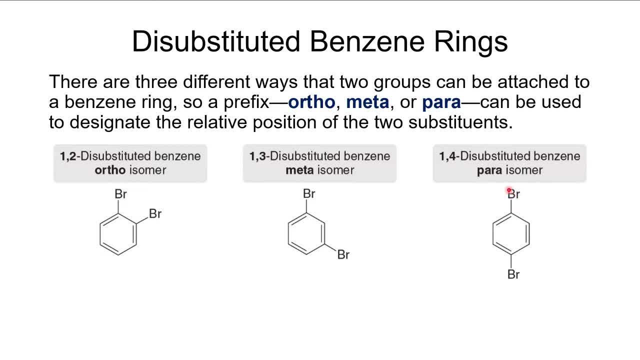 is in between and para is opposite, So 1, 2,, 1, 3, and 1, 4.. That means that you can name this in two different ways. You can refer to this as ortho-dibromobenzene, or you can refer to it as 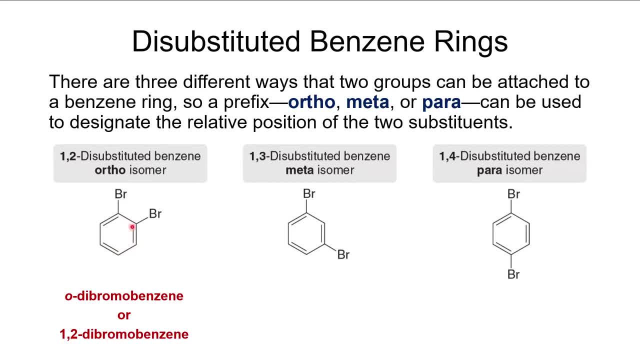 1, 2-dibromobenzene. 1, 2-dibromobenzene, Both of these are correct, So ortho-dibromobenzene or 1, 2-dibromobenzene, both of those are satisfactory. You need to know, of course, you know the numbers. 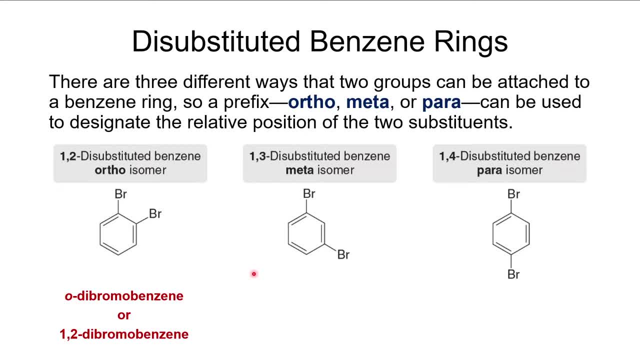 already, but you need to know what the ortho meta and para mean. if you see it, This one we would call meta-dibromobenzene or 1, 3-dibromobenzene, And this one would be para-dibromobenzene. 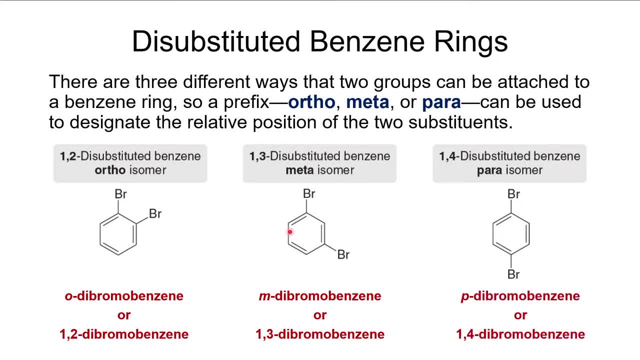 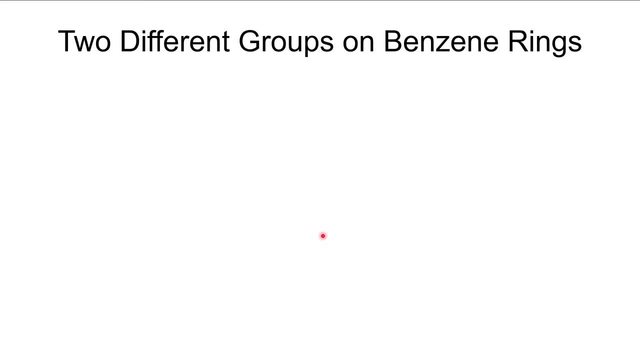 or 1, 4-dibromobenzene. If you have two different groups on the benzene ring, then we need to know what order to put them in. If it's two different groups and it's not part of a common name, then we are going to. 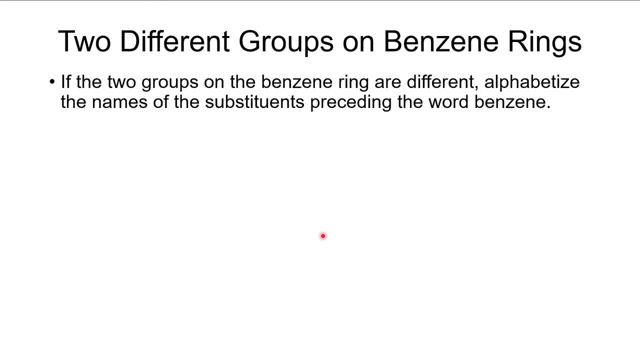 alphabetize the substituents, where the first one alphabetically gets the one position and the second one gets whatever the other position is. For example, here we've got a bromo and a chloro. Since B comes before C, this would be ortho, and these are ortho to each other. this would be ortho-bromochlorobenzene. 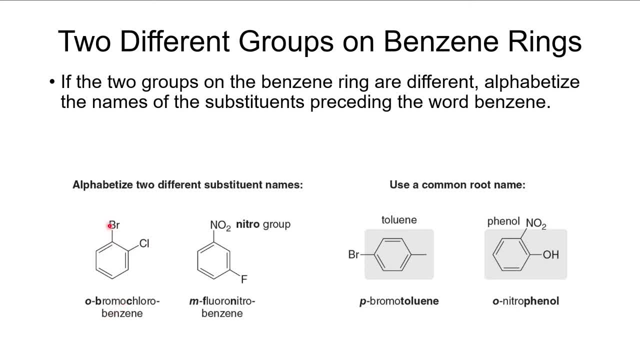 It would also be accurate to call this 1-bromo-2-chlorobenzene. That would be an accurate description of that molecule. On this one, we've got nitro and fluoro. fluoro comes first alphabetically before nitro, and so, as a consequence, we would call this: 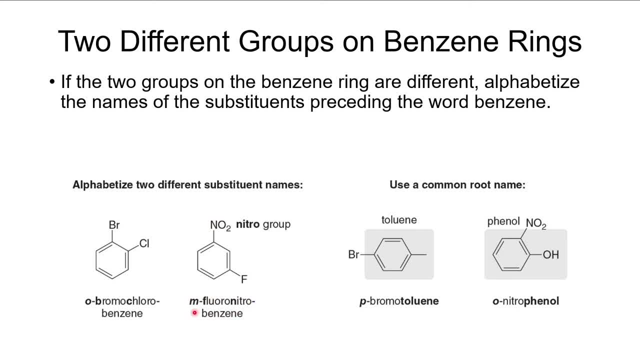 metafluoronitrobenzene, Or we could call this 1-fluoro-3-nitrobenzene- That would also be a correct name. I will be doing it both ways if we have a disubstituted benzene ring. 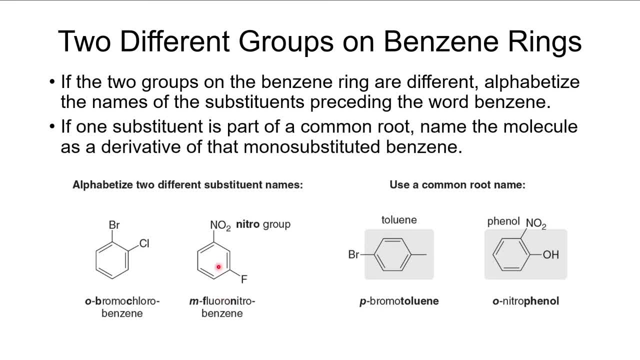 Another thing that we will see is if one of the substituents makes up one of our common names- toluene, phenol or aniline- I had to think what. the other one was there. So toluene, phenol or aniline- then we're going to name the molecule. the parent name is going to 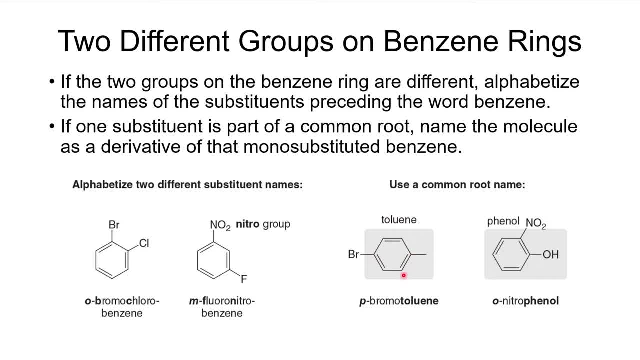 be the name of whatever that common name is. So this would be toluene. Whatever the position of that is, that's the one position. The toluene has a substituent that's methyl. we're going to call that the 1-phluorobenzene. So that's the one position. We're going to call that the 1-phluorobenzene. 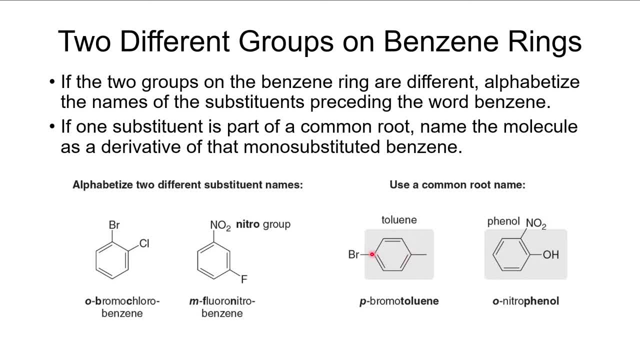 And so this bromo is in the 4-position or the para-position, So we could call this para-bromotoluene or we could call it 4-bromotoluene. That would be sufficient On this one. 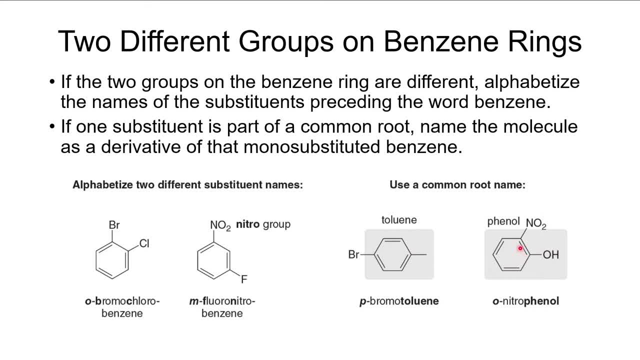 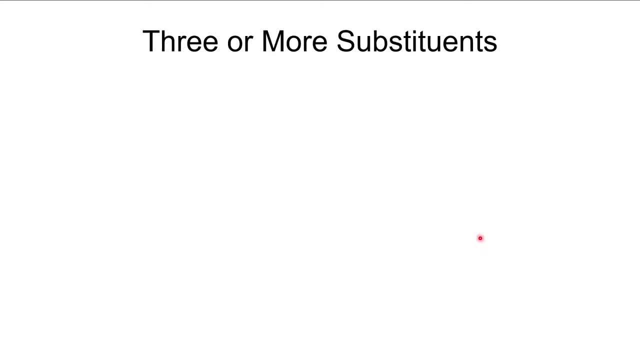 we have ortho-nitrophenol, or again we could call this 2-nitrophenol. Well, what if we have three or more substituents? In that case we're going to not use the ortho-, para- and meta-prefixes. We only do that for disubstituted, For trisubstituted. 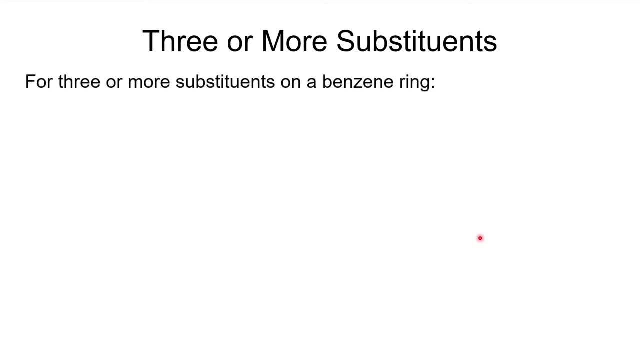 we're going to stick with the numbering, So we want to number to give our lowest possible numbers around the ring, And so in the case of this, we've got three substituents, Since we have two that are adjacent, the two that are adjacent are going to be one and two, And since we have 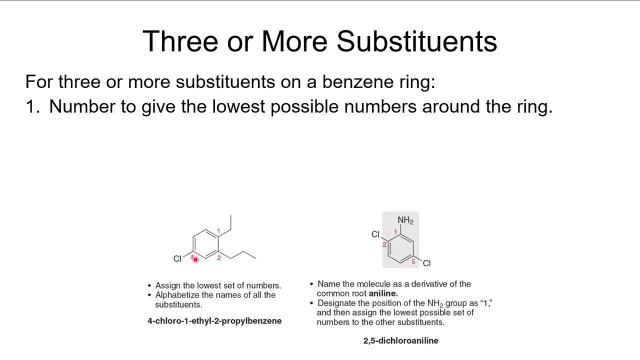 one that's here. opposite of this ethyl we have this chloro. then we're going to number clockwise to give that one the lowest possible number. If we called this one one and that one two, this would be five. So we want to number it to give this also the lowest possible. 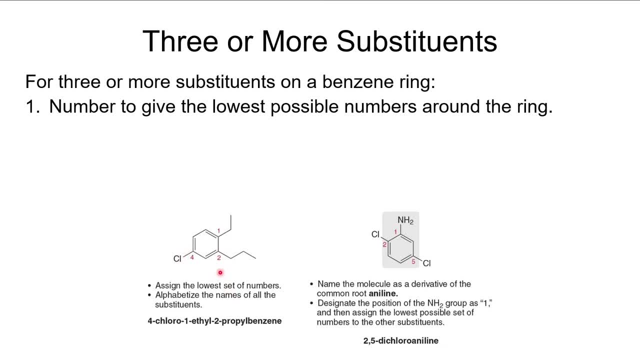 number. So in this case we would number it that way, but then the naming is still going to be alphabetical. So we have an ethyl group, a chloro group and a propyl group. Well, chloro comes first alphabetically, so it would be four chloro, one ethyl, two propyl benzene. So we 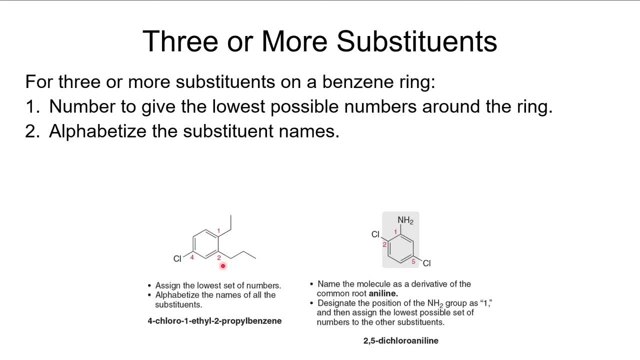 alphabetize the substituent names. If we have a common root, so toluene, phenol or aniline- and in this case we have the aniline- then we're going to name the molecule as a derivative of that monosubstituted benzene. So this would be aniline and we would have. we would have. 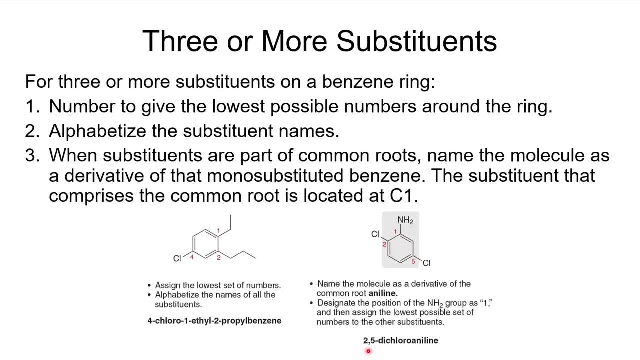 chloros at the two and the five position. So this would be two, five dichloroaniline, And so this is a little bit different than this. You know, if we were going to number this the same way we would, you know, we would call this two amino, one, four dichlorobenzene. But here, since we're going to 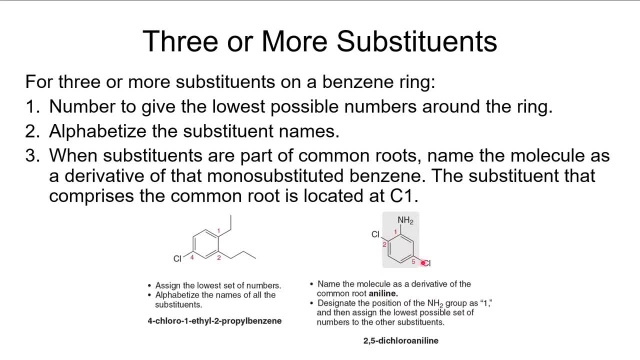 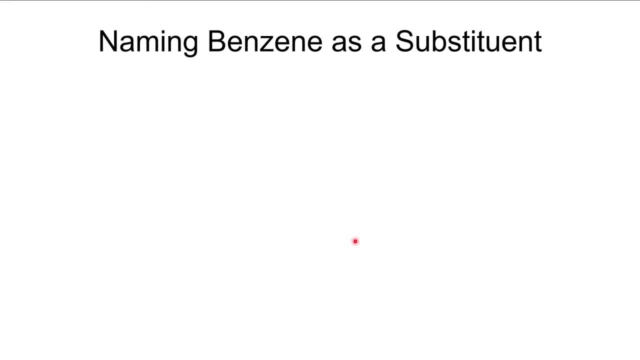 name it after aniline. we're going to call it two five dichloroaniline. All right, In the case that we're going to be using a phenyl group, we're going to call that a benzene ring as a substituent. Well, if it's a substituent that is directly attached, we're going to call that a. 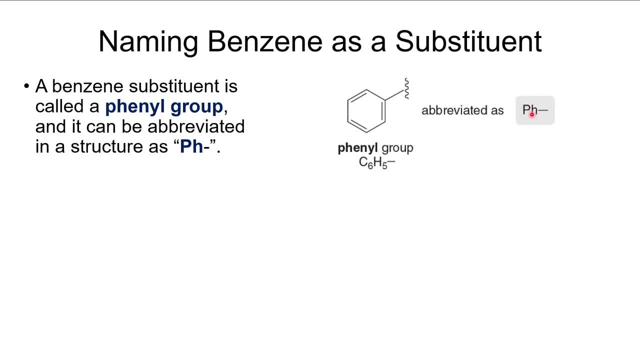 phenyl group, And so we can represent that shorthand. We can just put P H uppercase P, lowercase h for the phenyl group. We can also write it as C6H5 dash as a substituent if we don't want to draw out the entire benzene ring. Sometimes it's not convenient to draw out that entire. 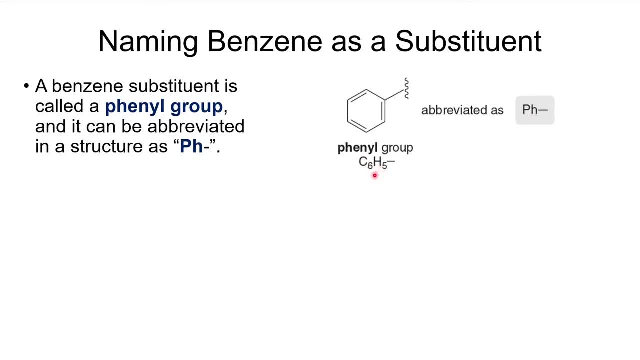 benzene ring Or the C6H5 dash would be sufficient. All right, That P H. we can use that in other contexts. So anytime we have a benzene ring and we're trying to do shorthand, we can put the P H in place of. 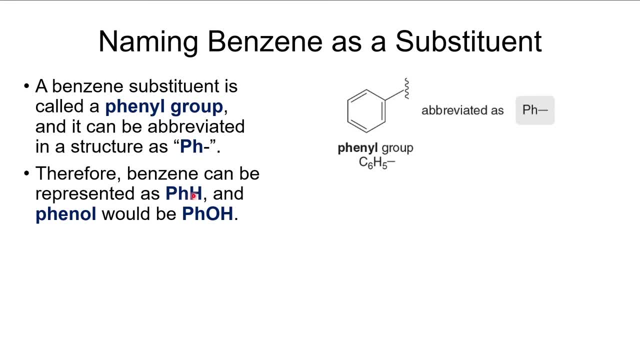 the phenyl group, which is the C6H5, and then whatever's attached, So P H and then uppercase H. we can represent that as benzene. And if we want to represent phenol, we could do P H, lowercase O H, And that is another way that we represent. It's a shorthand way of representing. 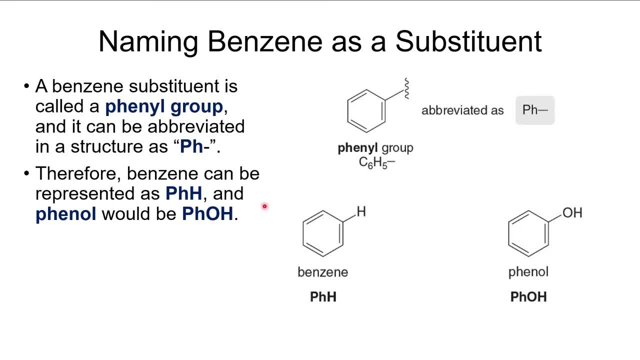 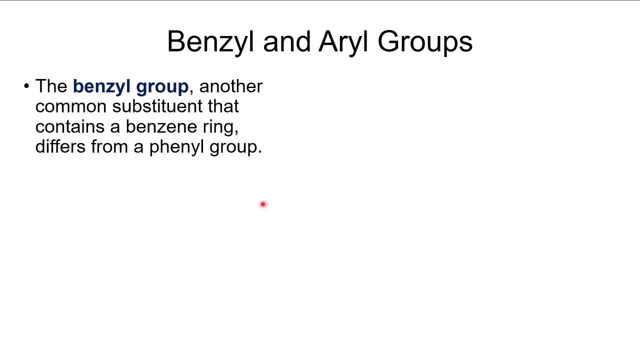 phenol. All right, One other thing, and that's benzyl and areal groups. The benzyl group is a little bit different than a phenyl group. A benzyl group has a phenyl group in it, but it also has a CH2, and then that is attached to whatever your substituent is. 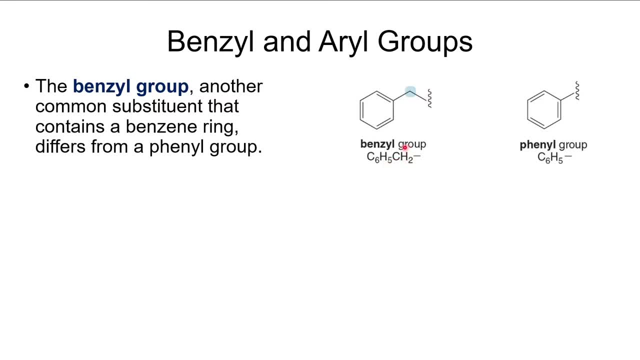 So it's C6H5CH2.. The reason that we separate out benzyl groups is that benzyl carbons have special reactivity. We're going to see all kinds of examples where we can do reactions at that benzyl carbon that we wouldn't be able to do on a normal SP3 hybridized carbon. So you want to be? 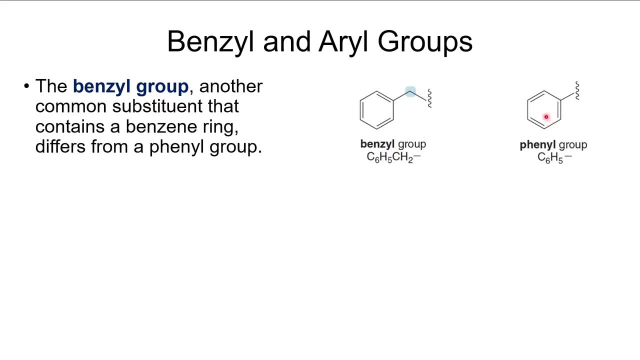 able to differentiate between the benzyl and the phenol And in case you're wondering what's the difference between the benzyl and the phenyl, If you're curious, if you want to abbreviate the benzyl so we have pH for phenyl, you can. 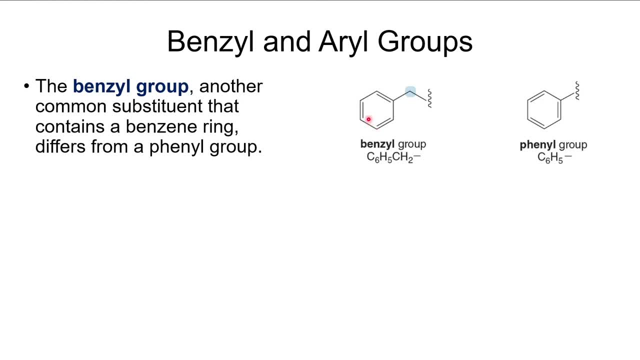 abbreviate benzyl by putting uppercase B, lowercase N. I say that because I don't want you to use BZ. We use BZ for benzoil- We'll get to that one later- but that one involves a carbonyl. 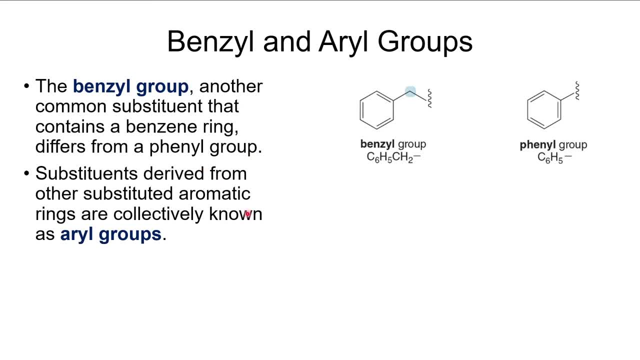 And then, generally speaking, if we are referring to substituents that have aromatic rings in them, we're going to refer those as areal groups. So areal hydrocarbons or areal components are going to have a benzene ring in it. So this toluene or tolyl is an areal group. So there we go. 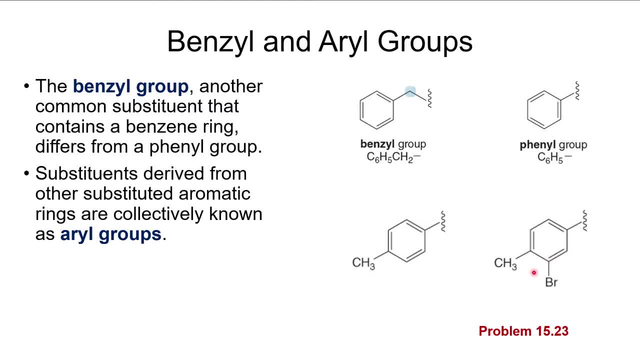 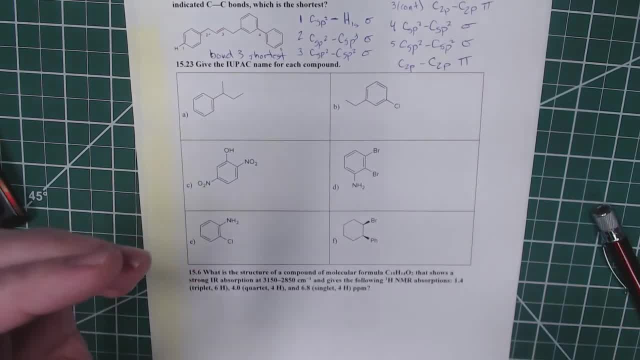 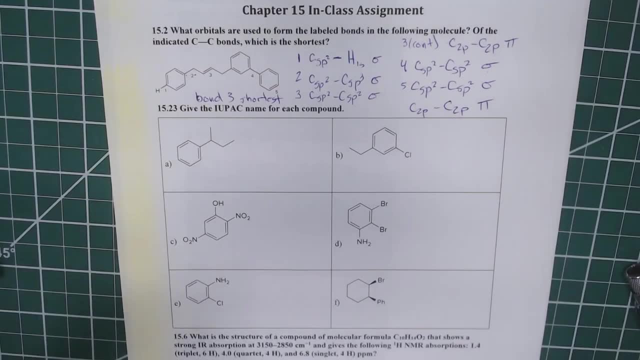 So let's look at number 23, and we're going to give IUPAC names for several compounds. I'm going to switch over here, All right, I'm going to lower my camera just a smidge here. All right. For monosubstituted, very easy, We just name whatever the substituent is. 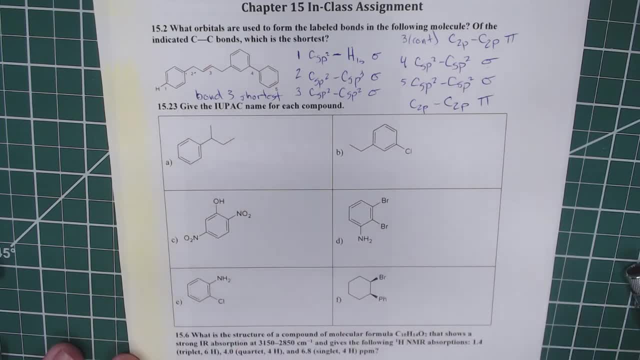 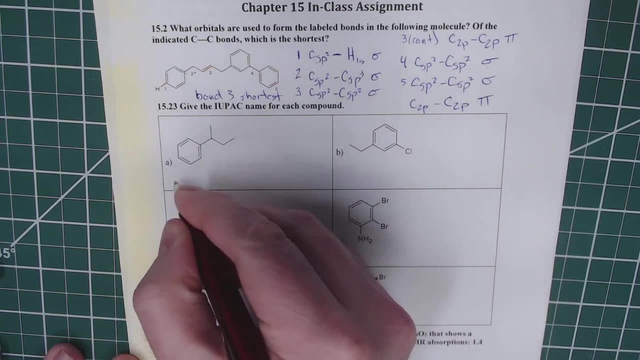 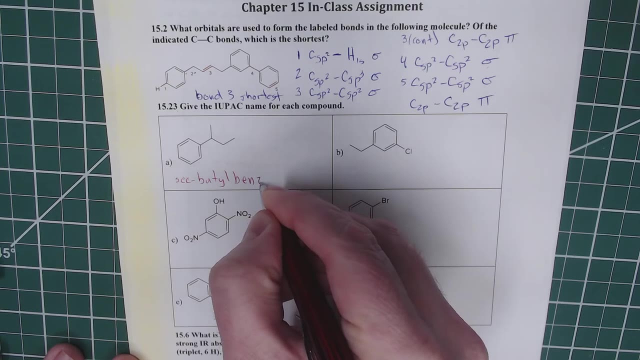 and benzene. And because that substituent it's a butyl but it's attached to the second carbon on the butyl, we call this sec butyl. So this we refer to as sec Butyl Benzene, So sec butyl benzene. 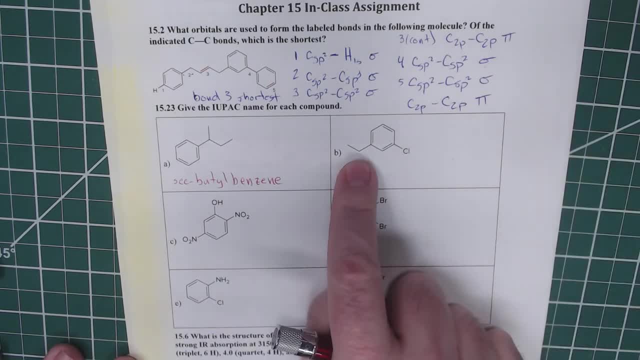 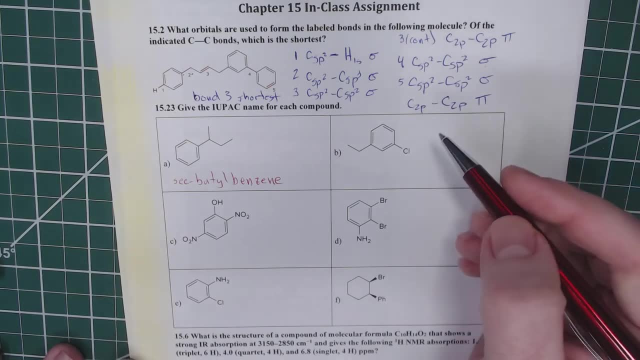 All right, Here we've got two substituents. We've got an ethyl and a chloro. We need to indicate which one is which. We're going to do the chloro, because it's disubstituted. we're going to do the. 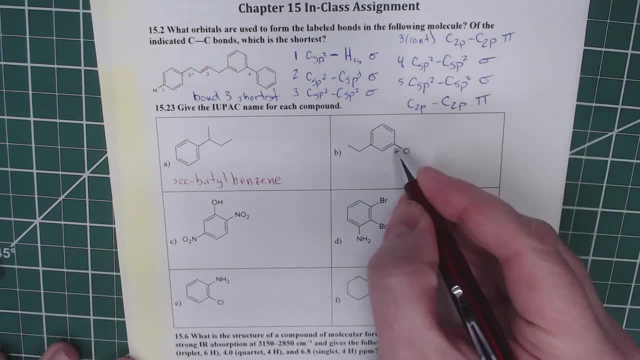 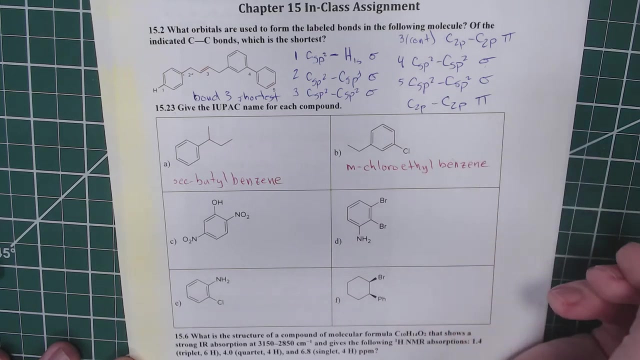 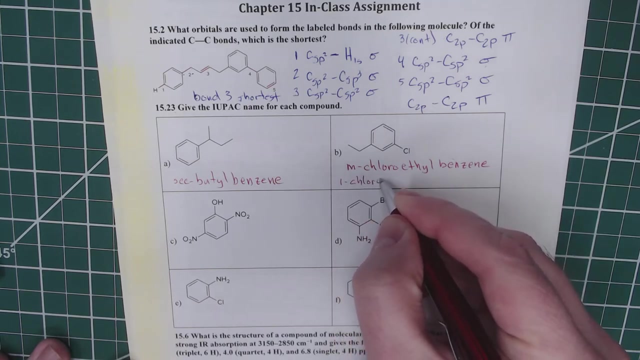 chloro first, And so there's two ways that we can refer to this. We could refer to this as meta-chloro-ethyl-benzene, No spaces in there. Or we can refer to this as 1-chloro-3-ethyl-benzene. 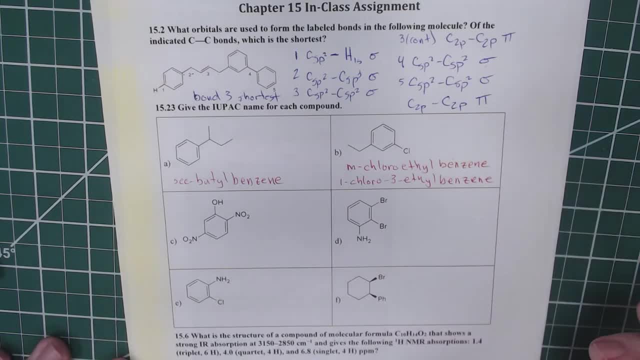 And that would be correct as well. So this would be the one position and the ethyl would be the three position. All right, On this one, we're going to name this with the root phenol. All right, So we'll call. 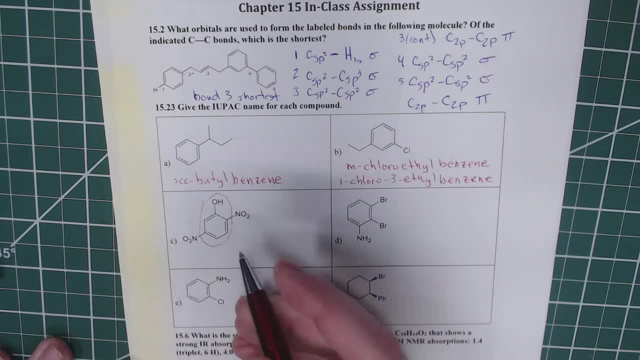 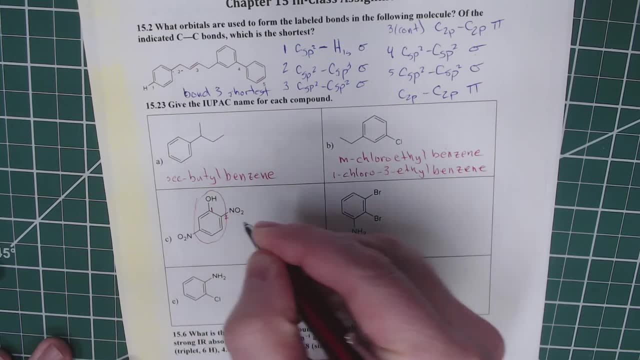 that one a phenol, And we have two nitros that are attached to the phenol. Since we're naming it a phenol, that's going to be carbon one And the next one. we want to have the lowest possible number, So that's two, And then, as we number around the ring, three, four, five, six, seven. 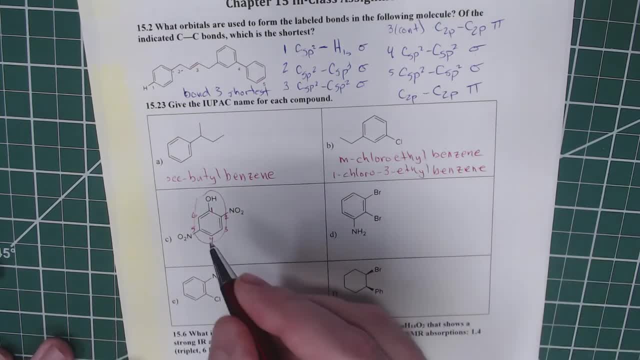 I can label it, But there's nothing on it. So we have two nitros that are attached to phenol, So this would be 2,5-dinitrophenol, So 2, 5-dinitrophenol, And again that phenol is its. 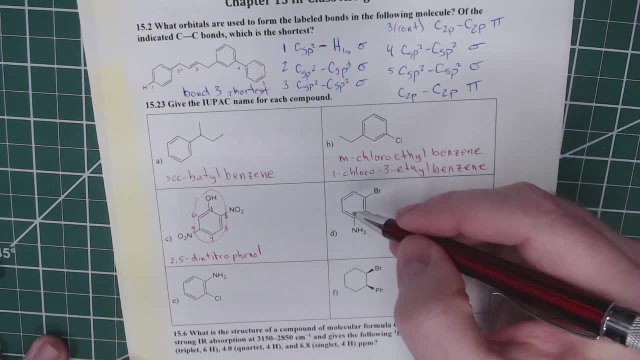 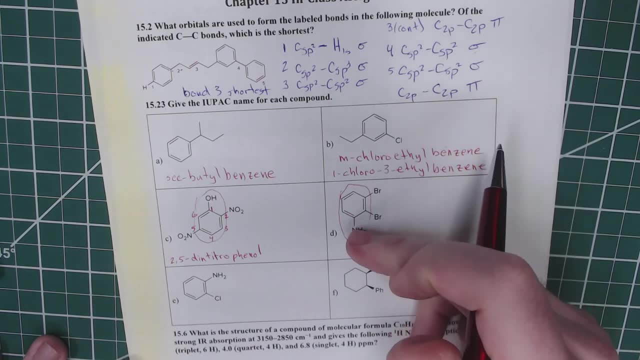 own unique functional group In a similar fashion. here we're going to name this after the common root, aniline, So that is aniline, and we have bromo at the 2 and 3 position. So 1, 2, 3.. 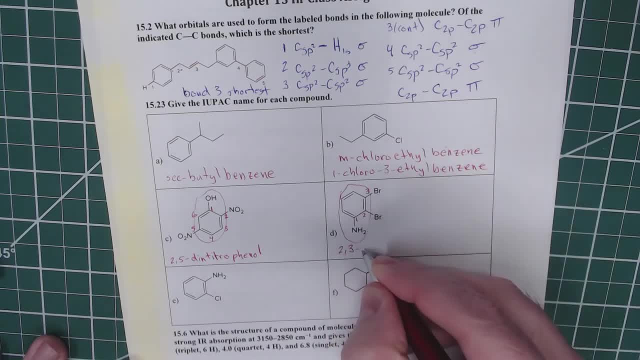 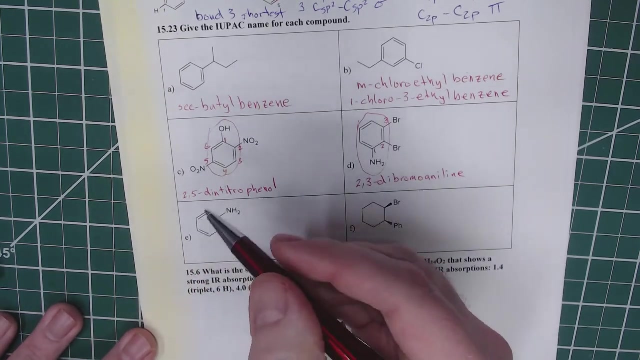 So this, we're going to name it as 2, 3-dibromoaniline, And that would be the name of that one. All right, and then finally, here this one also is an aniline. So this is our base group. 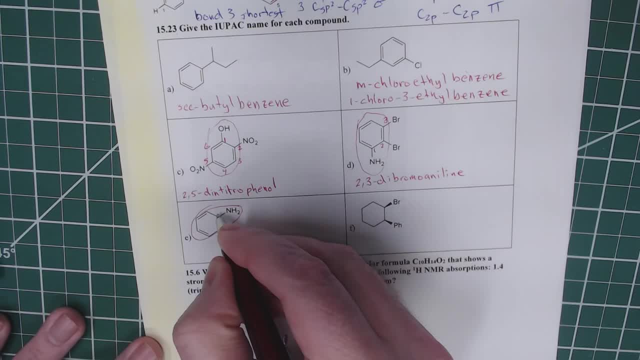 Since it's di-substituted, there's two ways to name this, But because we're going to name it after that root, we're going to call that one 1 and that one 2.. So this could either be ortho-chloroaniline. 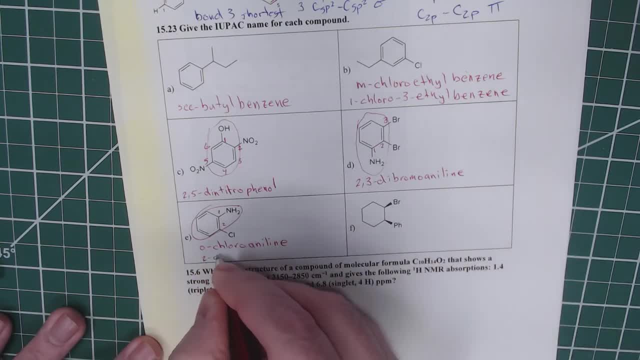 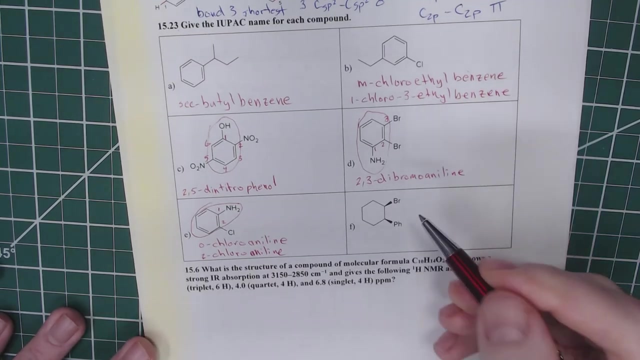 Or, if we wanted to use the number, we could just call it 2.. 2-chloro-aniline, So 2-chloro-aniline, And then finally, here we've got an example where we have a phenyl as a substituent. 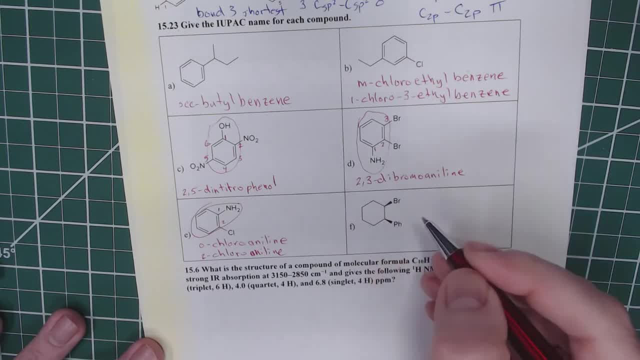 So our parent is going to be cyclohexane, We have a bromo and a phenyl. Bromo is going to come first, alphabetically, Alphabetically, So we're going to call this 1 and 2.. All right, and if we look at the stereochemistry, they are cis to each other. 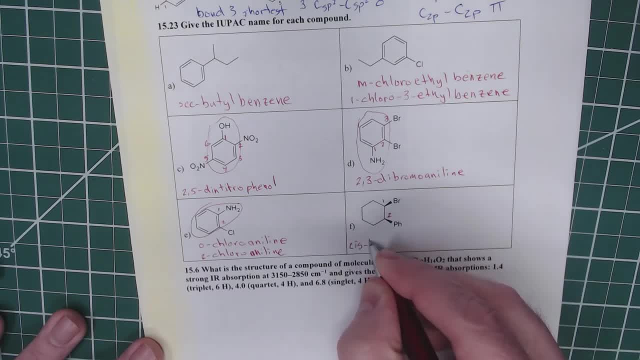 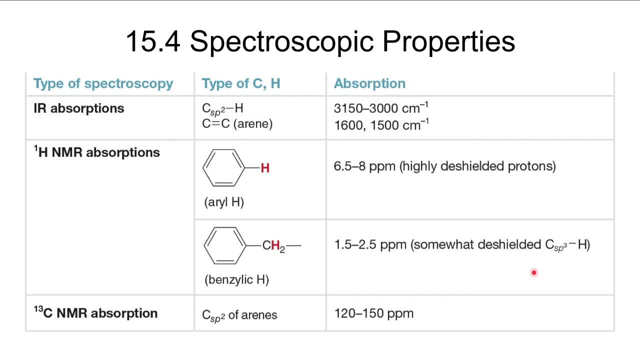 We're going to talk briefly about spectroscopic properties. We've talked about spectroscopic properties before, When we did the chapter on mass spec. we talked about that in spectroscopy A. In spectroscopy B we talked about IR And in spectroscopy C we talked about NMR. 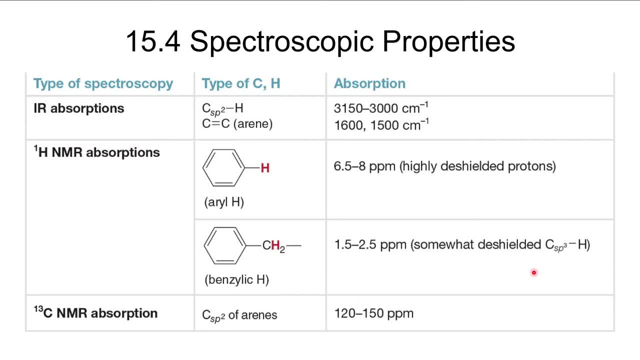 Just as a reminder, these are the things that are relevant for aromatic compounds, So remember where the carbon-hydrogen stretching is for carbon SP2.. It comes out between 3150 and 3000 reciprocal centimeters. So that one is one that you know. 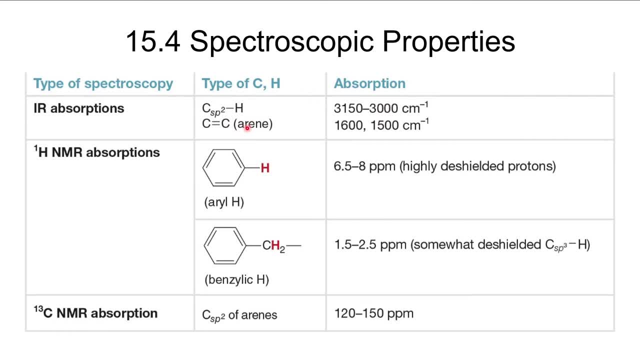 And then we have two absorptions that are associated. They're associated with benzene rings, with phenyl rings, areal rings, arene, however you want to call it, And those are two peaks that are at 16 and 1500 reciprocal centimeters. 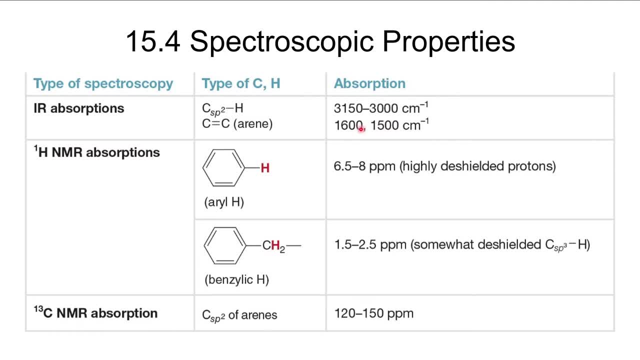 Remember that these numbers can be within about 15 or 20 of that number and still be valid. It just depends on what's attached to it that will affect where they are. For proton NMR are areal hydrogens, The hydrogens that are directly connected. 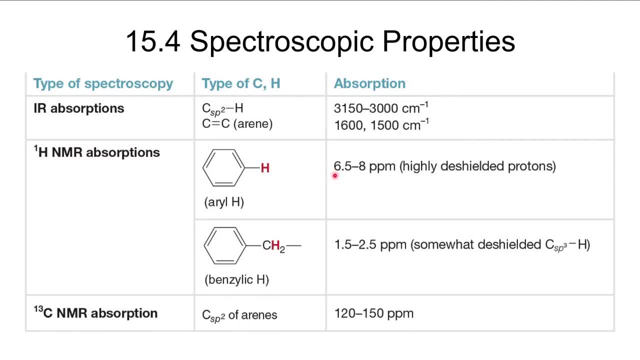 Directly connected to the benzene ring are going to have absorptions out at 6.5 to 8. They're highly deshielded protons, So, and that's because of the aromatic ring, So 6.5 to 8 parts per million. 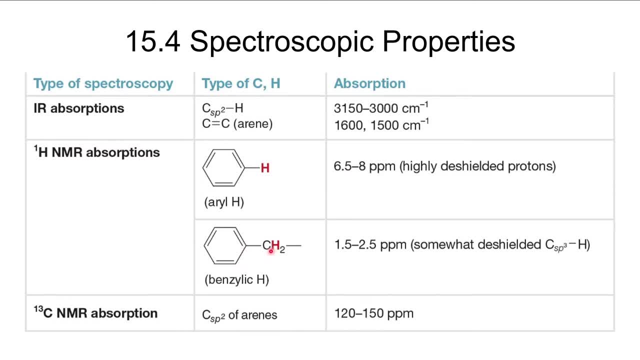 And for the benzyl, this is kind of like the allylic ones, where the hydrogen is going to show up in the 1.5 to 2.5 part per million range, Not deshielded, compared to other carbon, sp3, hybridized carbons with a hydrogen on them. 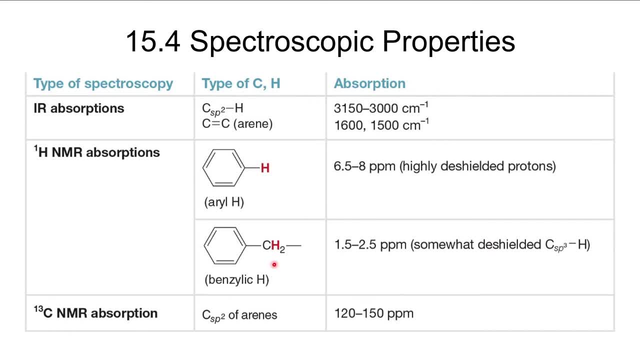 So benzylic 1.5 to 2.5.. You'll want to know that For the carbon NMR, we're going to find that they all fall in a range from 120 to 150 parts per million. Remember, for carbon NMR our range is total. range is from zero out to about 220, and this 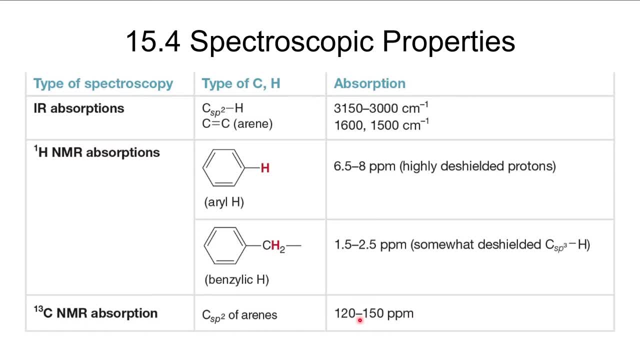 falls in that relatively narrow range: 120 to 150.. What's attached to it will affect these numbers. If you have something very electron withdrawing, it will pull this, it will pull it downfield, And if you have something that's electron donating, it will pull it upfield. 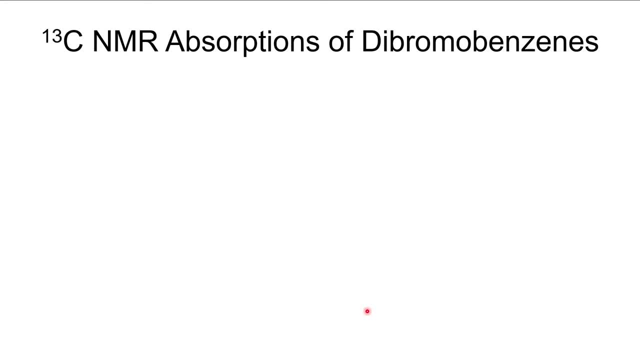 All right. Now there is something that's very interesting that you can. You can determine When you have disubstituted. when you have two of the same substituent on a benzene ring with carbon NMR, you can determine what the substitution pattern is. 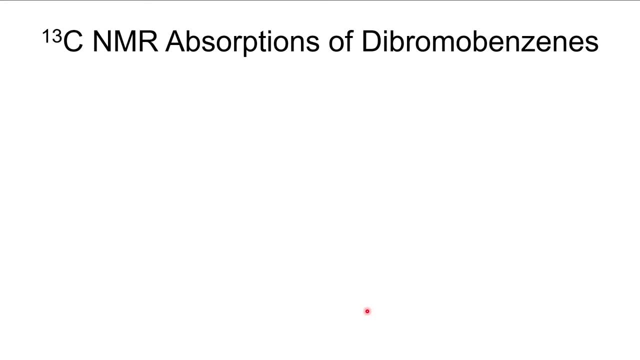 So if you have dibromobenzene, ortho, meta and para, you're going to get a different number of carbons depending on what the substitution pattern is. So the number of lines: remember, they show up essentially as singlets, as lines in the 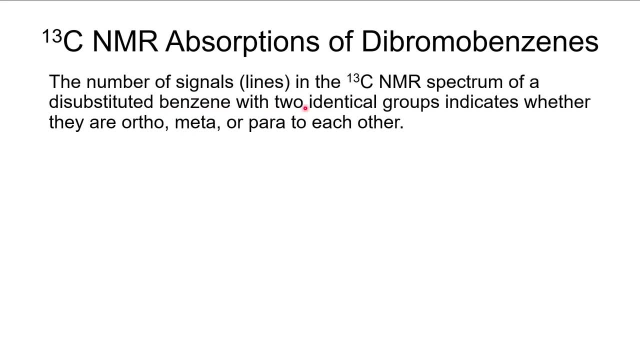 carbon NMR spectrum. So the number of lines will be. when you have two identical groups, it all depends on whether it's ortho, meta or para. So if you've got the ortho dibromobenzene, there are three different types of carbon. 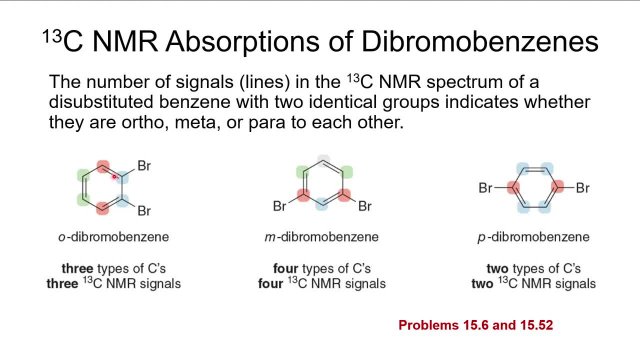 So the two carbons that have the bromine are identical. These two carbons that are adjacent are also identical, And these two carbons are identical. Remember, if you can put a plane of symmetry through it, like you do with this one, then 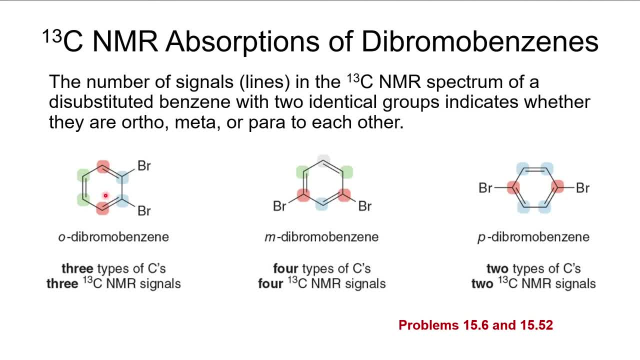 that means the things that are opposite each other are identical. With the meta dibromobenzene we'll find that again the two carbons bearing the bromines are identical. These two carbons, the two green ones here, are identical. 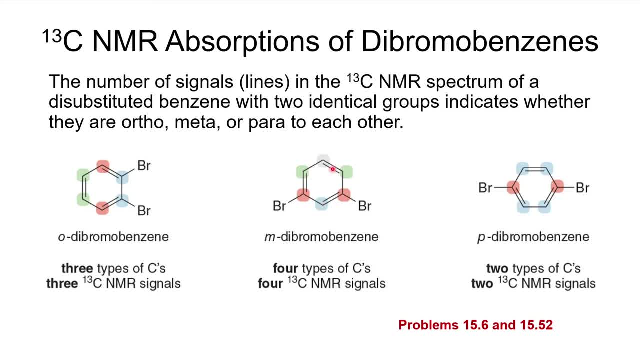 But then this carbon that's between the two bromines is unique, and this carbon out here that is furthest away from the two bromines is also unique. So there we get four carbon NMR signals With the para dibromobenzene. 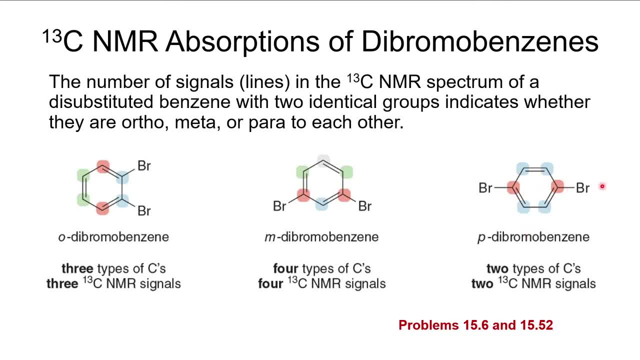 We have two planes of symmetry. We have one that goes right down the middle this way, and one that goes this way. So that means that these two are identical. these two are identical, but then these two are also identical to these two. 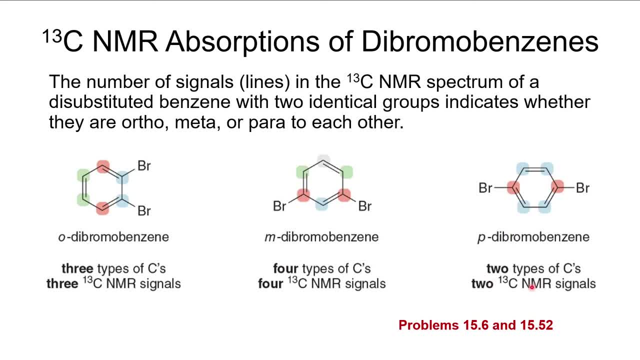 So we only have two types of carbons in the signal. At some point you can do this now and pause the video, or you can think about this a little bit later, But at some point I want you to think about what happens if I have two different substituents. 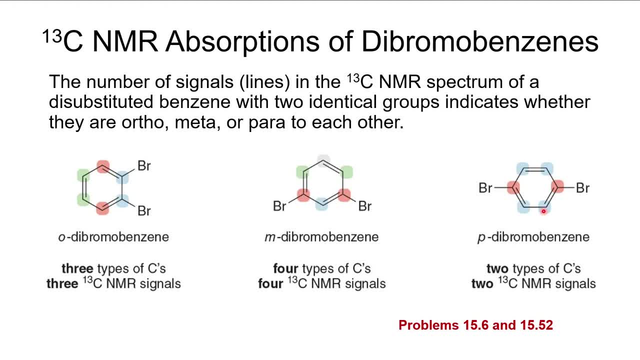 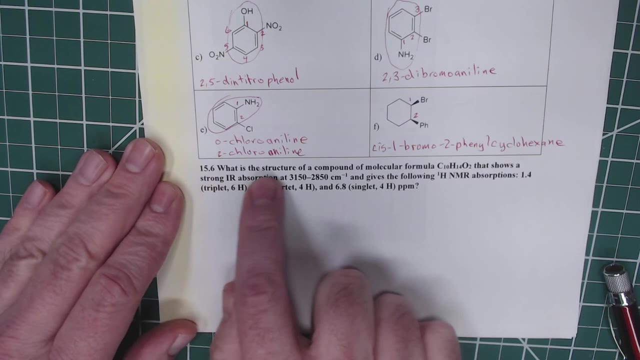 How many peaks? How many peaks would I get for each of these? And you might be surprised at the answer. But for now we're going to go over to number six and number 52 on the in-class assignment. So on number six, it says: what is the structure of a compound molecular formula C10H14O2?? 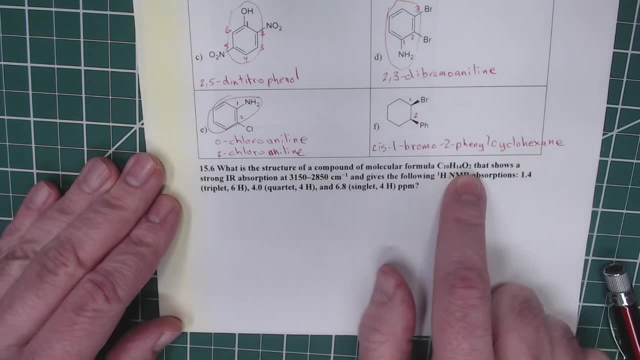 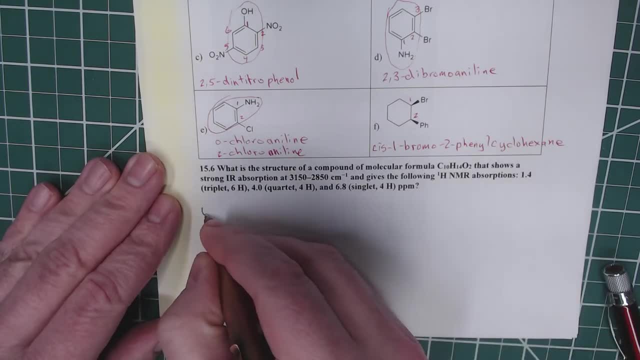 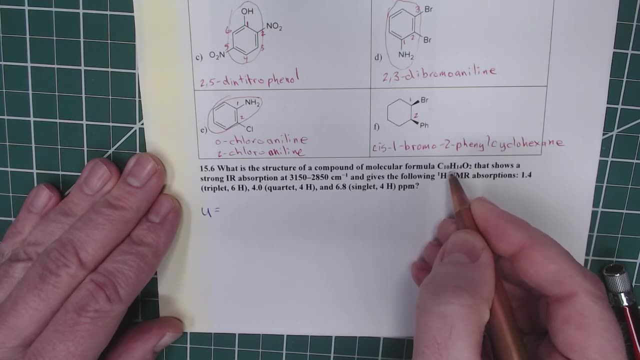 to calculate the degree of unsaturation. So the degree of unsaturation is going to be the maximum number of hydrogens with 10.. Ten times two is 20, plus two is 22.. We're going to subtract the actual number of hydrogens, which in this case is 14, and 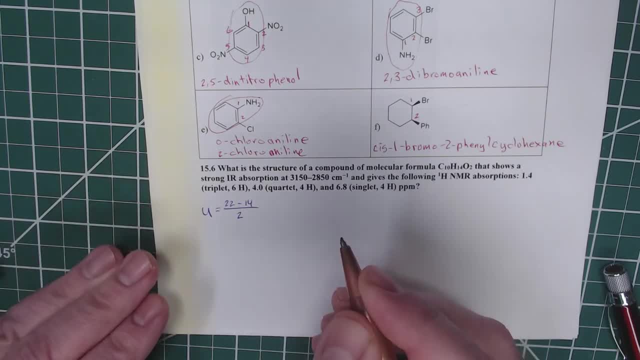 then we'll divide by 14.. We're going to divide by 2.. And when we divide by 2, that'll be 8 divided by 2.. That gives us 4.. So there are 4 degrees of unsaturation. 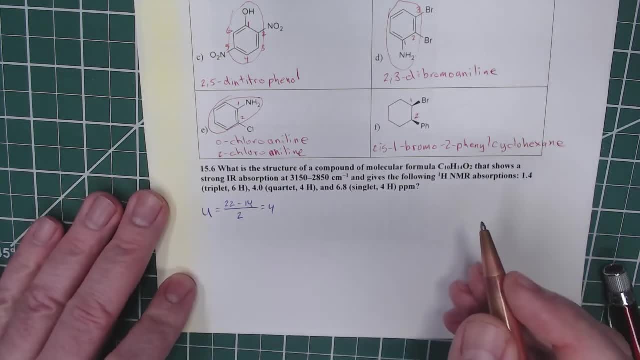 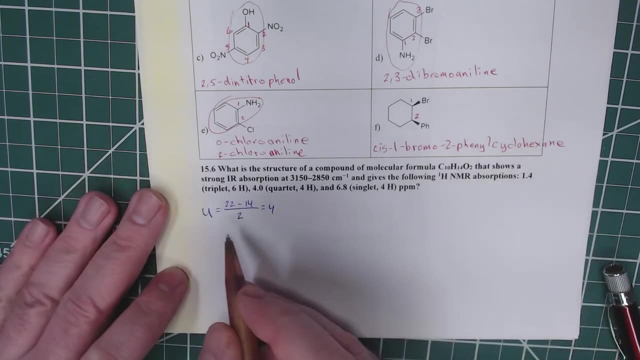 Because this is a chapter on aromatic rings, that's not very surprising. That means that we have a benzene ring. Benzene ring in and of itself has 4 degrees of unsaturation. That would account for it. That means that we also have no additional unsaturation. 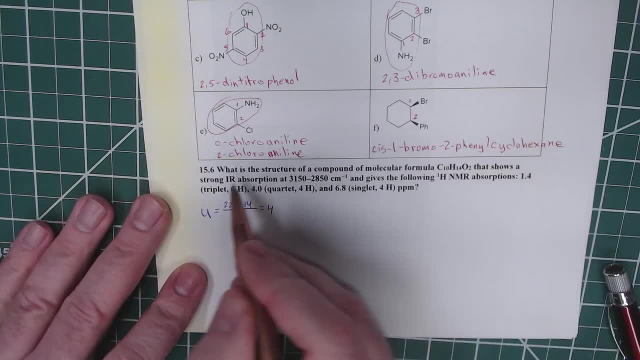 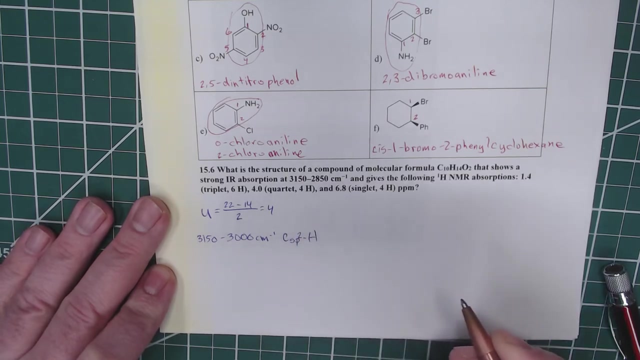 So we have no additional double bonds. It shows a strong IR absorption: 3,150 to 2,850.. And so that covers both of our carbon hydrogen. So the 3,150 to 3,000 reciprocal centimeters, that's what corresponds to the carbon sp2. 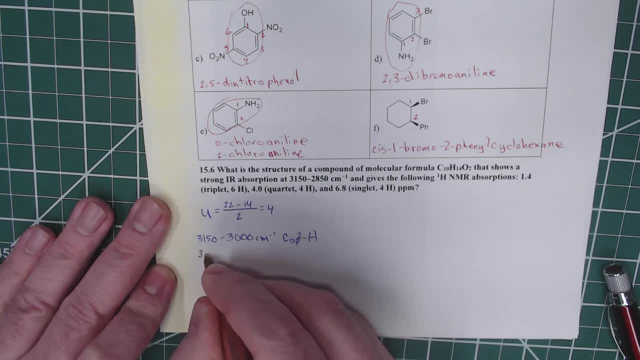 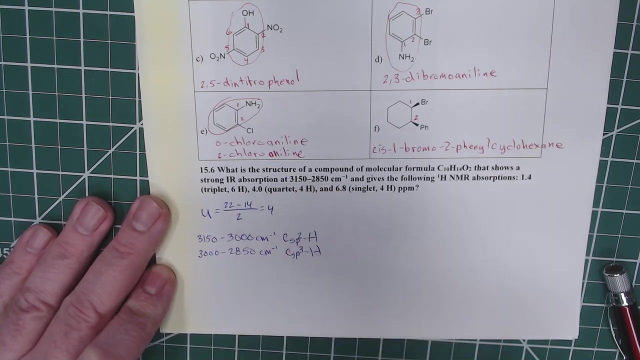 hydrogen stretch, And then the 3,000 down to 3,000.. And then the 3,000 down to 2,850 reciprocal centimeters. that's the carbon sp3 hydrogen. So when you see it stretch across both of those ranges, that tells us we have both types. 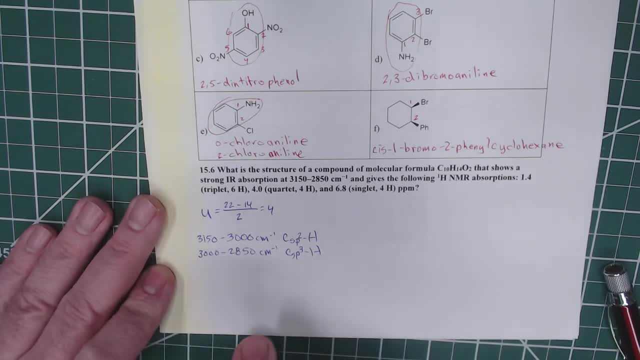 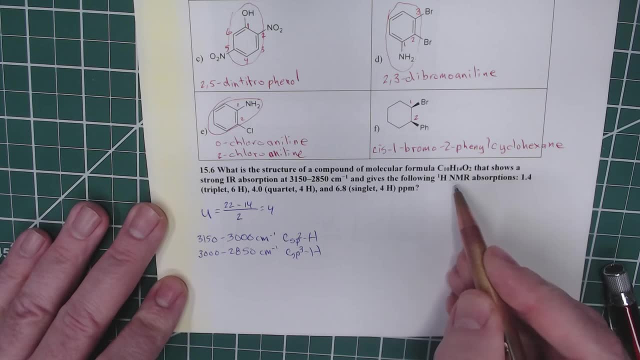 of carbon hydrogen, stretching both sp2 and sp3.. That gives us structural information. Now let's look at the rest. All right, And it gives the following: proton, NMR, absorptions 1.4, you've got a triplet and it's 6 hydrogens. 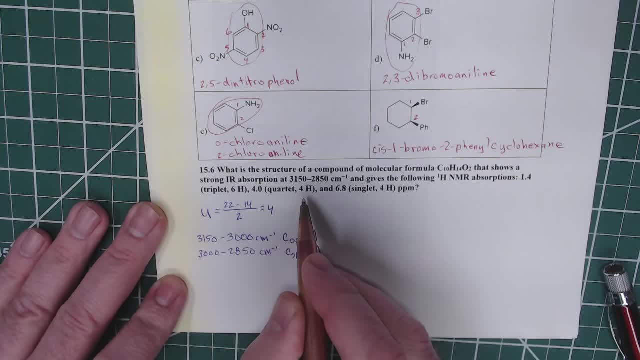 4.0, we've got a quartet and it's 4 hydrogens. Well, if we look at those, whenever we have that triplet quartet pattern and look over here, we've got a singlet that's 4 hydrogens and it's at 6.8.. 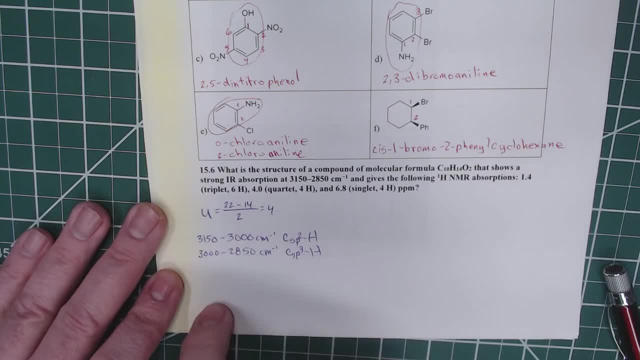 We'll talk about that one in a minute. But for this, when we have that triplet quartet pattern, that is an ethyl pattern And it matches The numbers match here. So we've got 6 hydrogens that are the triplet and we've got 4 hydrogens that are the quartet. 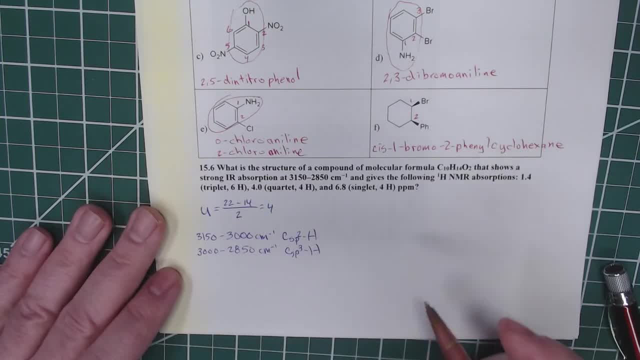 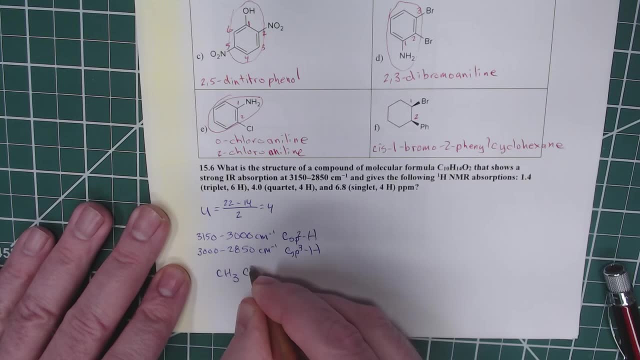 That's a 3 to 2 ratio, as we would see with an ethyl group. All right, So we've got the CH3, CH2, that's a 2 there, not a 3. And it's attached to something. 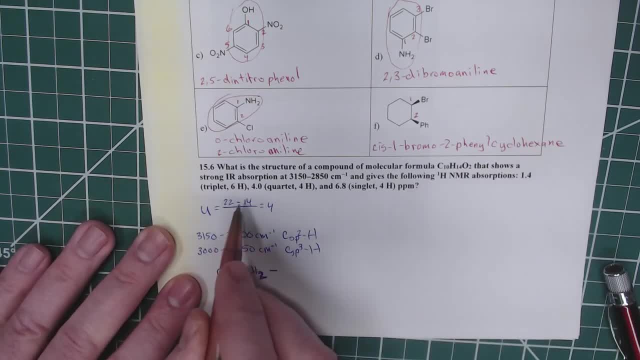 And this corresponds. all right. so this corresponds to the triplet, the 6 hydrogens. There's 2 of the ethyl group, All right, There's 2 of the ethyls that are identical, And then the quartet is going to correspond to this. 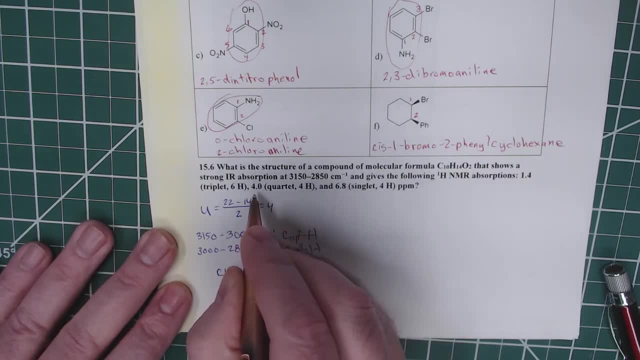 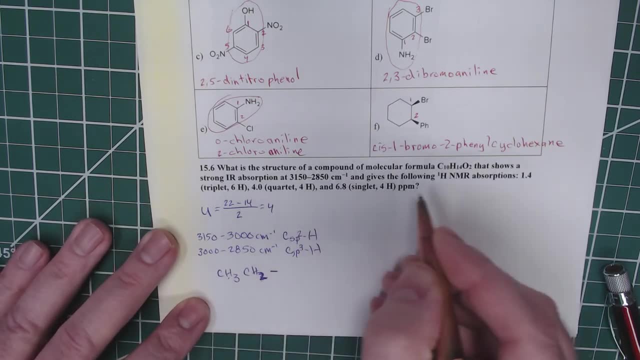 Because that quartet, the 4 hydrogens, is at 4.0, that tells us that those hydrogens must be adjacent to something that's very electronegative And, given that we have oxygen in the compound, we probably have an oxygen directly adjacent. 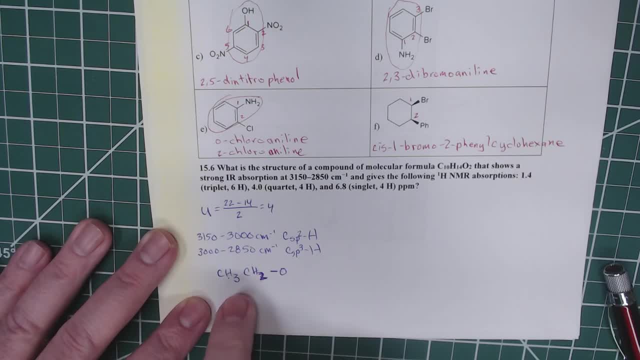 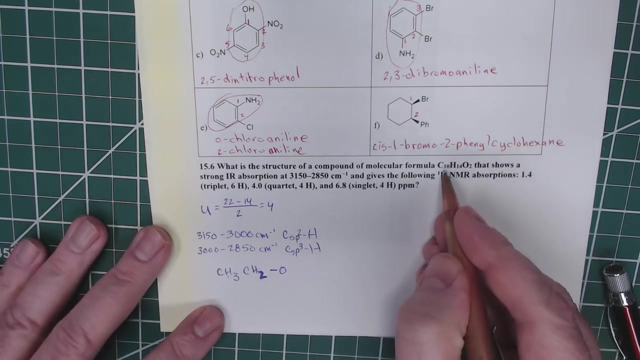 to those 2 hydrogens. But we've got 2 ethoxy groups that are attached to a benzene and that these 2 ethoxy groups are identical. All right, If we look, that accounts for everything right. We have 6 carbons in the ring and we've got 2 of these ethoxy groups that are identical. 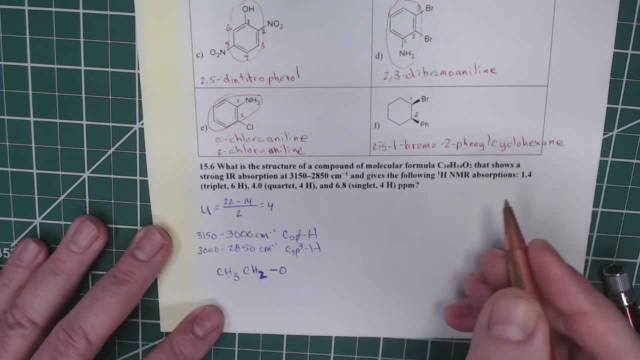 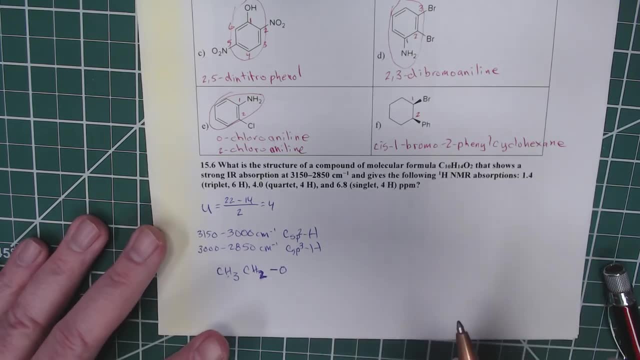 That would give us the other carbons and the hydrogens. Since we have 2 substituents, it makes sense that we have 4 hydrogens and so, really, this gives us. It gives us Just with that information, it gives us 3 possibilities. 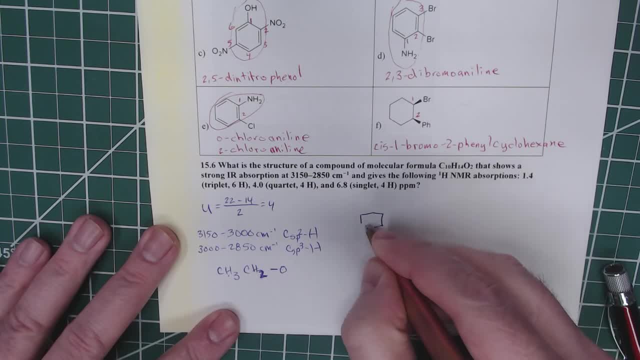 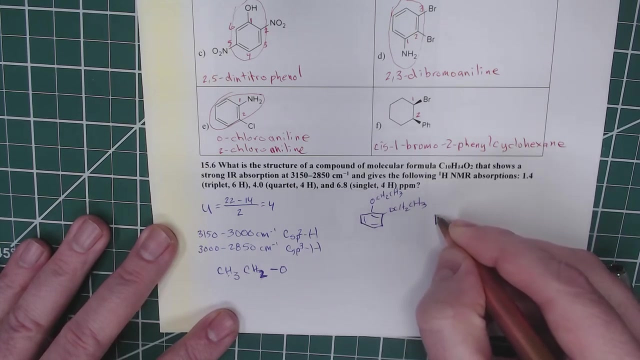 And the 3 possibilities are where we've got the benzene ring and we could have ortho, so CH2CH3, OCH2CH3, so that would be one possibility. Another would be where we have meta, All right. 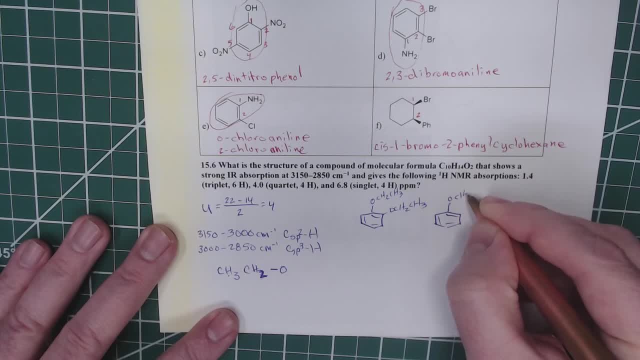 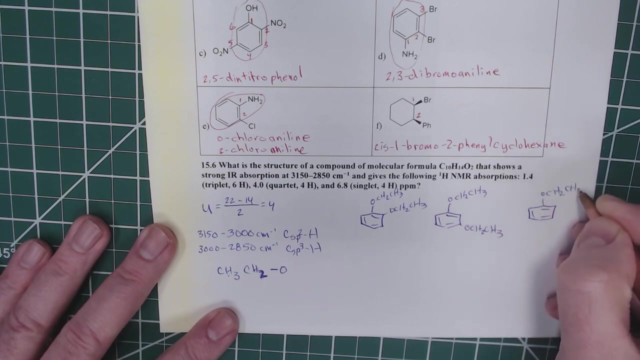 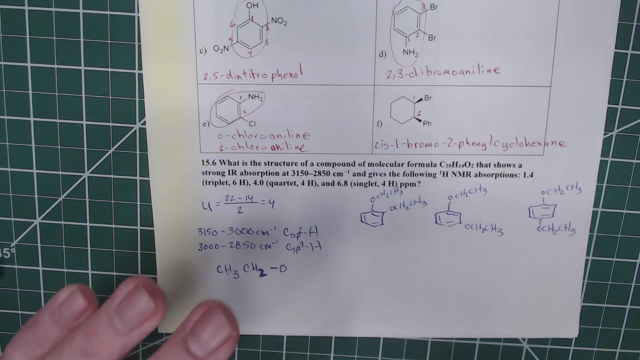 And so OCH2CH3.. All right, All right, All right. So OCH2CH3, OCH2CH3.. And then, finally, our final option would be where we have para OCH2CH3.. Now we can determine which one of these it is by looking at this thing. 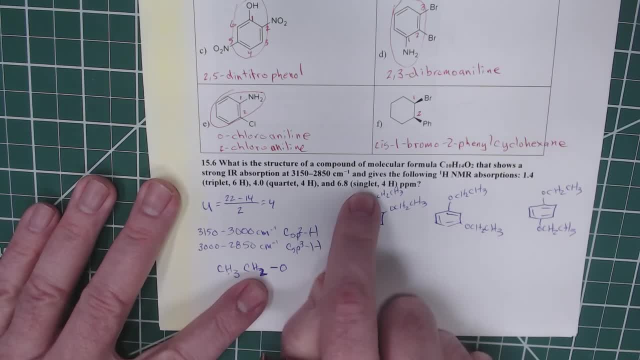 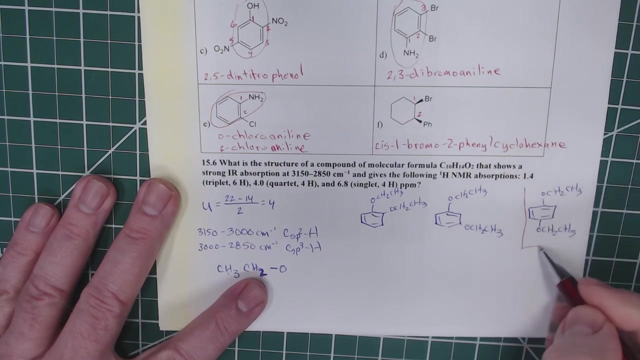 This particular one. it says we have a singlet, And for it to be a singlet, that means that all four hydrogens need to be identical. And that is only the case in this structure, where it is para. So, because it's a singlet, that tells us that all four hydrogens on the benzene ring are identical. 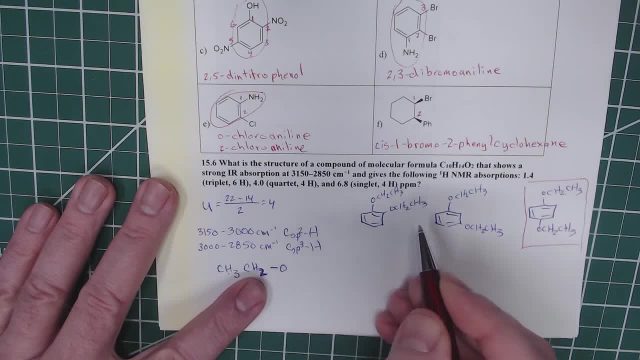 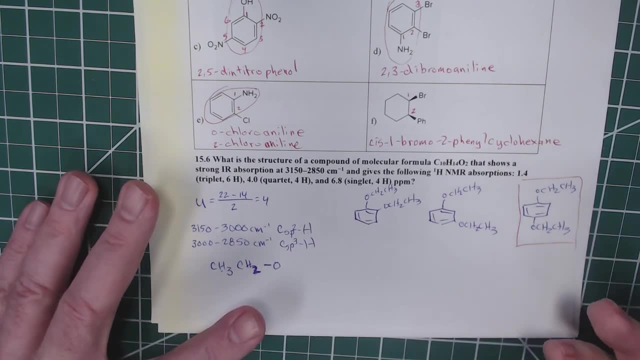 If we had this one, we would have a doublet of doublets, So we would have an interesting structure there. So this would be coupled to this and that would look different. If we had this one, we would have coupling between this and this. 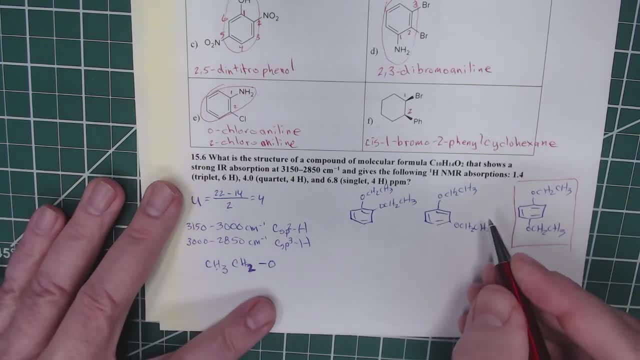 and we might get some cross-coupling weird stuff that happens in a benzene ring, but it would be a more complex pattern. With this, this is the only one that would give us a singlet, because all four hydrogens are identical. 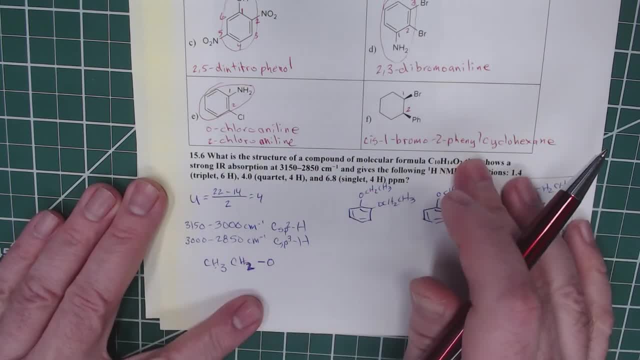 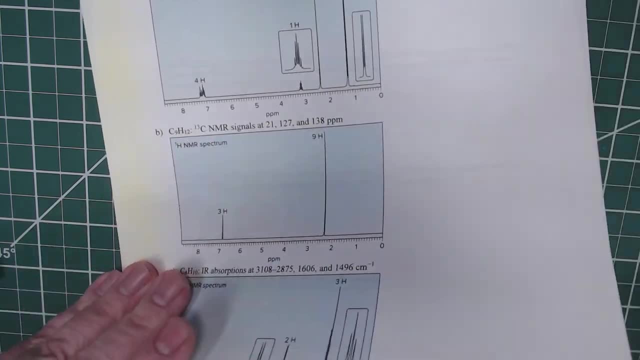 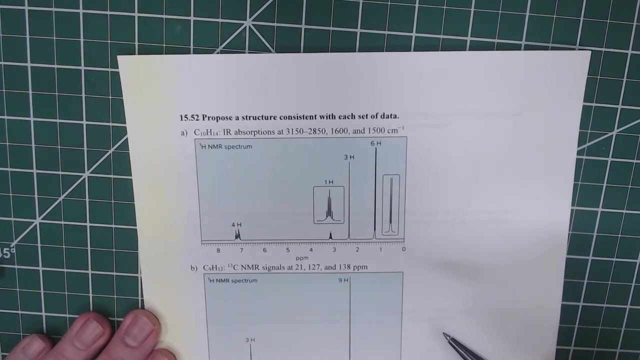 So this structure is consistent with all the information that we have there. So we're going to also look at number 52, and number 52 actually has three problems on it. We want to propose a structure that's consistent with each of these. 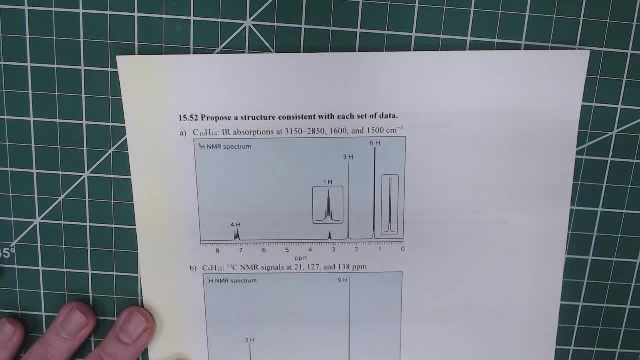 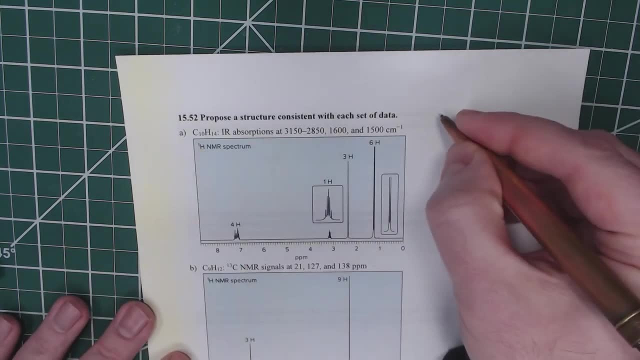 The very first thing I'm going to do on each of these is to determine the degree of unsaturation On all of them. we're going to find the degree of unsaturation is four, but we'll go ahead and calculate it. 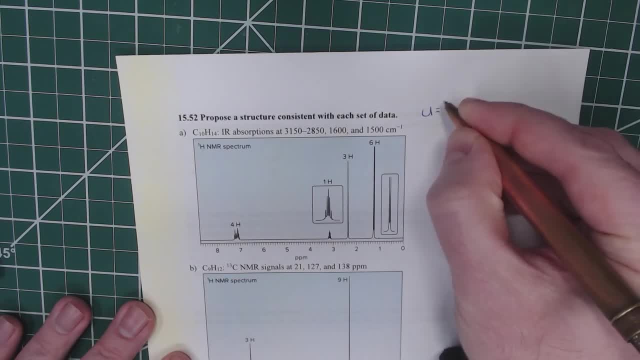 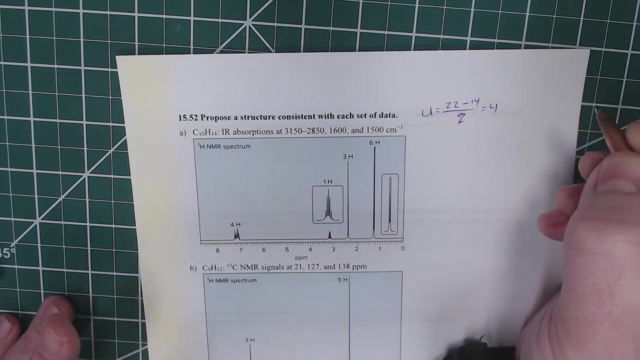 So our degree of unsaturation, Our degree of unsaturation is equal to. So 10 times 2 is 20, plus 2 is 22.. We're going to subtract 14 and divide by 2, and that gives us four degrees of unsaturation. 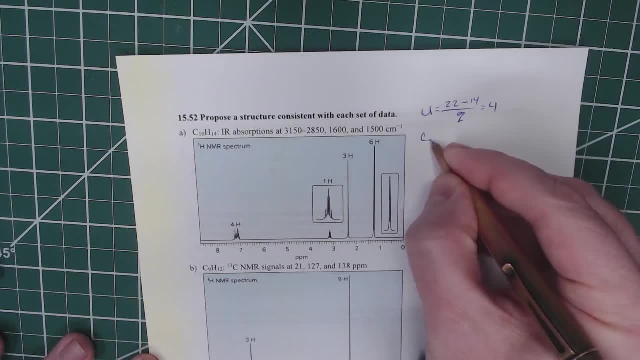 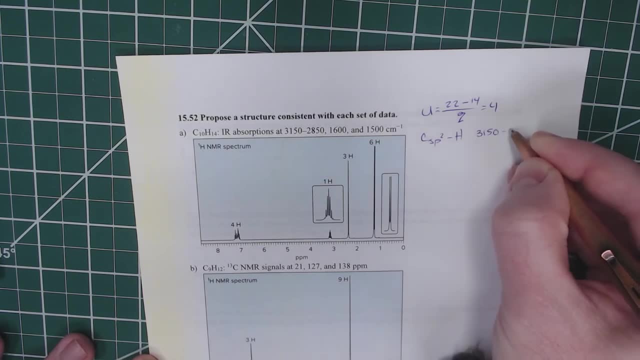 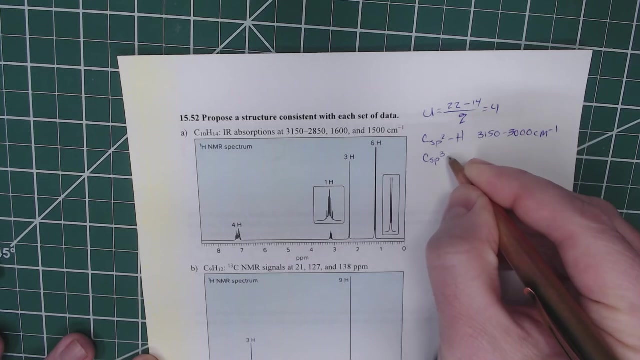 All right. so we have carbon SP2 hydrogen stretching, That is the 3150 to 3000 reciprocal centimeters, And we've got carbon SP3 hydrogen stretching, and that's the one that's from 3000 to 2850.. 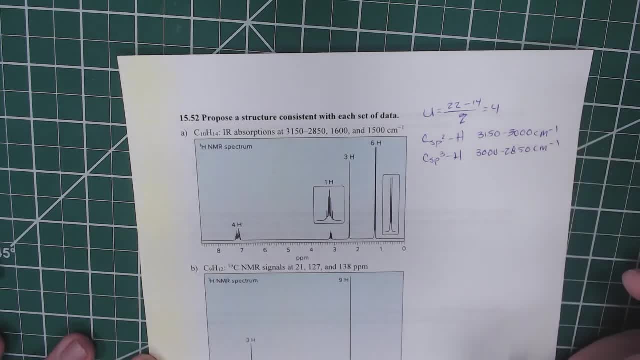 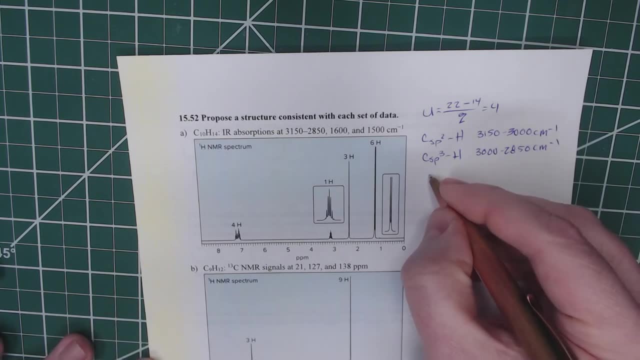 Okay, And we've got carbon, SP3, hydrogen stretching and that's the one. that's from 3000 to 2850.. All right, The 1600 and the 1500, that is typical that we have a benzene ring. 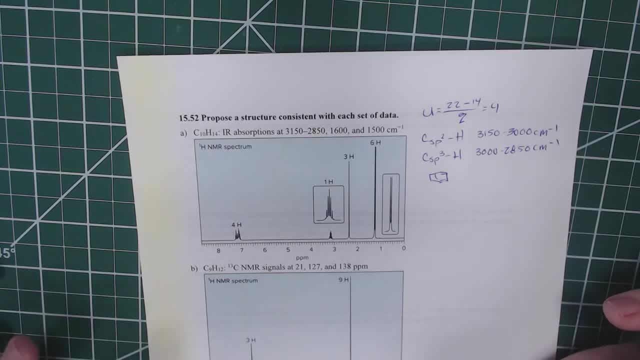 Not surprising, since this is a whole chapter about benzene rings. Now we need to deal with the substituents. We have four carbons, All right. We've got four carbons that are substituents, All right. So we need to look at these. 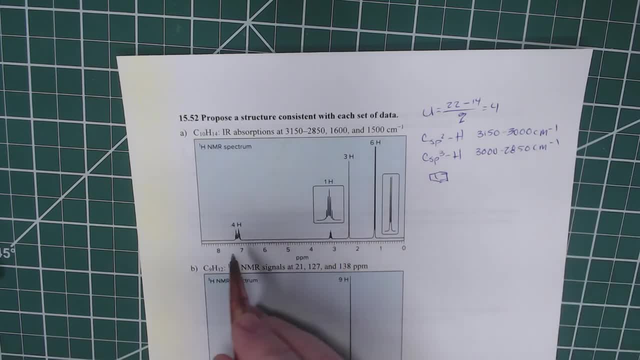 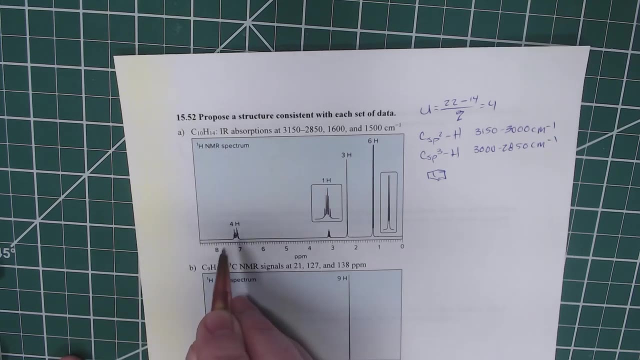 We need to look at these disorbances in the NMR. First of all, let's notice that out here in the aerial hydrogen range we only have four hydrogens and it is a multiplant With the four hydrogens we will find that means that we have two substituents. 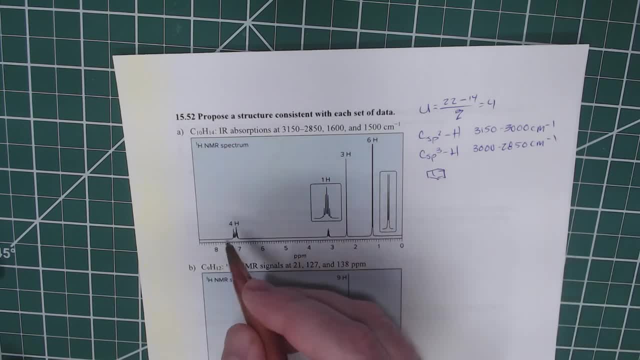 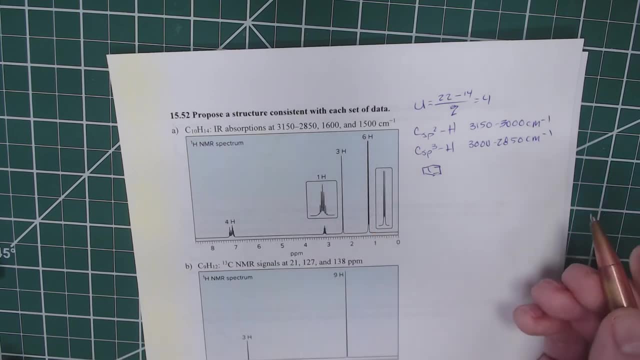 We've got two different substituents here, All right. When we look over here, we've got a singlet that's three hydrogens. The singlet that's three hydrogens, all right, so it's at about 2.4, we'll call it parts per million. 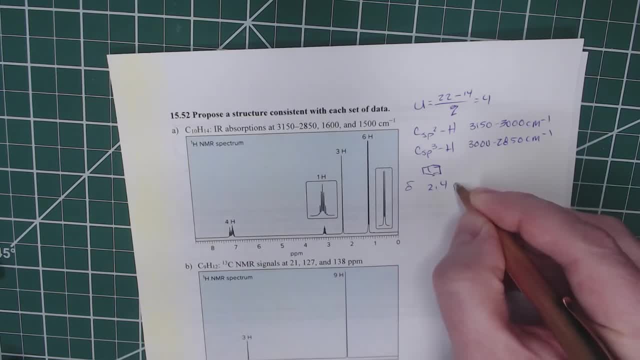 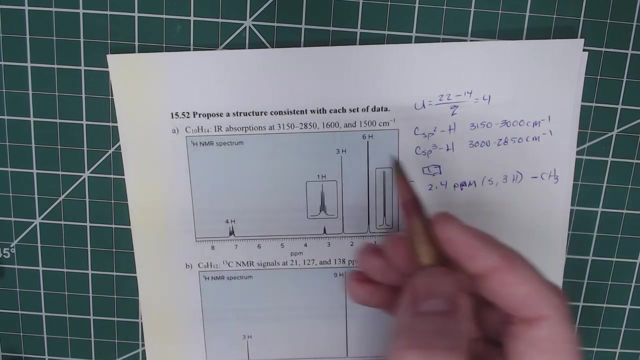 So delta is 2.4 parts per million, All right, And it is a singlet and it integrates for three hydrogens. That's almost certainly a methyl group, All right, And we don't have any oxygens on here. 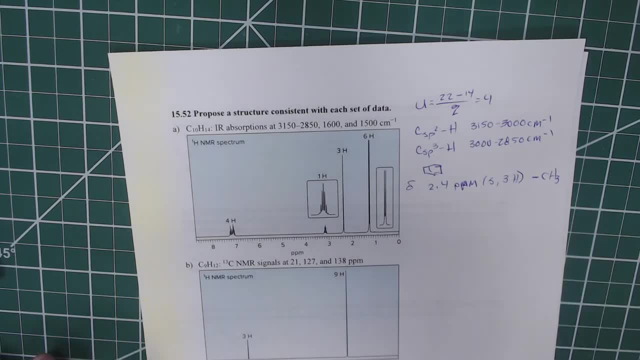 So it looks like that methyl group is directly attached to the benzene ring. If you go back and look at the absorbances that we have the proton NMR absorbance for a benzyl hydrogen, that fits With that at about 2.4, that's in the 1.5 to 2.5 range. that fits. 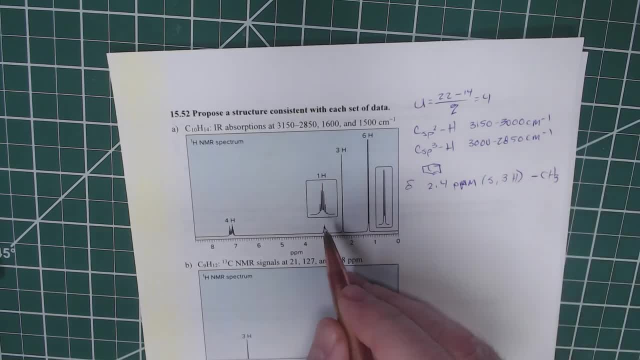 So it looks like we have a methyl. Okay, The other substituent has one hydrogen and six hydrogens, So that looks like a propyl group of some sort And if we look carefully, we've got a. this. it's hard to see, but this is a septet. 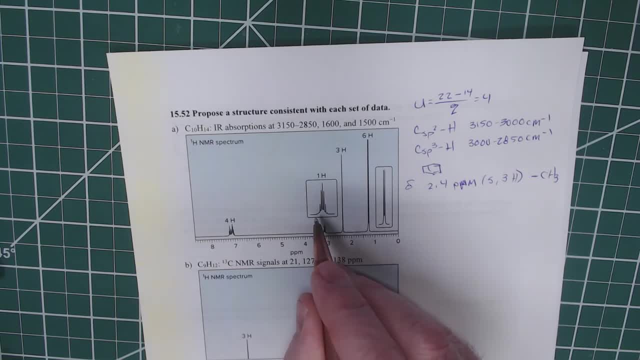 It looks like a. it looks like a quintet because it looks like there's five, but there's actually one that's kind of buried on the sides. It's a multiplet and it's coupled to this one, which is a doublet. 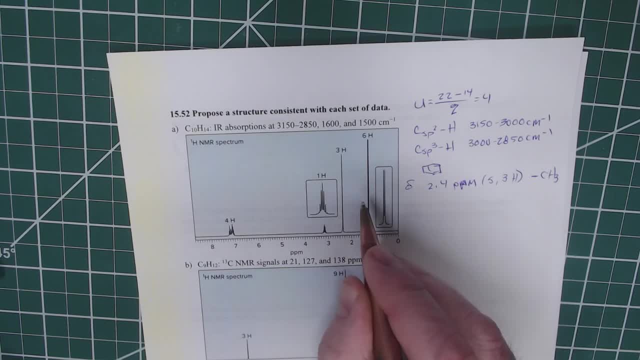 So we've got one hydrogen, that is a septet, And six hydrogens, that is a monosubstituent. All right, that's a doublet. That is a pattern that we see with isopropyl. So our our absorbance. 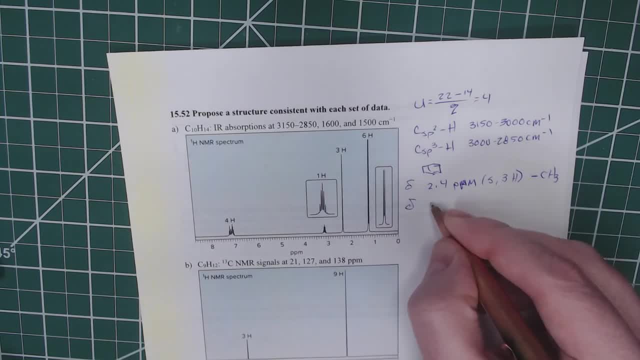 that is the let's see. one point looks like about 1.3 parts per million. All right, It's a doublet and it accounts for six hydrogens. All right, And so that those are two CH3s. 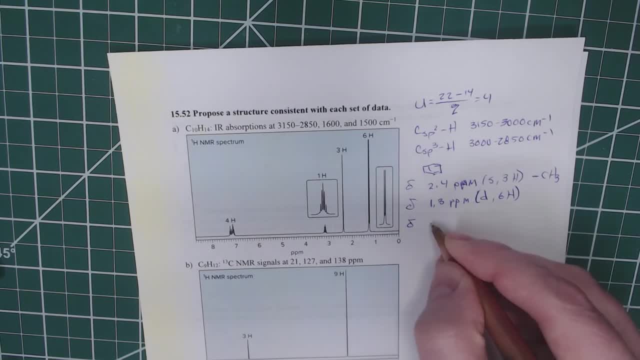 and then here we've got again at three. point looks about 3.1 or 3.2.. We're just going to call it 3.2 parts per million. We've got a septet and it accounts for one hydrogen. Again, these together. 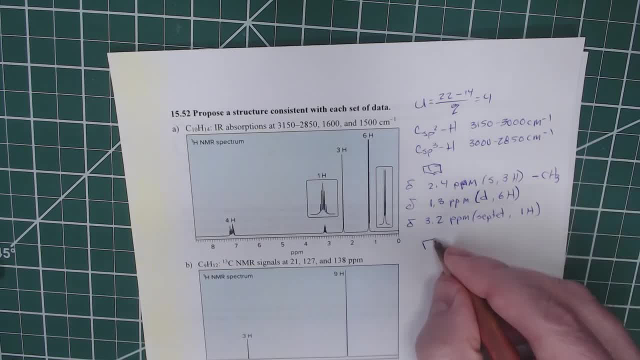 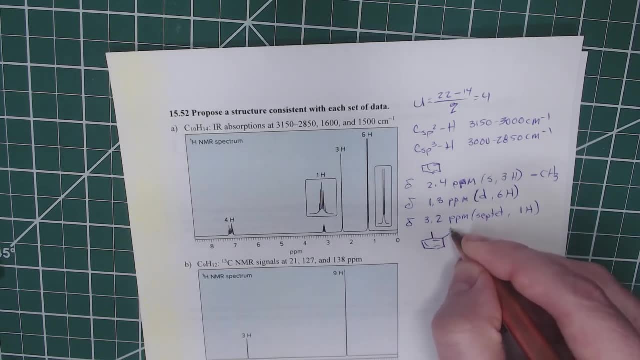 is an isopropyl group. So we've got two possibilities here. Technically we have three, but one we can kind of rule out. So we could have the methyl there and an isopropyl there, All right, And that. 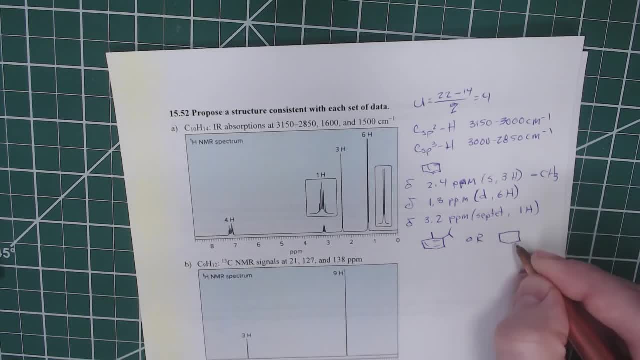 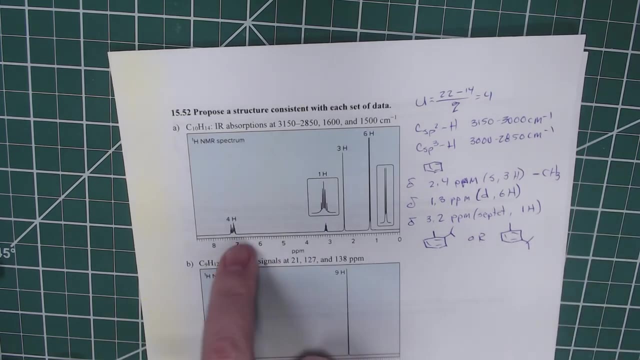 would be the ortho, or we could have a methyl there and an isopropyl there. The reason I didn't draw the para: if we had the para substituent, these couplings would be, it would be, it would be a doublet of doublets When we have two different substituents on a benzene ring and they 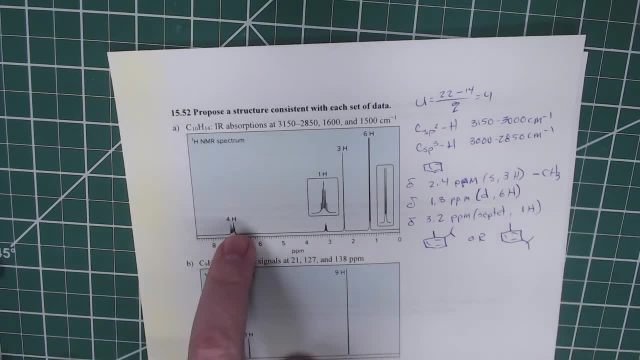 are para to each other, we get a doublet, of doublets. It looks a little bit more regular And in this case it's going to be one of these two. With the information that's supplied. I don't know that we could figure that out. We would have to do some additional experiments to 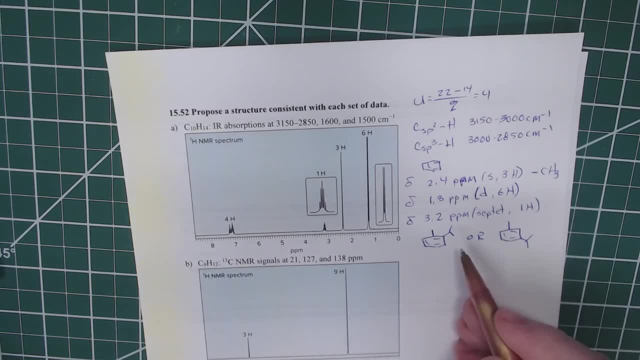 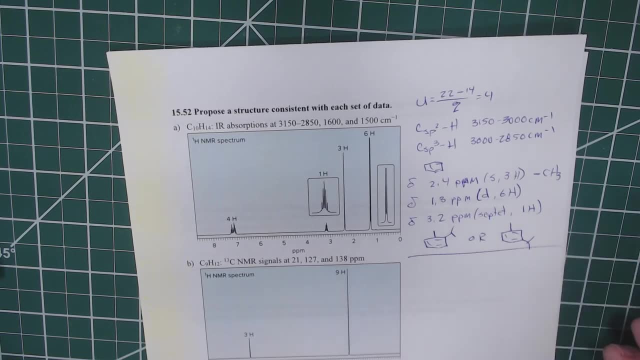 figure that out. But if we can narrow it down to two, that's usually a pretty good, a pretty good job, All right. So one of those is going to be our structure. So now let's look at this one: our degree of. 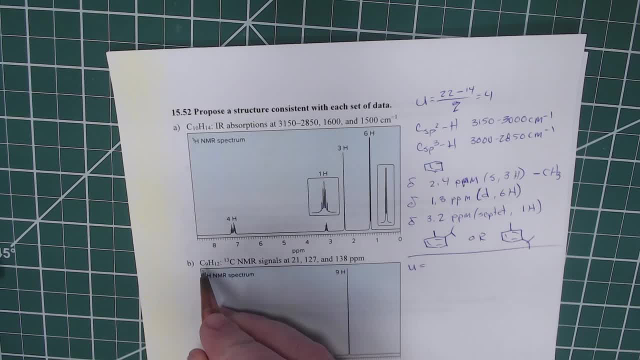 unsaturation. So nine times two is 18 plus two is 20.. So 20 minus 12 over two again gives us four degrees of unsaturation With four degrees of unsaturation, with four degrees of unsaturation. 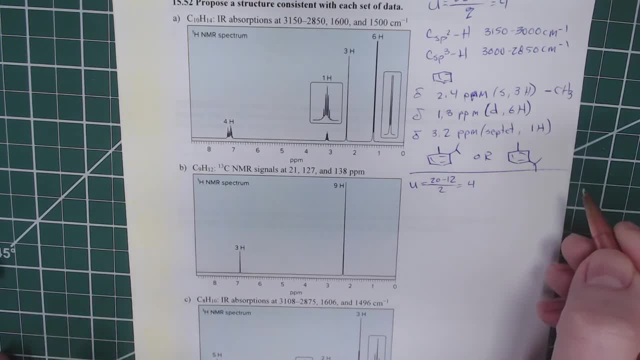 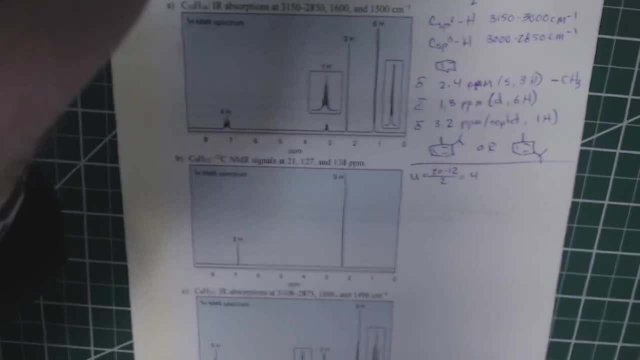 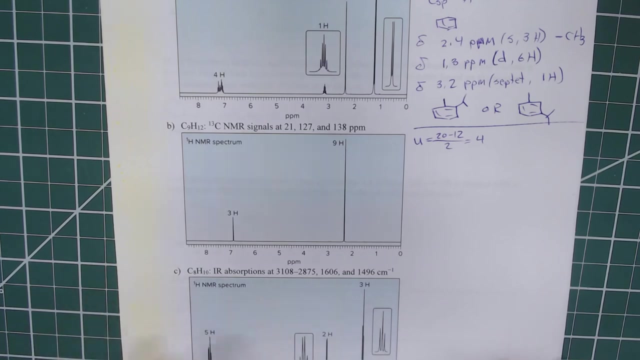 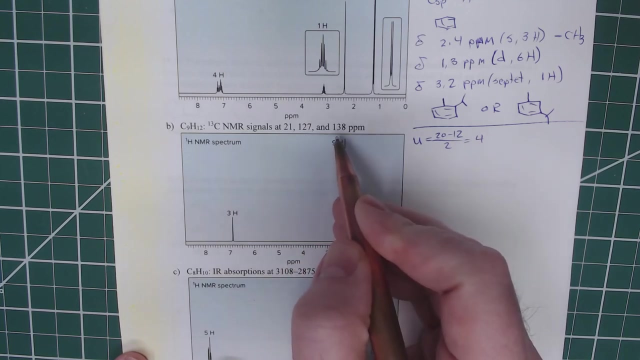 then that tells us that we have a benzene ring and no other double bonds, so no other unsaturations. All right, I'm going to pull this down a little bit. Okay, We've got a carbon NMR signal at 21,, 127, and 138.. That tells us that we've got. 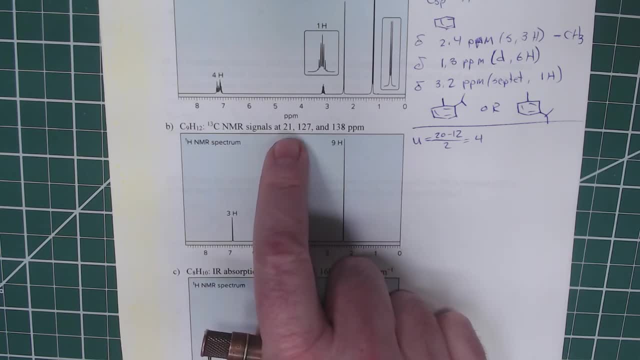 uh, we've got that tells us that we've got a signal, a carbon that is an sp3 hybridized carbon, but there's only one carbon in there. So we've got a carbon NMR signal at 21,, 127, and 138.. 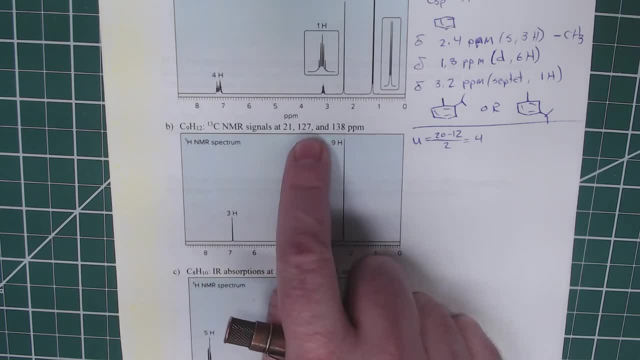 There's only one type of that and that we've got two aromatic carbons, All right. So there's only two peaks, two different types of peaks, in our, our aromatic ring. If we look where the aromatic ring is, we have a singlet and it's three hydrogens, So we have a tri-substituted. 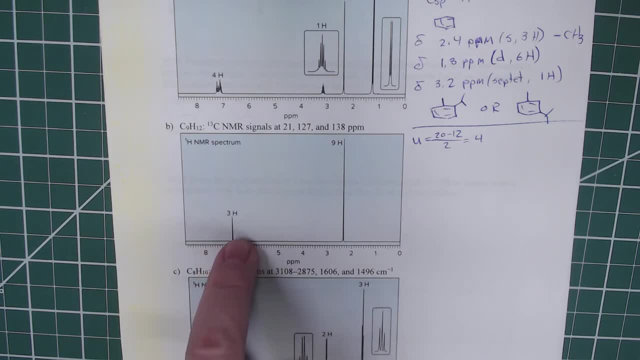 benzene ring, and all three hydrogens on the benzene ring are identical. In addition to that, we've got nine hydrogens in this singlet That's at about two point something, And that tells us that we've got nine hydrogens that are all identical. They're all identical, All right. 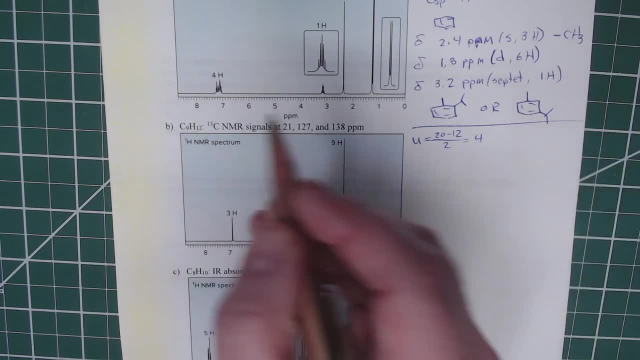 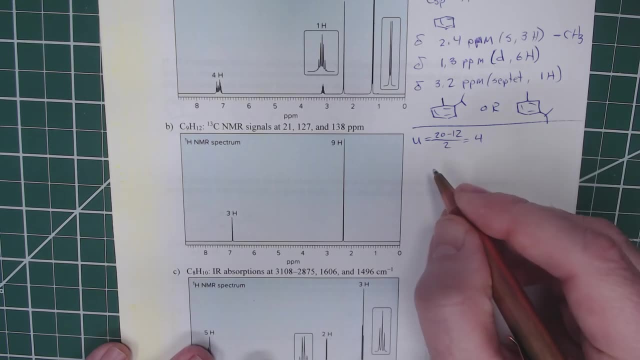 With the nine hydrogens. uh, uh. so six of the carbons are going to be in the ring with the nine hydrogens. that tells us that we probably have three methyl groups on a benzene ring. And if we look at the possibilities, 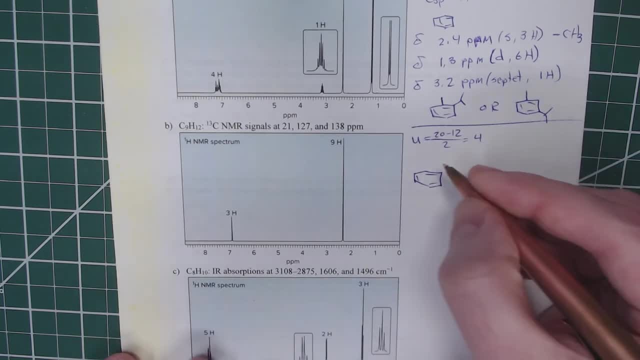 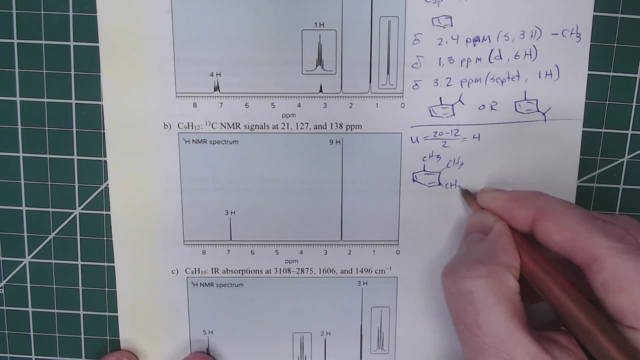 all right, we start to. we start to, uh, um, weed out some things pretty quickly. So CH3, CH3, CH3.. Well, this can't be it, uh, because, uh, these methyls are not identical. This one's identical. 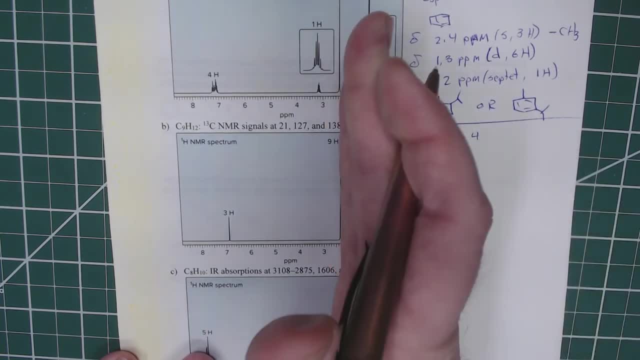 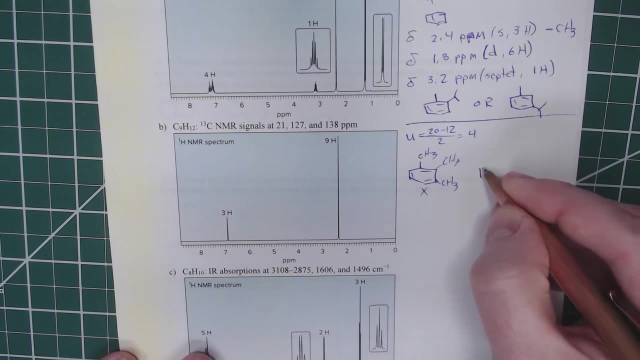 to that, but these hydrogens are not identical to this, So we wouldn't get a singlet, We'd get two singlets there. So this can't be it All right If we just start going around and looking at all the possibilities. 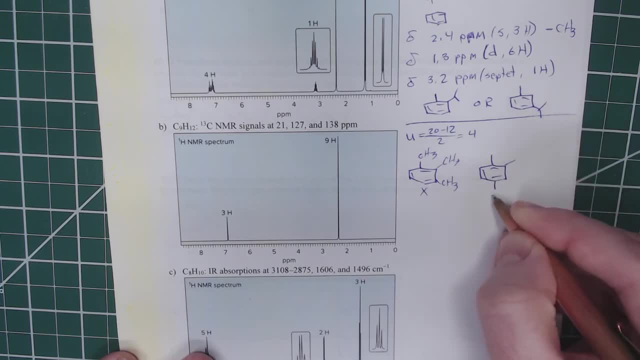 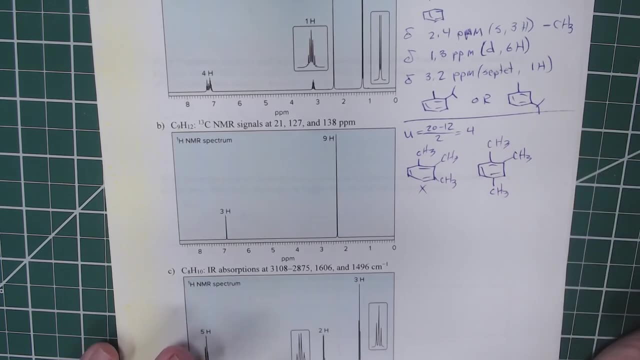 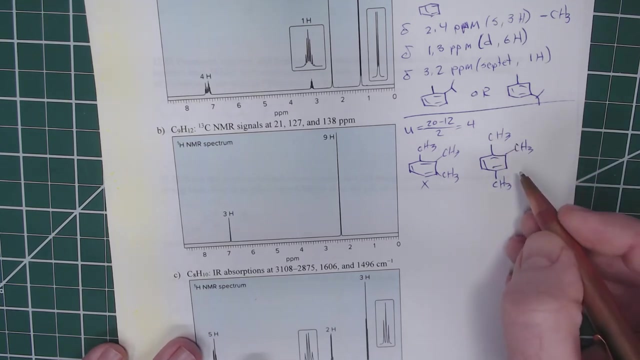 all right, one, two, uh, four. All right Again. CH3 is for all of those. Well, that also isn't going to work. Uh, and the reason that that isn't going to work is because, uh, all three of those methyls are different. Uh, we have these two that are adjacent to each other. 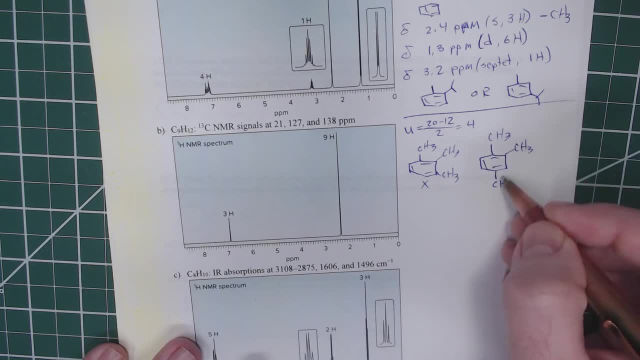 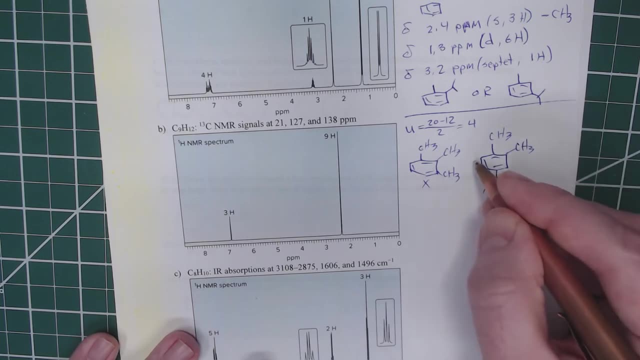 This one, that's para. to that one, It's met, it's ortho or meta to this one, It's. this one's not going to work, because that would give us three different uh methyl signals. In addition, these should not be singlets as well. And then, finally, we can look at another possibility, If we start. 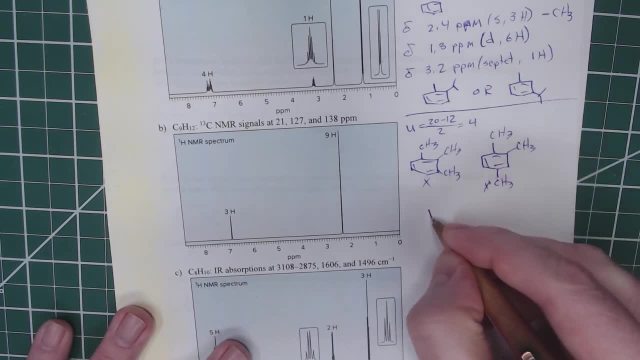 going around, we'll see that there are. there's limited number of possibilities. The only other one is going to be this: All right, here the three, the nine hydrogens that are in the methyls are going to be identical And, uh, the three hydrogens that are on the benzene. 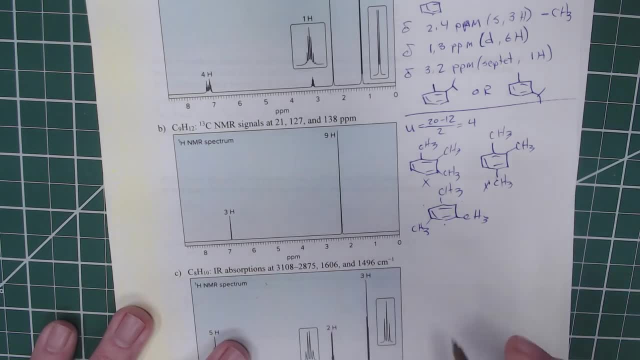 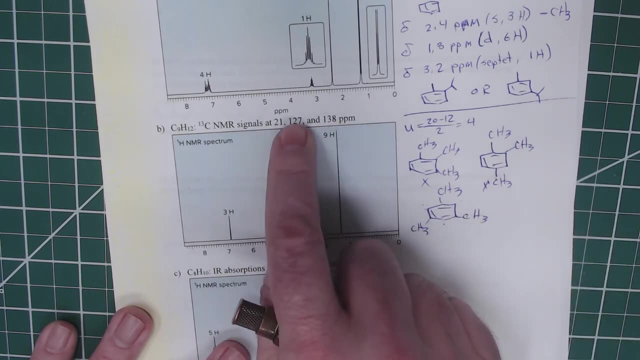 Are going to be identical And we only have three different types of carbons, Since these three carbons are identical. these three carbons are identical And these three carbons are identical. That would account for the three different types of carbons, And so this is our structure. 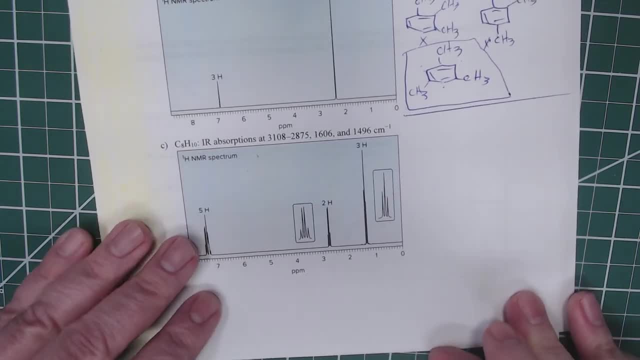 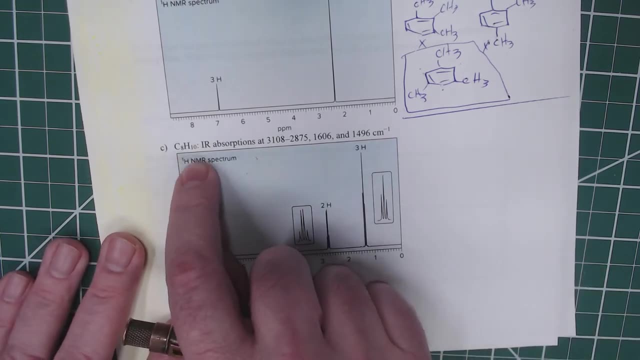 So that is our best structure for that data. All right, And then next we've got C8H10.. Uh, again we'll do the degree of unsaturation. Uh, when we calculate that degree of unsaturation eight times two is 16 plus two is 18,. 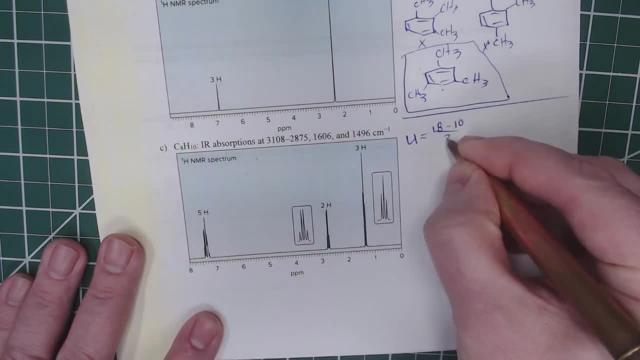 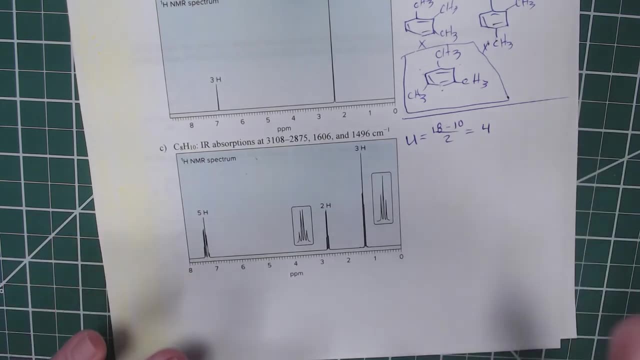 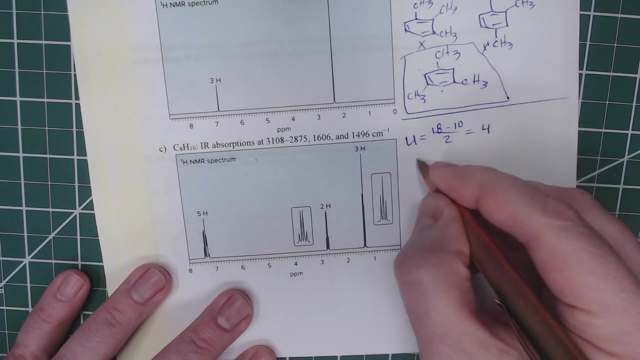 18 minus the actual 10 hydrogens divided by two, And that gives us four degrees of unsaturation. So we're not surprised by this. We've seen this a number of times. So we have a benzene ring And if we look here we've got the carbon, SP2 hydrogen and the carbon. 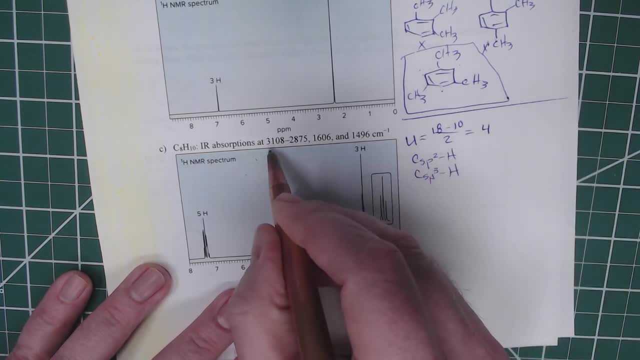 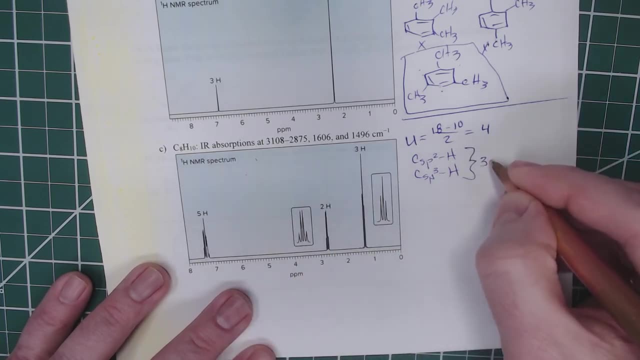 SP3. Hydrogen, All right. So because we have it on both sides of 3000, that's why we have both of those And I'm just going to put that together, So 3108 to the 2875. And because it goes on both. 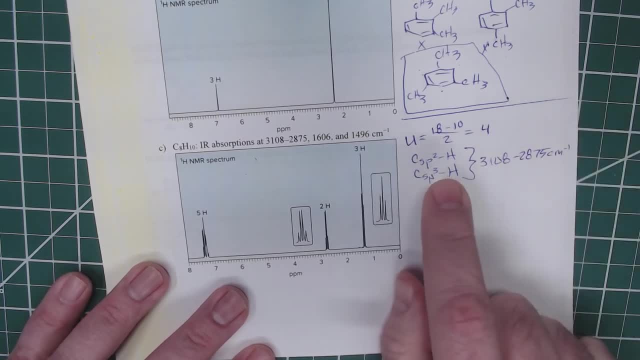 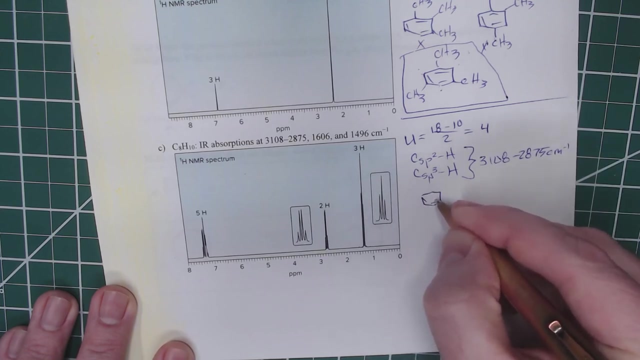 sides of 3000, we have both types of hydrogens. If we look, it's mono substituted, because we've got five high Oh, and here we have a benzene ring. So this is benzene, So we've got a benzene ring in there and that's the uh, the 1606 comma, 1496 reciprocal centimeters. 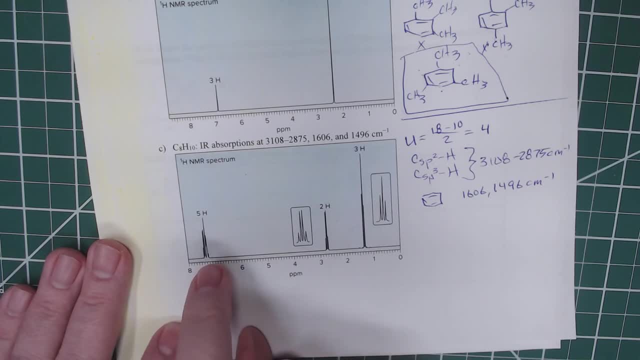 All right, So we have a benzene. and then, uh, when we look at this, we have a mono substituted benzene ring, because there are five hydrogens on the benzene ring. That means only one carbon has a substituent on it. All right, So six of the carbons are in the benzene ring We have. 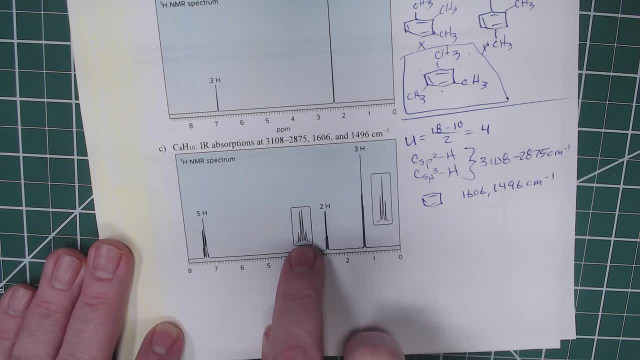 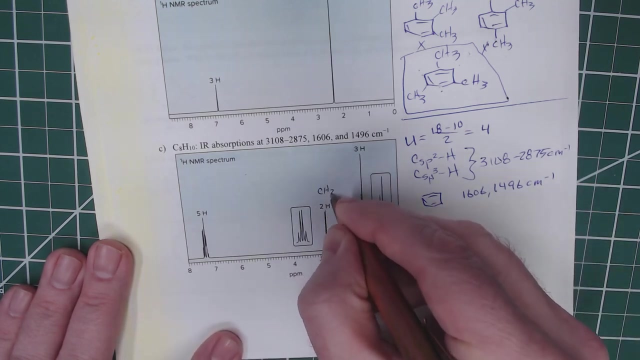 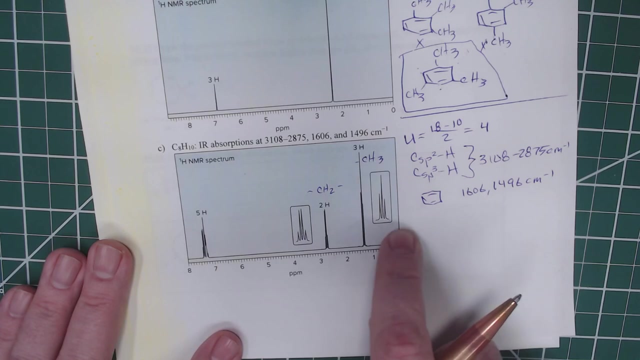 two that are not. if we look over here, we've got a quartet and a triplet, because these must be coupled to each other. and when we have a quartet and a triplet, that is a typical pattern of an ethyl. all right, where this is the ch2 and this is the ch3 and the ch3 is adjacent to that ch2. 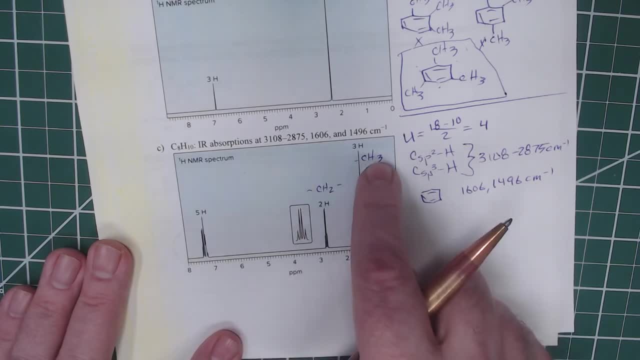 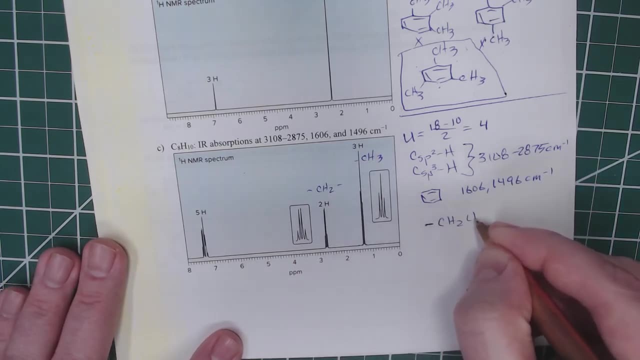 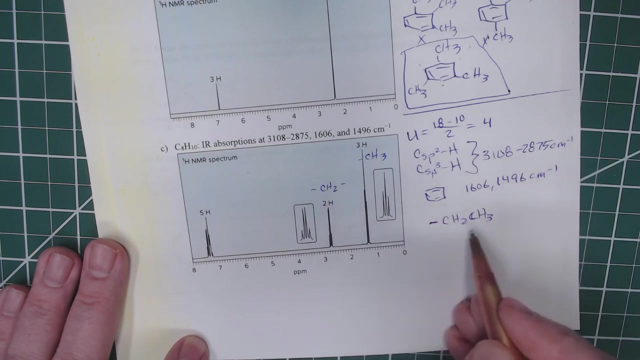 that's why this one is a triplet. the ch2 is adjacent to that ch3. that's why that one is a quartet. so that is a typical ethyl pattern: ch2, ch3, since we don't have any other atoms, and we've accounted for c6, h5 and then the other five hydrogens and other two carbons. here there's